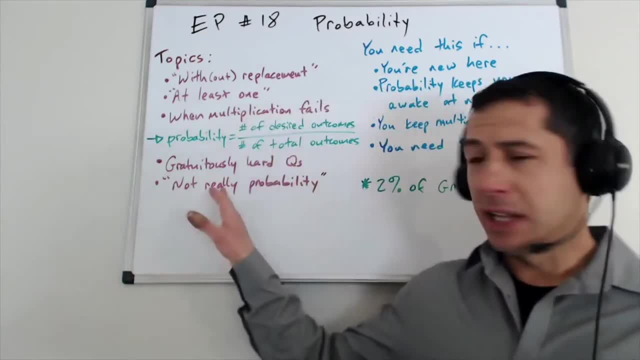 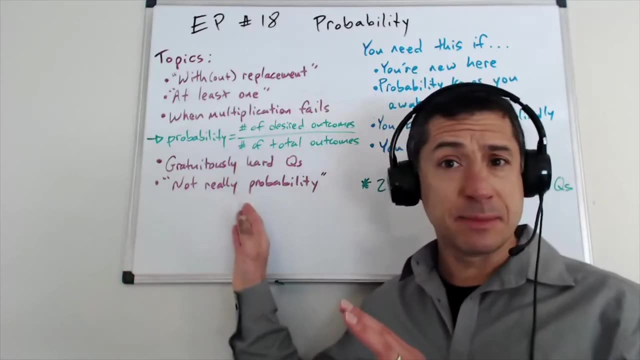 overlapping sets or combinations of permutations. So I'll give you a little sampling of a couple of those towards the end of the video, And I'm not trying to get through a ton of different topics and cram them all in here. I just want you to be aware that sometimes when you see the word 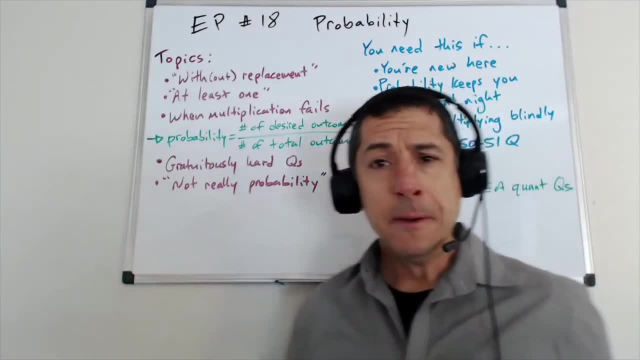 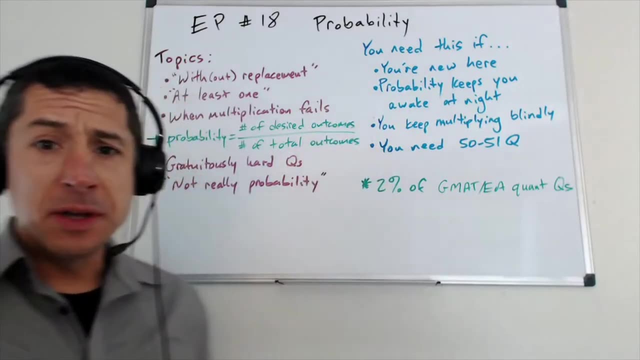 probability. there's nothing really technical going on with the probability itself. Now, who's this video for? Obviously, if you're totally new to studying probability, first third to a half of the video is going to be really valuable for you. More importantly really, who we're aiming this at is people who are just kept up at night about. 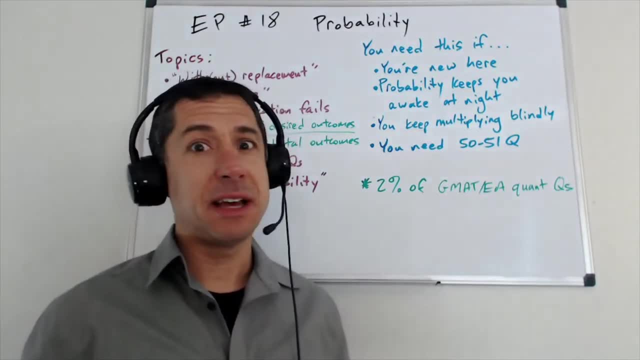 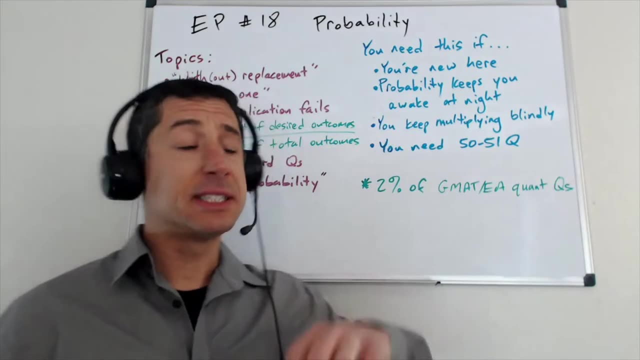 probability, or you walk out of your exam and you go: oh man, the probability. that was the thing that really got me Again. you probably aren't going to see a lot of it on your exam, but if it's really bugging you. number one, we're going to cover those foundations. Number two, I'm going 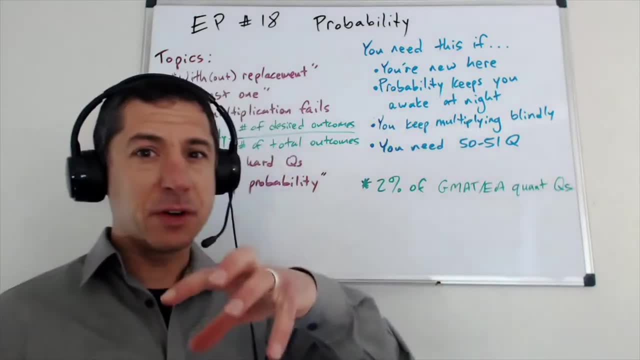 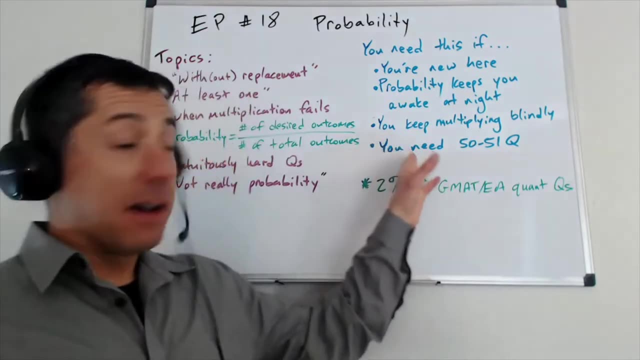 to be super clear about kind of where that line is between what you really need to know if you're going for a pretty good GMAT or EA score versus what you might want if you're going for a super, super high quant score. Obviously, if you are going for that super high quant score, 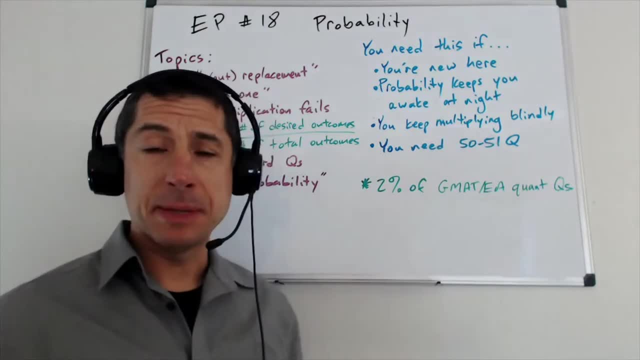 pretty much everything we're going to do today is going to be at least of some value. maybe the first few will be a little bit easy. Feel free to hit that fast forward button if you're a high flyer and skip ahead to some of the tougher ones towards the end And again. 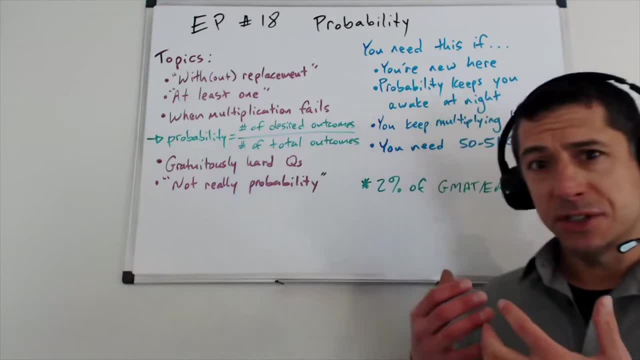 one of the things we're going to emphasize is if what happens to you when you do probability questions is you find you're just multiplying things blindly. you're just multiplying fractions, not sure why, not sure what it's doing, get a lot of wrong answers or at least inefficient. 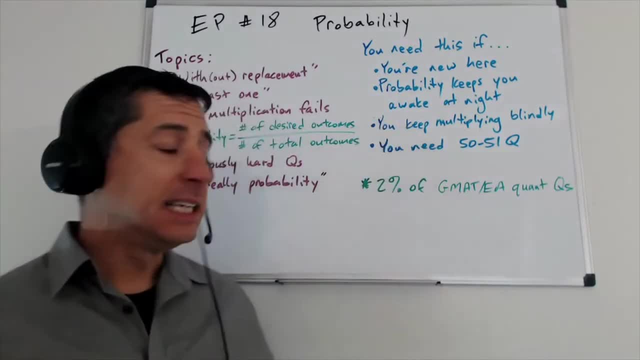 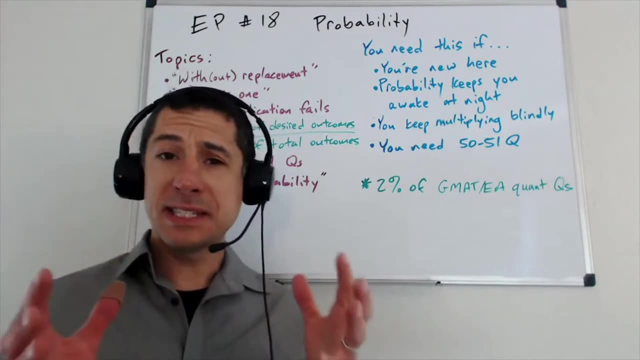 solutions. We're going to address that in quite a few of the questions today And again can't emphasize this enough. only about 2% of your GMAT and EA questions on the quant are going to be a probability, So this isn't something that's worth losing a ton of sleep. 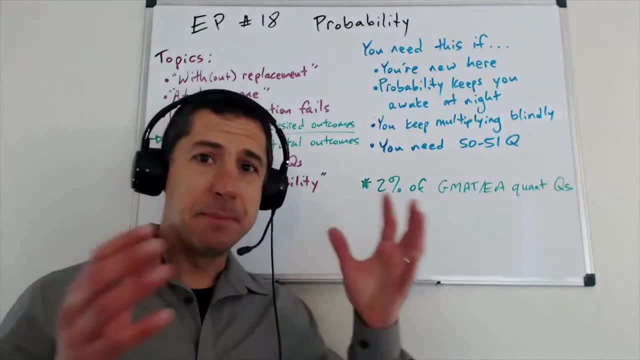 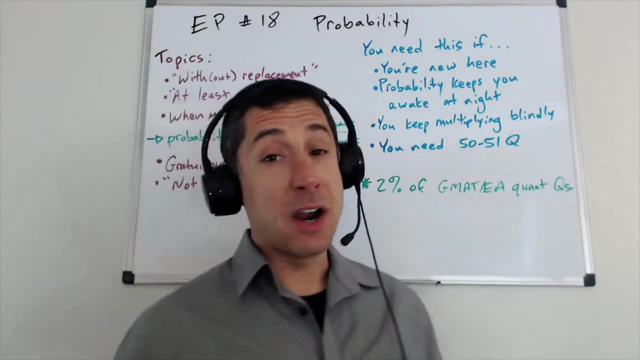 over Again. if you're going for something like a mid 40s or below score on the GMAT, first half is going to be great for you. Last half of the video is going to be more for those of you who are high flyers. All right with that. we'll warm you up with our first question. 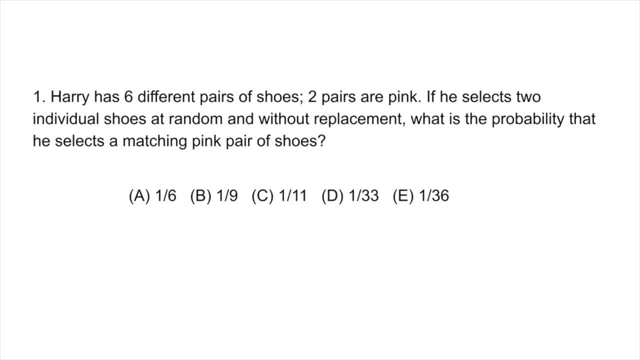 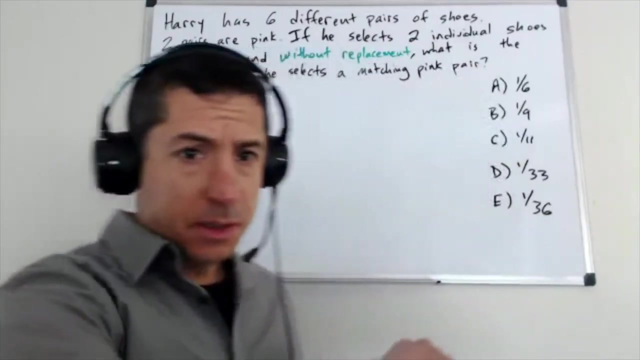 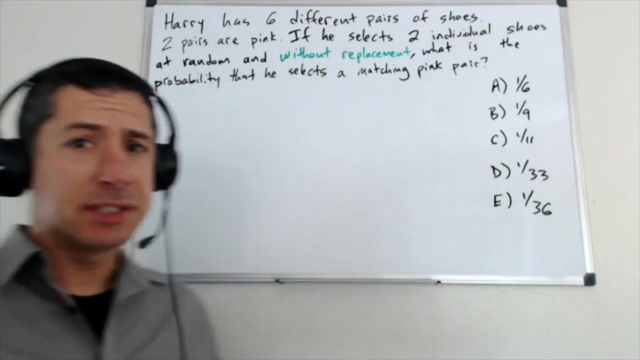 All right, let's get started, As always. if you need a little bit more time, feel free to hit that pause button. All right, nice little warm up question here with a bunch of different components, just trying to pull apart that word soup you sometimes see in probability questions, but nothing super. technical here at all Got to go. I'm going to be right back in a minute. Let's get started. All right, so here we go. All right, so let's get started. All right, so let's get started. 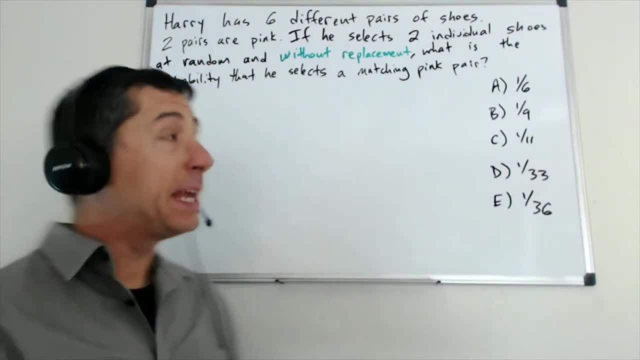 Let's get started, All right, so let's get started. All right, so let's get started. All right, let's get started. All right, let's get started. All right, let's get started. guy named Harry, six different pairs of shoes. two of those pairs are pink, and he's going to 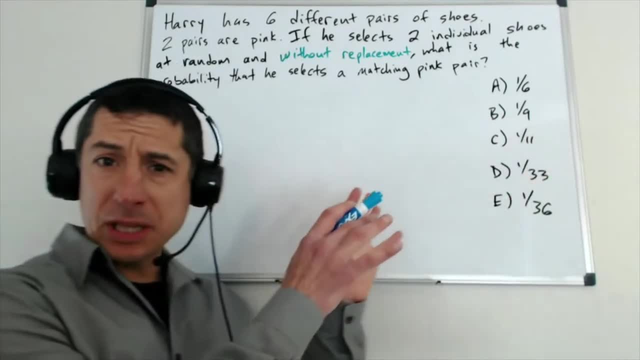 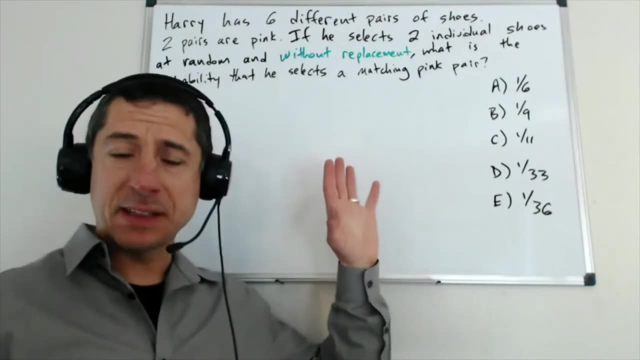 select two individual shoes at random. I'm not trying to be tricky here with the language. GMAT really is never out to be tricky with language. It's one of the things we kind of tell ourselves and it just makes our lives harder. They're really, really specific. They're usually phrased. 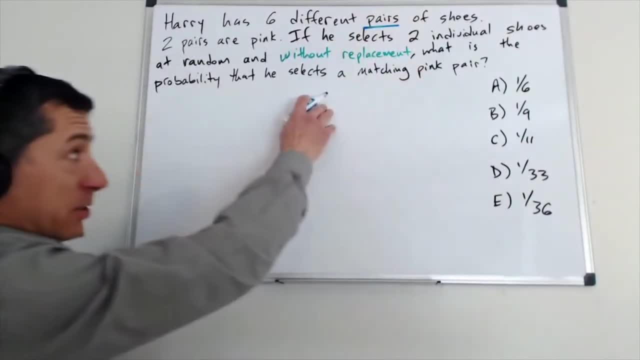 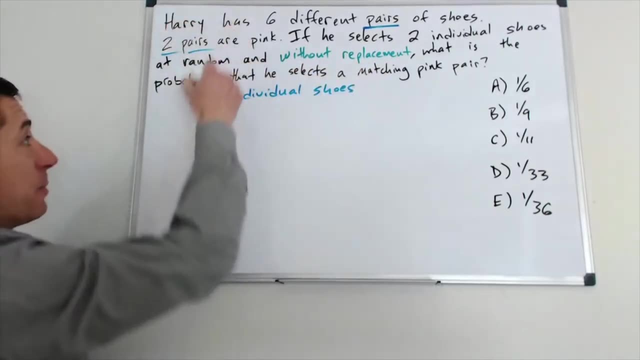 super, super carefully, Talking about six pairs of shoes. He has a total of 12 individual shoes in his closet And two pairs are pink, So four pink shoes And we're selecting two individual shoes at random, without replacement, And we want to know what's the probability, not just that he. 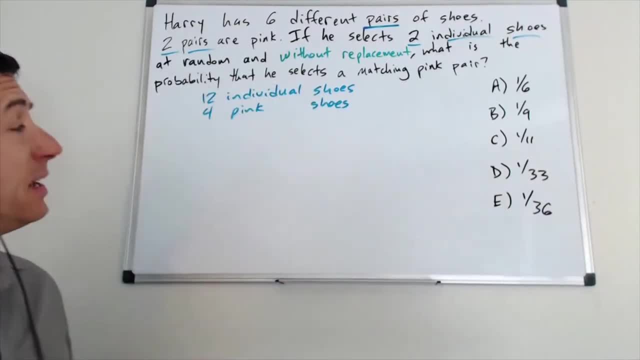 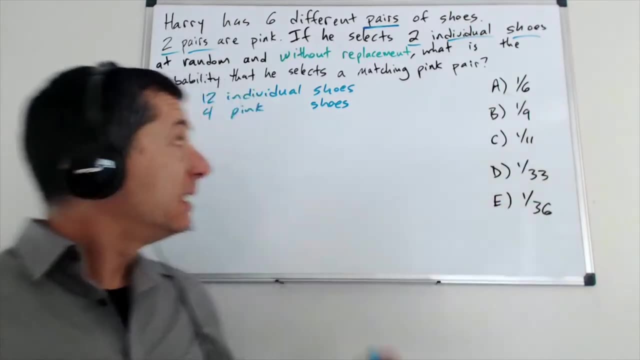 selects two pink shoes, but that he selects a matching pink pair of those shoes. All right, So fairly straightforward. in one sense, you're only reaching in. let's say that all of these shoes are just laying on the ground in the closet, reaching in twice, picking a shoe first time. 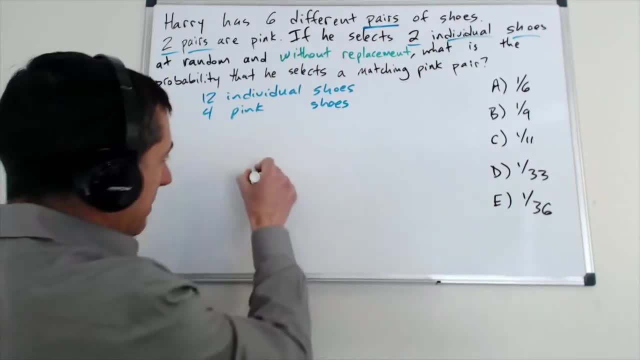 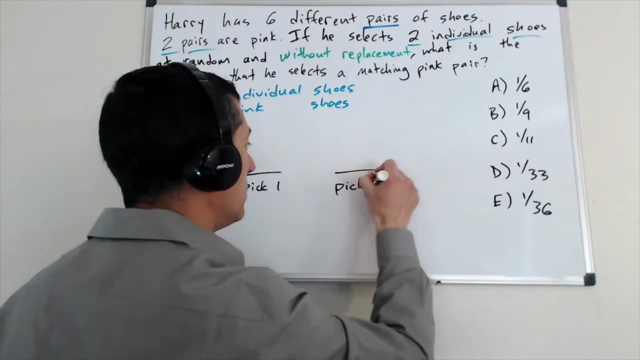 and then reaching in and picking another one. So we can kind of set it up as a fairly straightforward little probability problem. on pick one, We're going to have some probability that he gets what he wants. Pick two: some probability that he gets what he wants. We can multiply those two things together and get our 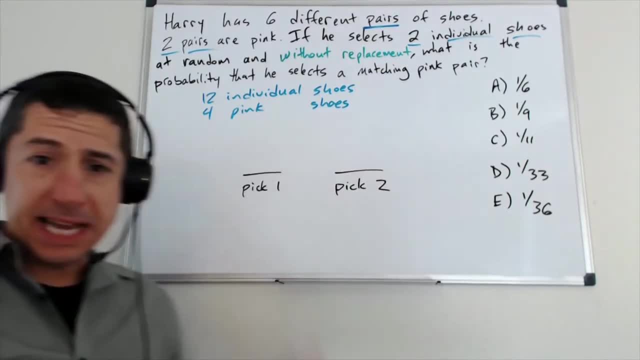 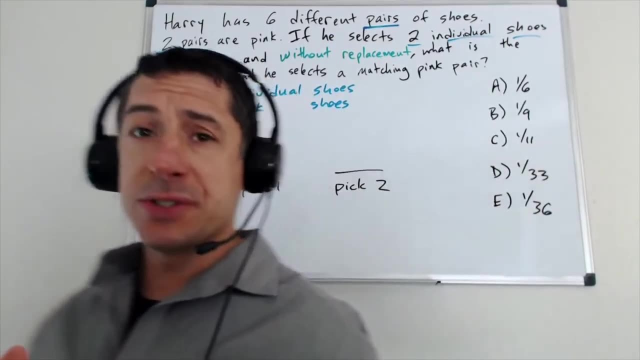 answer: Okay. So on the first pick, what's the probability that Harry ends up happy and gets a pink shoe or get something that would set him up to get a matching pink pair of shoes? Obviously, he just needs to get any pink shoe on this first one He's going to be a happy guy. So four pink. 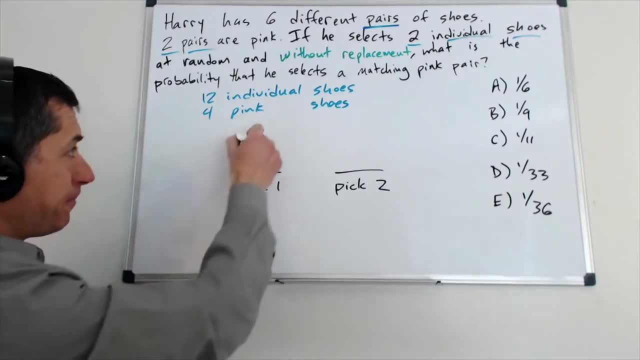 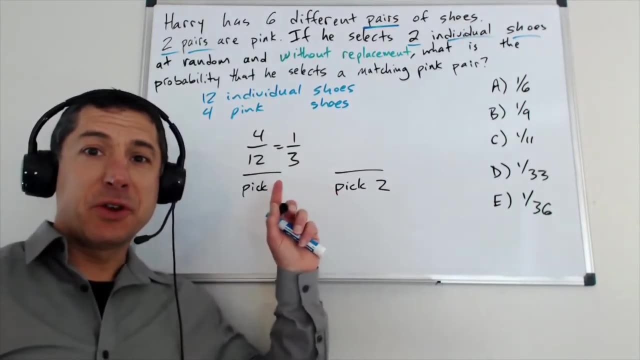 shoes out of 12.. That's the probability that he gets a matching pink pair of shoes. That's the fairly straightforward part here. Call that one third, if you prefer. Now pick two is where it gets interesting. So if you're not paying attention you might say: well, this is also four. 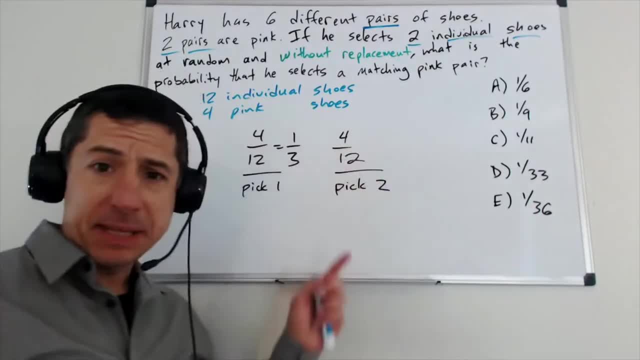 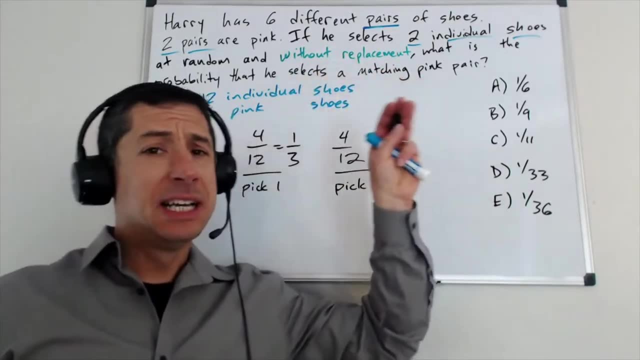 out of 12, or one third. Well, why would that be the case? Well, it'd be the case if you're putting the shoe back in. That's where this language around, with and without replacement, really matters. Again, nothing super fancy there, but we find out of our students, is they sometimes just? 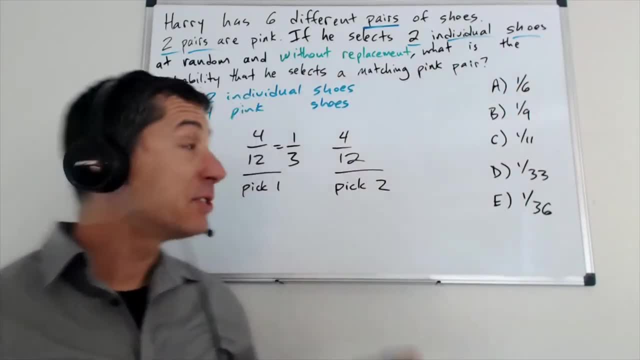 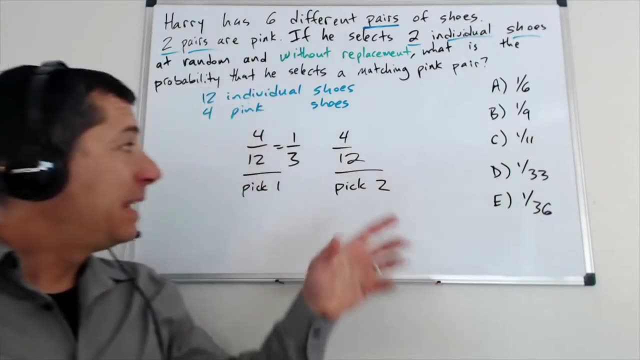 blast right through that kind of language and don't think about whether the shoe's getting replaced or not. Here it's not getting replaced. So what's Harry doing? He reaches in, grabs a shoe, tosses it behind him. Now, what's left in? there isn't 12 shoes, four of which are pink. What's? 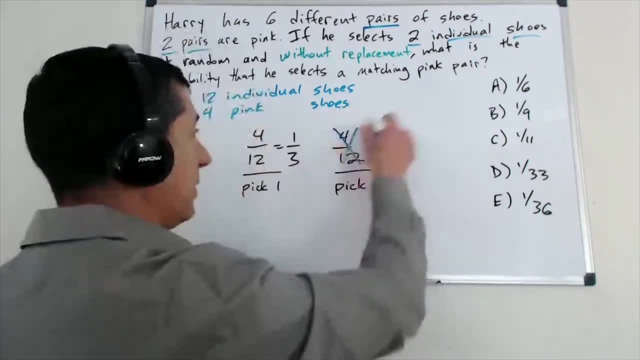 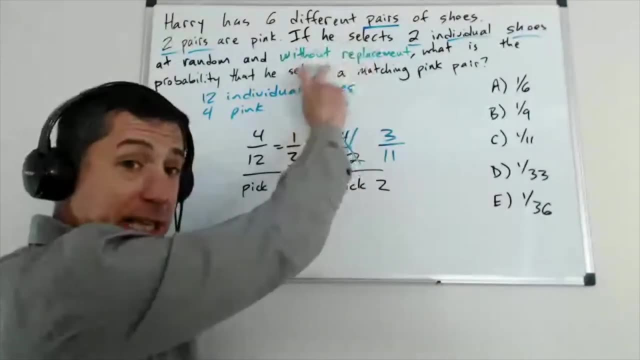 left in his closet are three shoes that are pink and 11 total. So again, nothing technical, Just a reminder: make sure you're paying really close attention to that language, And if it isn't obvious from the language it's going to, it'll be obvious in some way, right, Even if they don't. 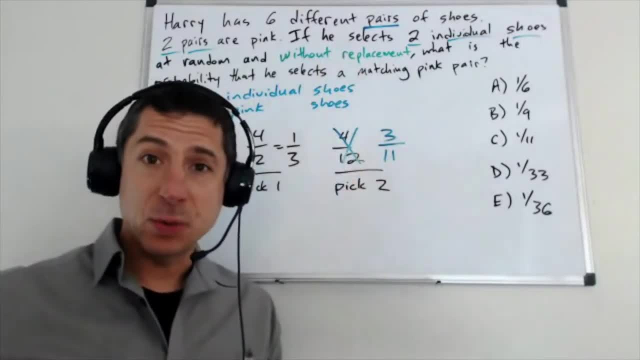 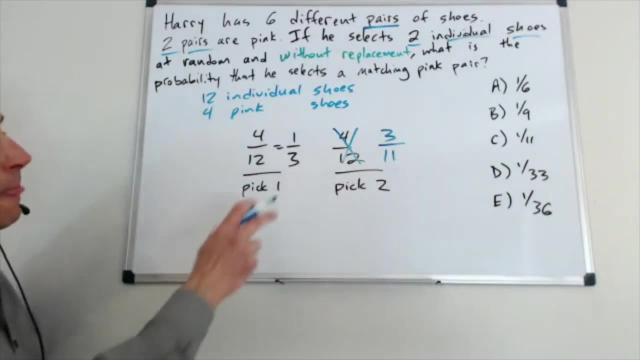 use that exact phrasing. it's just a question of making sure you give yourself that extra 20 seconds. take a breath and make sure that you're thinking through whether this number should be lower on the second pick than on the first. Okay, Now, this still isn't the right answer. Why? 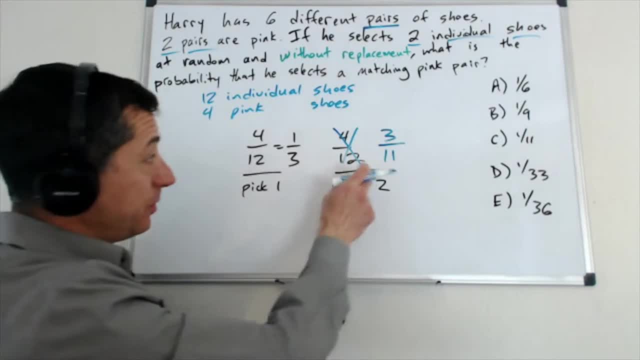 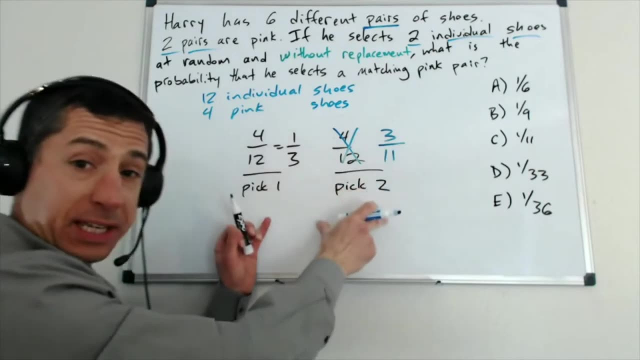 not. So 4 out of 12 is a probability of getting a pink shoe on that first pick. Three out of 11 on the second pick getting a pink shoe. But that's not what the question's asking us for. This would: 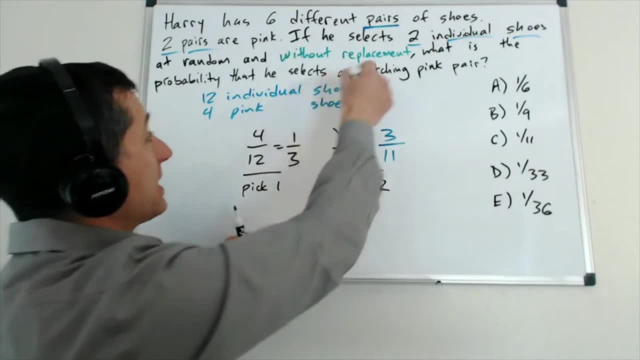 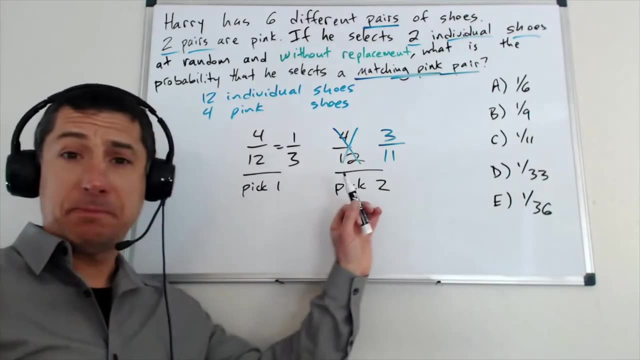 give you the probability of getting two pink shoes. What we want is a matching pair of pink shoes, So you're not going to wear your pink Uggs with your pink sandals, presumably, which is what you could well get when you set it up this. 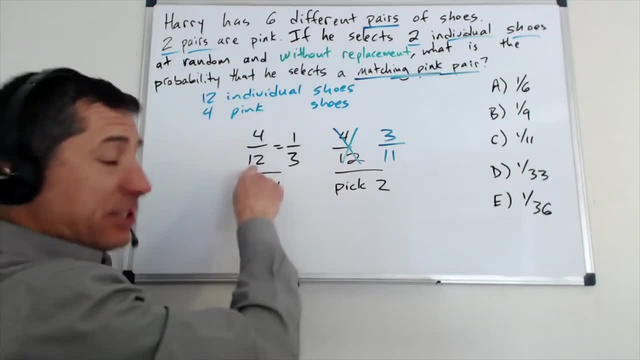 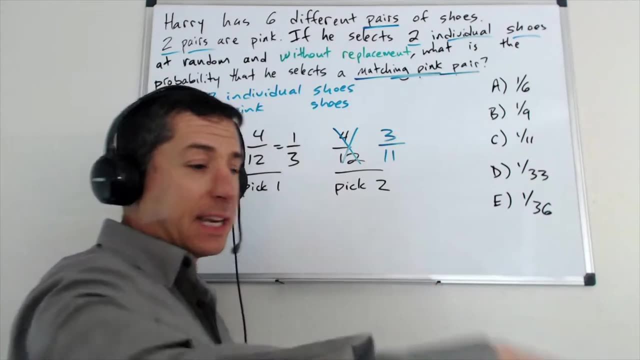 way And instead what we want is the match to this first shoe. So 4 out of 12 probability that you get a pink shoe on the first pick. Now there's only one shoe in there that's going to be its match. So, instead of three out of 11, the probability that you get its match is one out of. 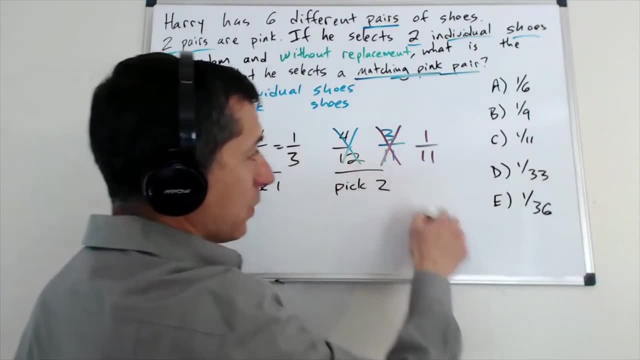 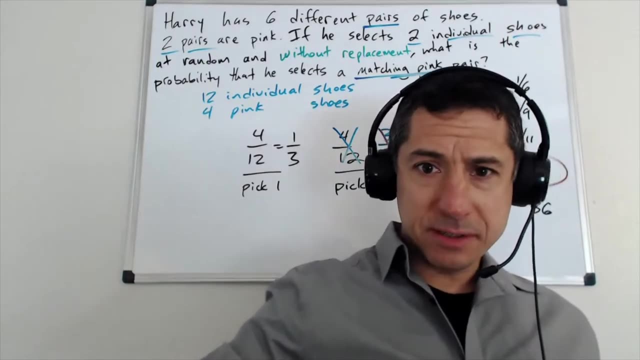 the 11 shoes that remain. Multiply these together one third times one 11th, and we get one 33rd in our answer. All right, Let's give you one more warm-up question, Not necessarily any harder than this last one. 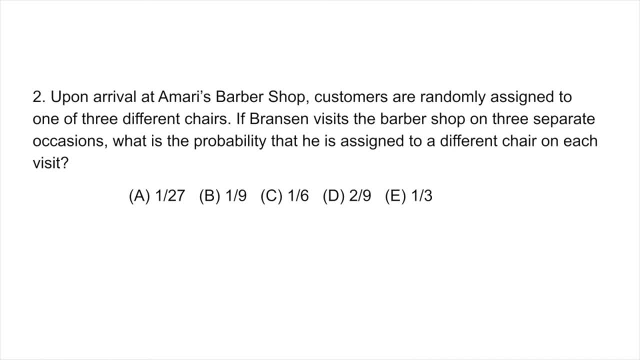 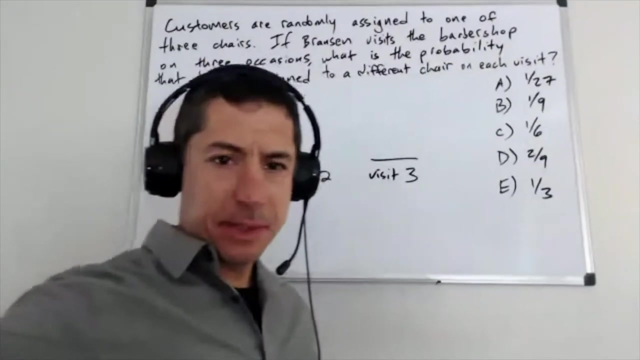 Let's give you one more warm-up question. Let's give you one more warm-up question. Hit the pause button if you need a little bit more time. Hit the pause button if you need a little bit more time. Okay, Nothing more technical here at all. Really just kind of the same foundations we talked about. 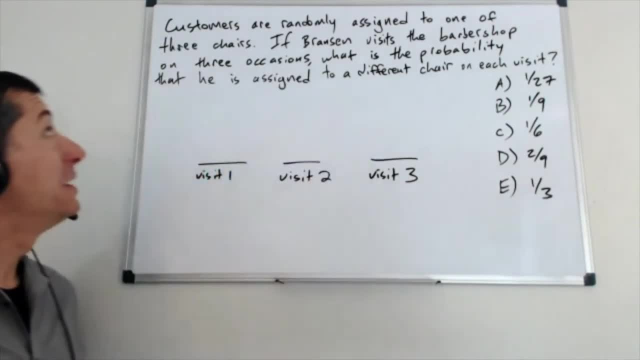 in the first question, just packaged in a slightly different way as the GMAT and EA like to do So. at a certain barbershop, customers are assigned randomly to one of three chairs. We've got a guy who visits the barbershop on three occasions. We want to know who's going to get the match. 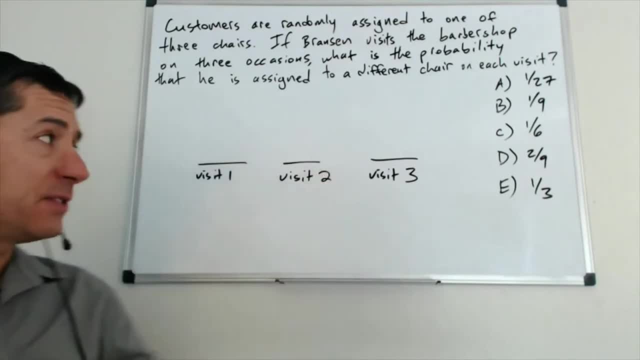 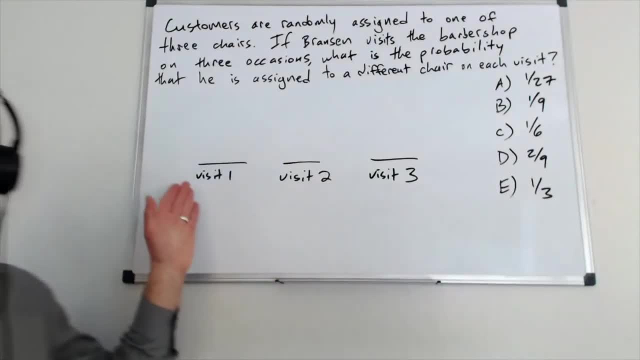 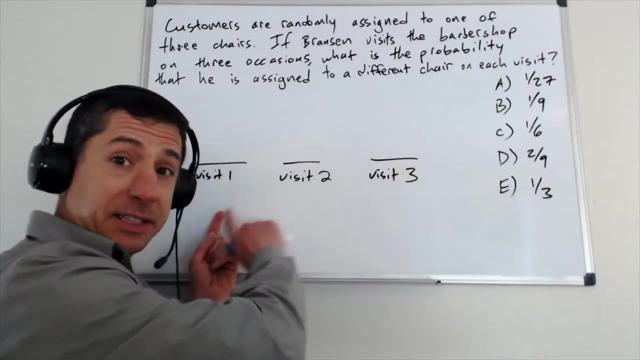 So we can just go through each of these three visits- Nothing super fancy going on- and say, well, what's the probability that he's going to do something on the first visit? but on that first visit he's assigned to a chair that gives him the opportunity to be assigned to a different. 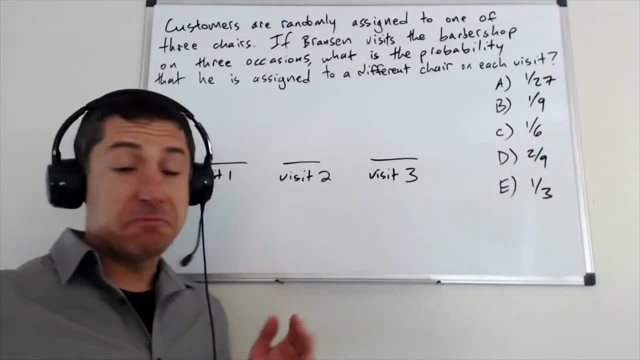 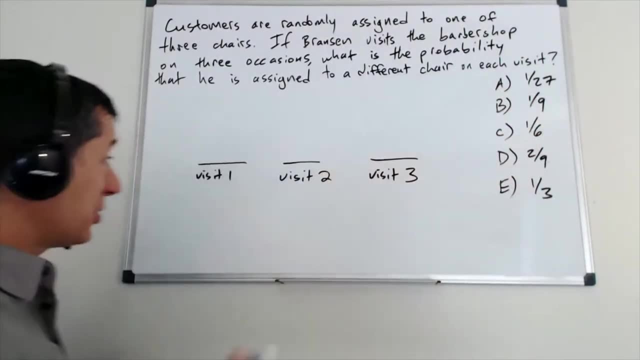 chair in all three visits. So in the first visit what has to happen? It doesn't matter. He has to be assigned to a chair. It doesn't matter which one he's assigned to, as long as the next ones don't match. 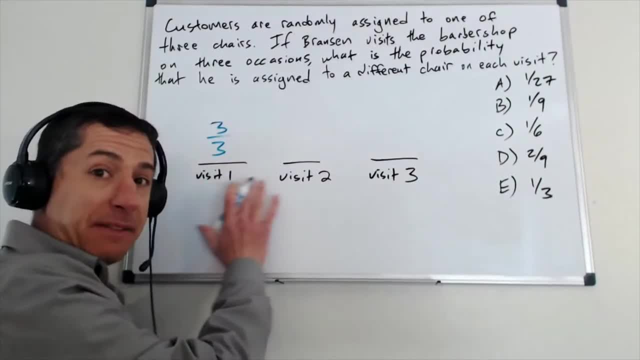 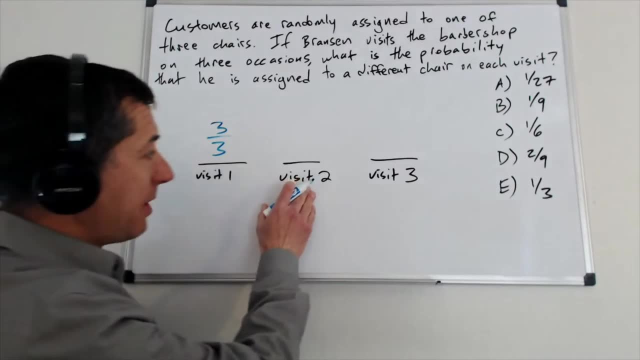 So your probability that he's going to be set up up to have a different chair on all three visits, The probability that happens on the first visit that he's set up for that is just three out of three, or one. What about visit number two? Now? 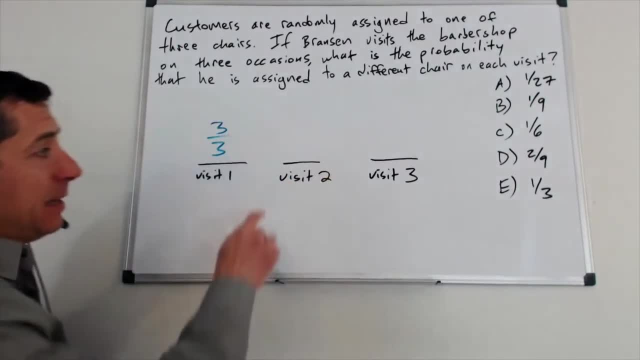 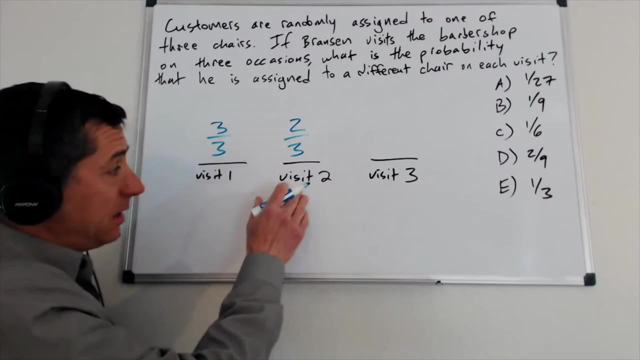 you just have two chairs that are left that Branson hasn't sat in yet, but you're still picking out of those three chairs in that random assignment. So your probability is two out of three on the second visit And on visit number three, what has to happen in order for Branson? 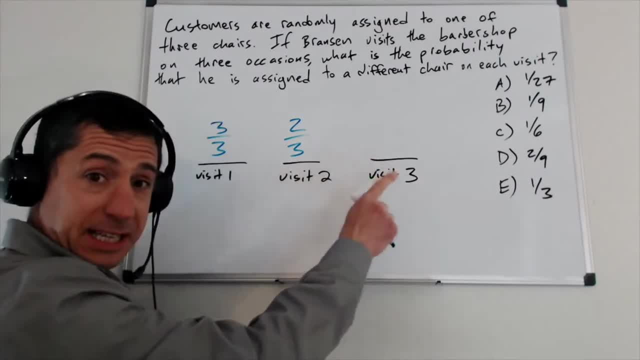 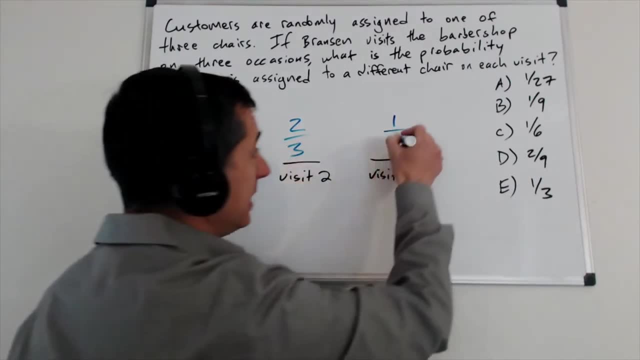 to get a different chair on each visit. Well, he still has to be assigned to that third chair that he hasn't been assigned to yet. So there's only one chair. that's going to work out for him. if he wants a different chair on each visit- And there's still three to choose from- Multiply these guys. 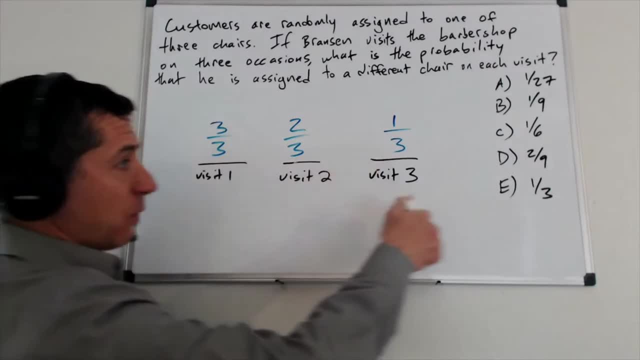 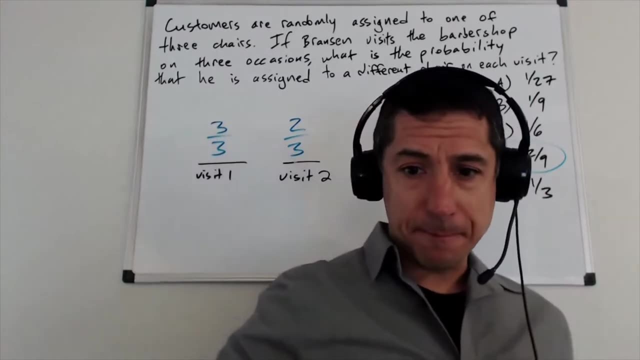 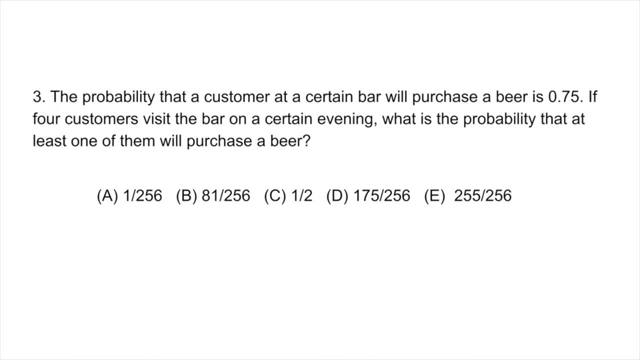 together. So this is just one. two thirds times one third just gives you two over nine, And that's it All right, One more warmup level question, then we'll start ramping this up a little bit. Thank you. 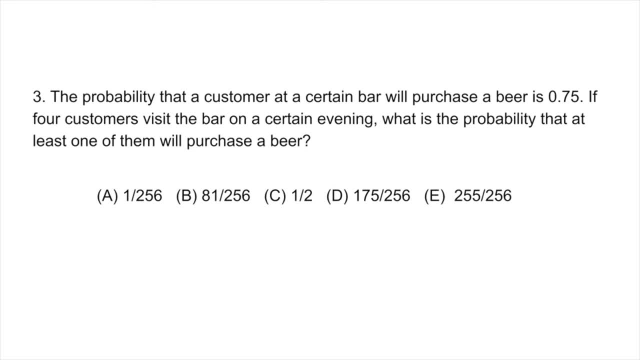 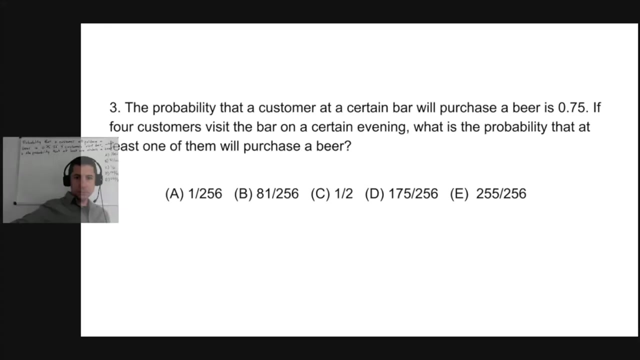 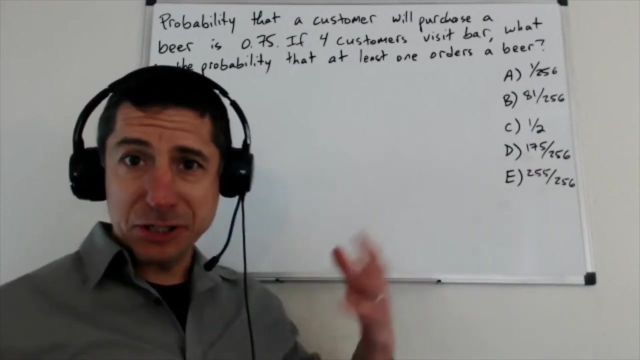 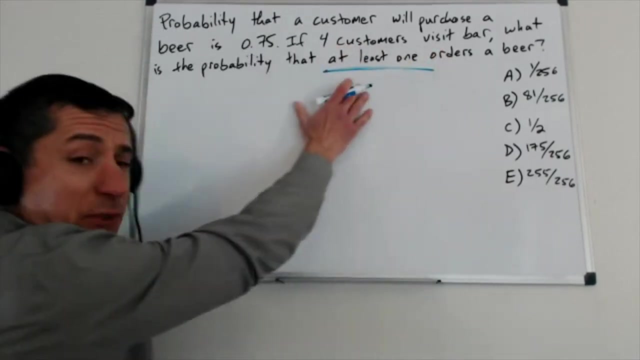 you as always. if you need a little bit more time, feel free to hit the pause button. okay, this is kind of the last of our relatively foundational probability questions. after this will start getting a little bit funkier and pretty gratuitously hard towards the end. that's what kind of centers on this phrase, at least one and to whatever extent you see. 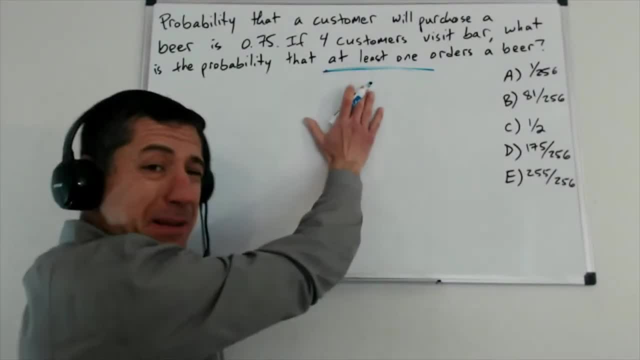 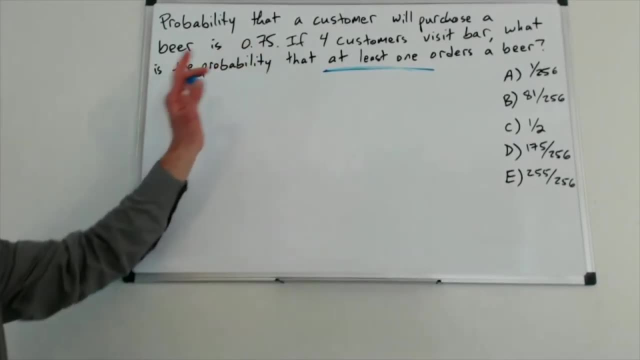 probability questions on the gmat. again, just two percent of the quant questions. this might be the single most frequently tested concept is: can you look at that and think of the most efficient way to solve it? now i see a lot of goofy stuff on this. so this particular question. we've got four. 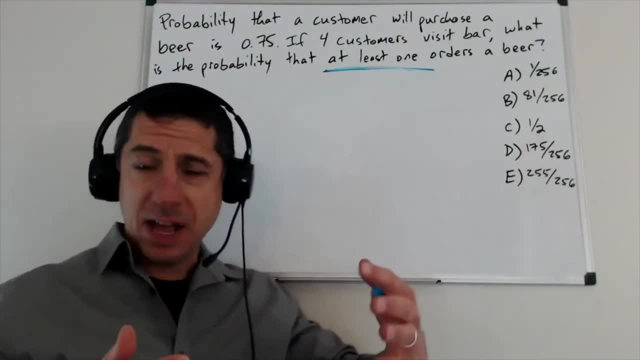 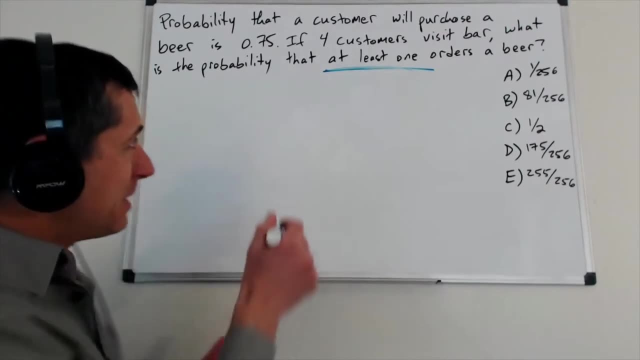 different customers entering a bar. each one has a probability of 0.75 or three quarters of the order of beer. we want to know what's the probability that at least one of these customers orders a beer. i sometimes see people just kind of start blindly multiplying here and again. that's. 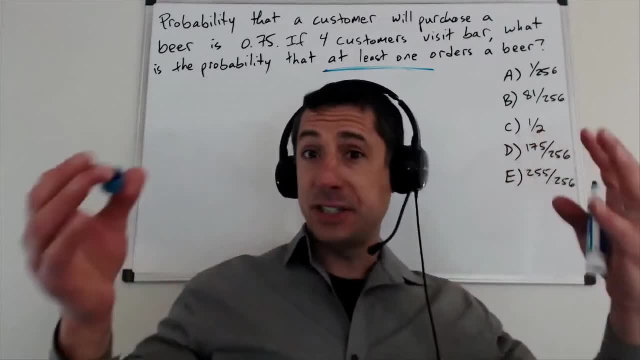 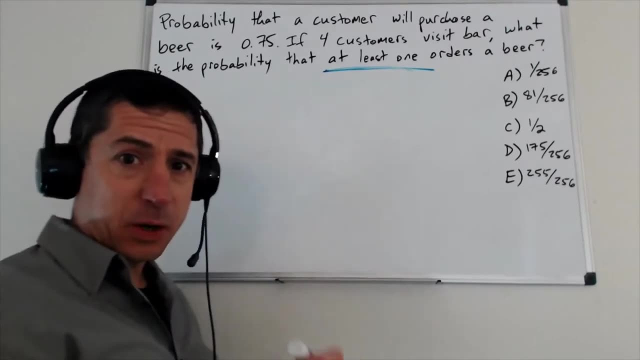 probably the single most common error, just in general on probability is that we think of it as just hey, i multiply a bunch of fractions together to get the answer and it doesn't take a whole lot to make the question just funky enough that that's not going to work for you. 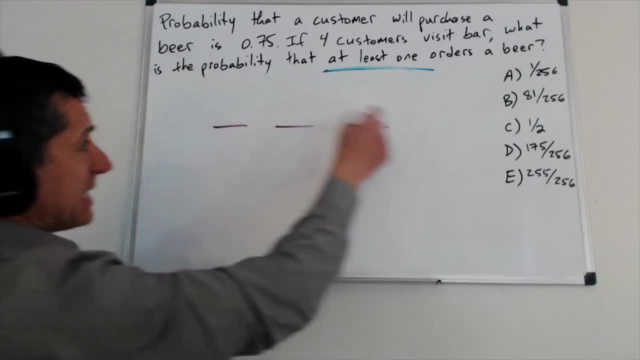 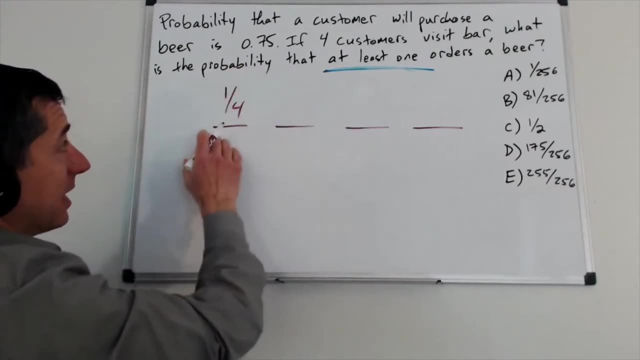 so here kind of mistake i see fairly often is they'll say, well, number one they might misread, this is just one. so they'll say, well, hey, the, the, i need the first one to be a customer that orders a beer, and then the rest will be customers. 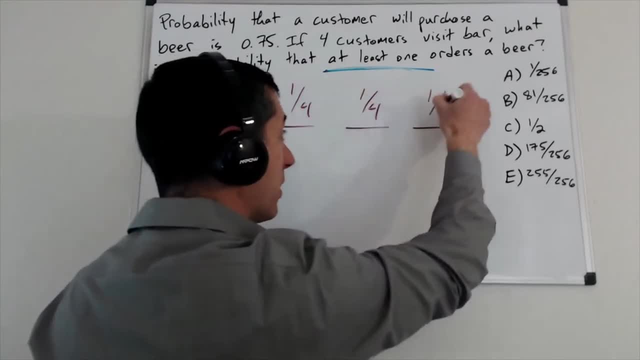 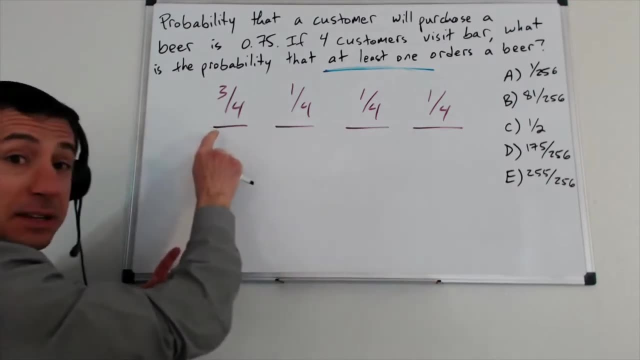 who do not, and this is nowhere close for a whole lot of reasons. number one is that this is the probability of getting exactly one beer, and not just exactly one one beer, but the first customer orders a beer and the rest don't, and then we get into this whole bloodbath. you could try to start. 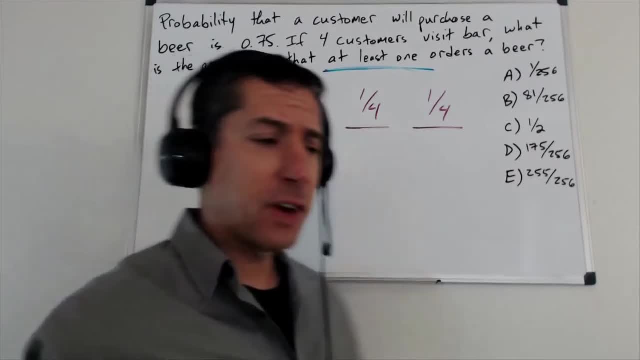 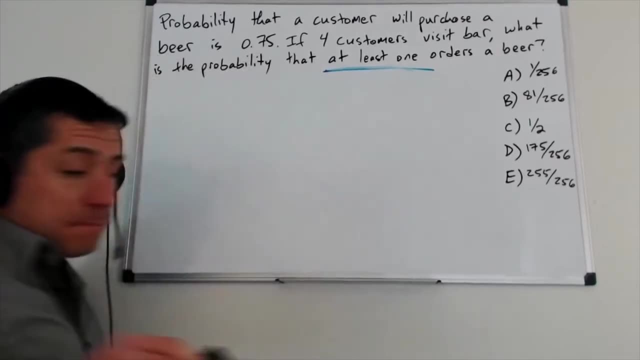 kind of taking this and going: well, what if it's the second customer in the third, and then you're going to be here for a very, very long time and there was still obviously that misread embedded in here. so okay, so that doesn't work. i see that mistake fairly often, probably equally as common. 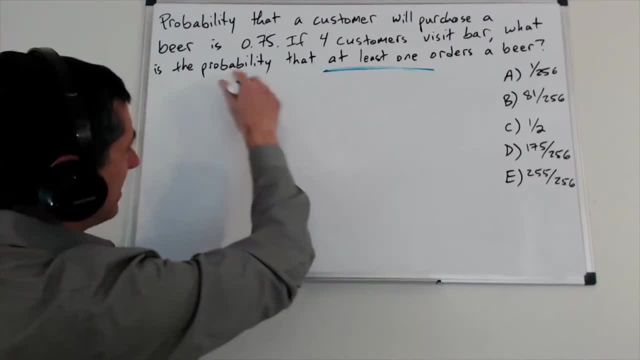 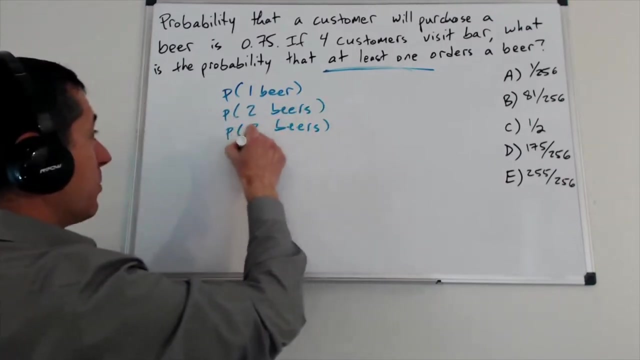 i'll see students who are kind of this for the first time say: well, what does this mean? so the probability of getting at least one, so i can calculate the probability of getting exactly one customer ordering a beer. so two customers order beers, probably that three customers order beers and the probability that four customer order beers, and i calculate each. 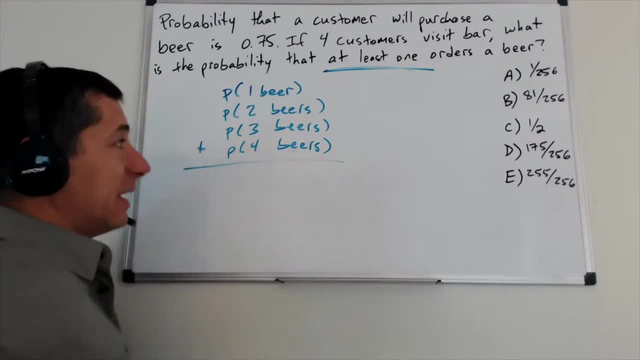 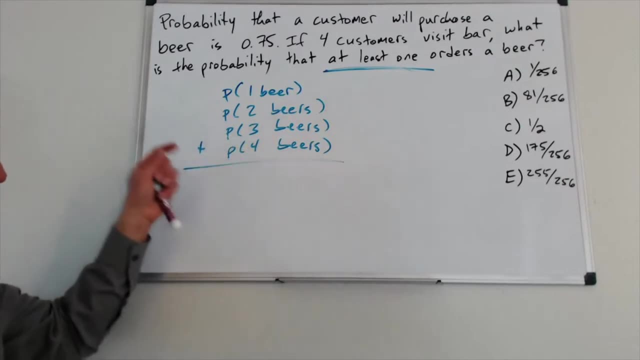 of these probabilities individually and i add all of them up and i get my answer. and that's pretty brutal too, because, number one, these aren't so easy to calculate. we'll talk about a little bit more later in the video. and also you've got to calculate the probability of getting at least one customer. 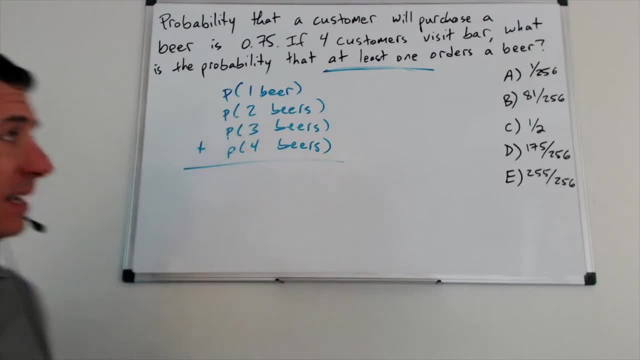 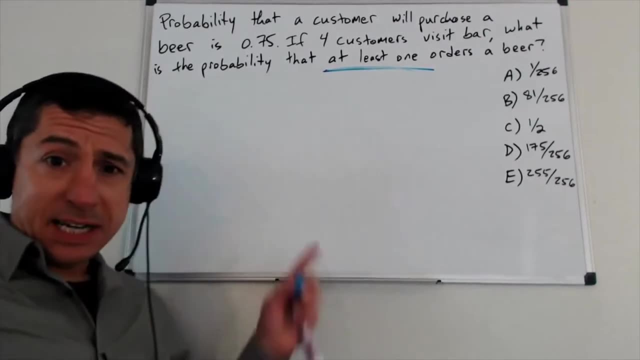 four different probabilities and then add them up and it's a ton of work. It's a big mess. So those are sort of the obvious ways that people tend to make mistakes on this. What can you do instead? It's really just recognizing a little bit of logic and credit. 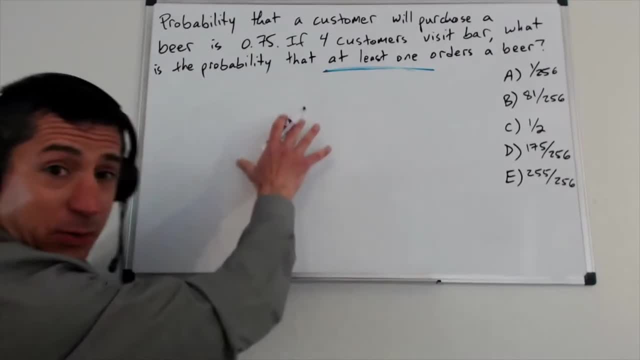 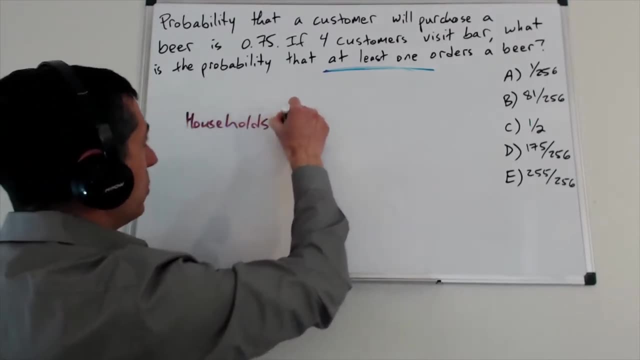 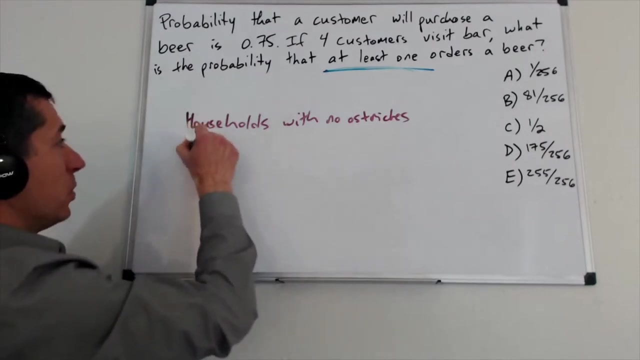 to a TA I had way back in undergrad who explained this kind of question this way. He said: well, there's two kinds of people in the world. There are households. we'll say two kinds of households in the world: households with no ostriches, And we have households. 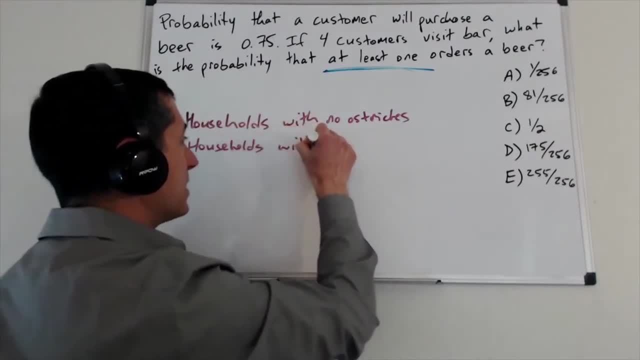 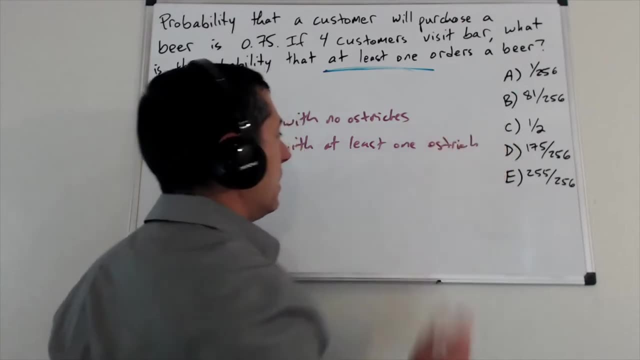 with at least one ostrich And it's like: why is this weird? I'm talking about ostriches. Well, it was a memorable way. It stuck with me 15,, 20 years later. I've kind of explained the. 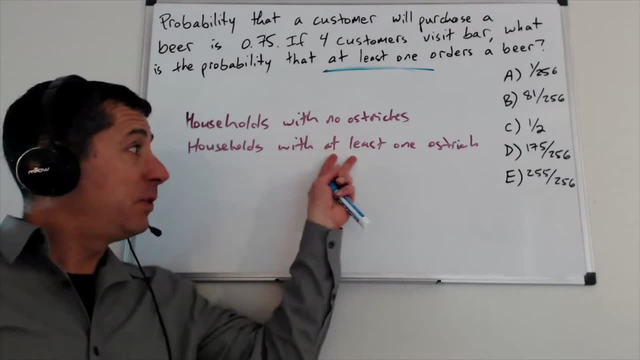 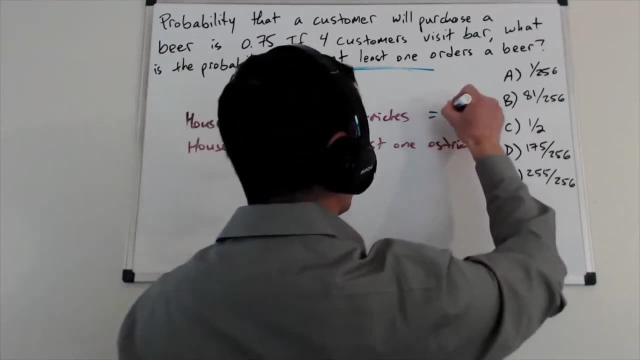 idea that everything in a situation like this, if you have that phrase, at least one, the compliment of it is having none of that thing. So, for example, if we know that 90% of American households have no ostriches, then we know. 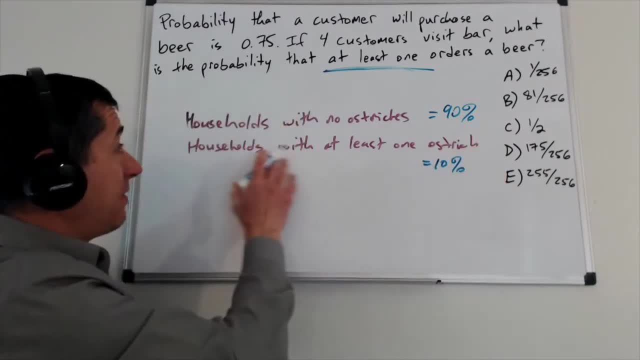 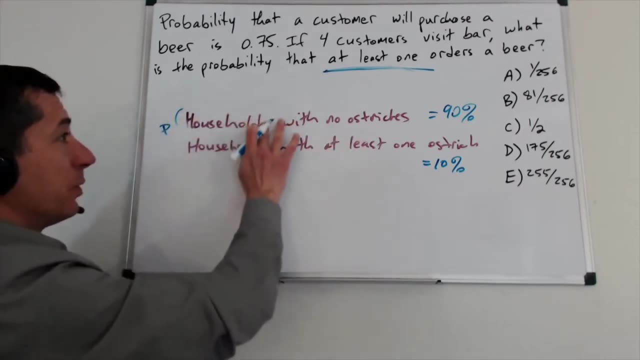 10% have at least one ostrich. Okay, fine, Now we could also express this as probabilities and say you randomly select an American household. What's the probability that you select a household with no ostrich? And instead of 90%, it's 0.9.. So then, what's the probability? 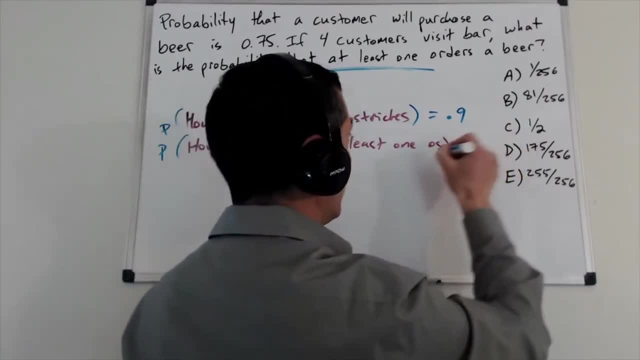 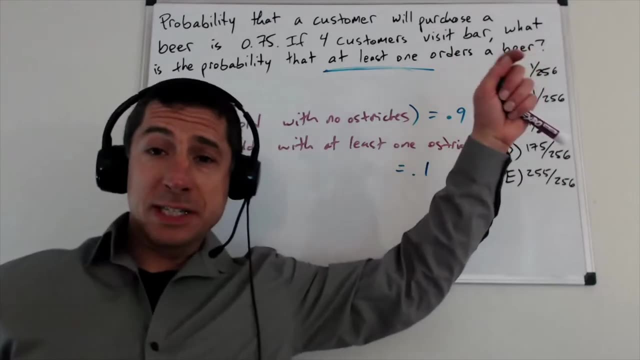 that you select a household with at least one ostrich. Well, same idea, It's got to be the compliment of that. So now you can apply that here and just say: well, what's the probability that at least one of these four customers order a beer? It's the compliment of that. So now you can. 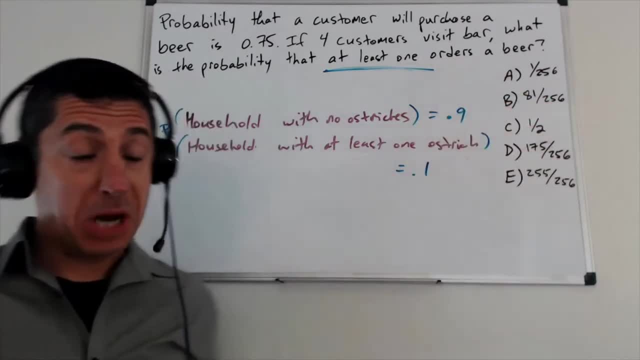 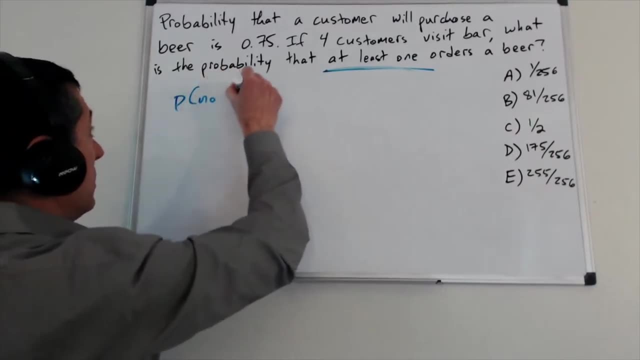 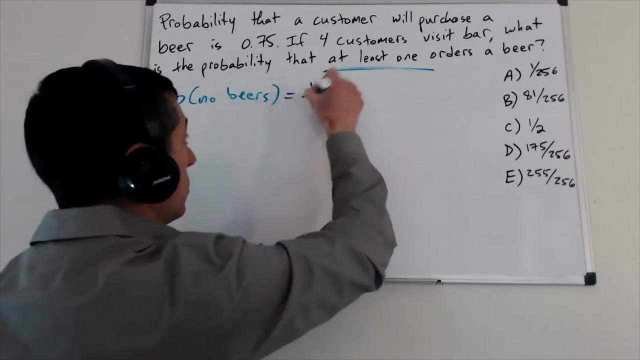 say: well, what's the compliment of no customers ordering a beer? Okay, And that doesn't sound so hard, What's the probability that no customers order beers? Well, probability is three-fourths that they do order a beer. That means one-fourth that they don't, So one-fourth times one-fourth. 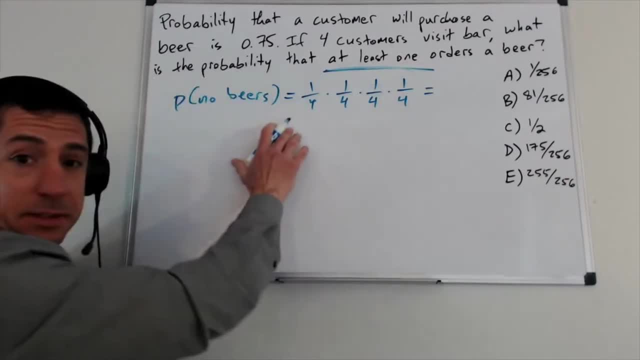 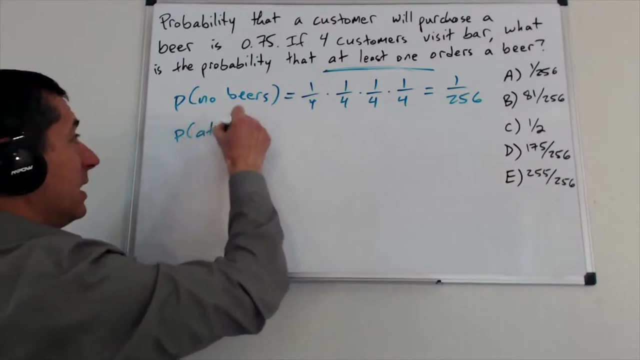 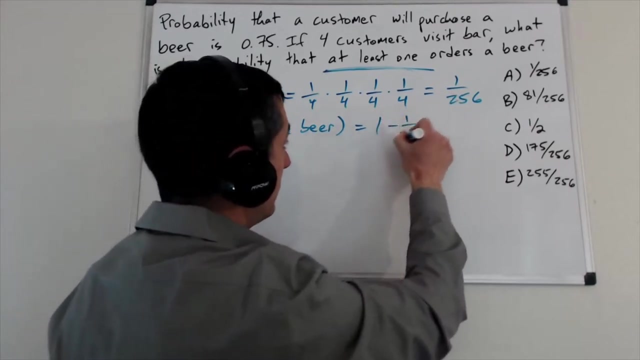 times one-fourth times one-fourth, So four to the fourth, So 16 times 16, one over 256.. That means that at least one orders a beer has to be one minus 126 or one minus one over 256.. 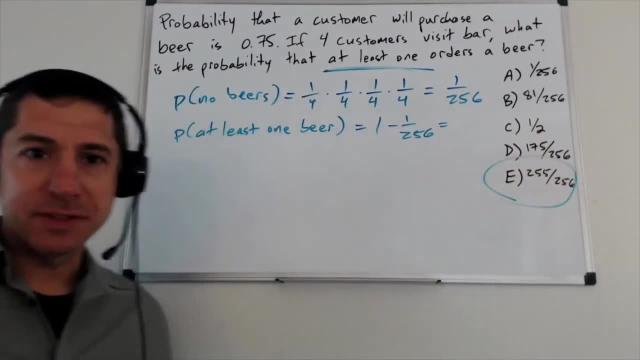 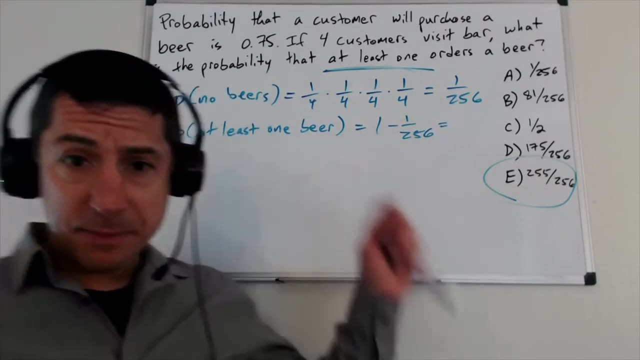 And that gives us answer: choice E: 255 over 256.. And that's all there is to it. Just want to make sure you hit the point where, whenever you see that phrasing, at least one or something implies it that that jumps off the page. You're also going to see this in probability. 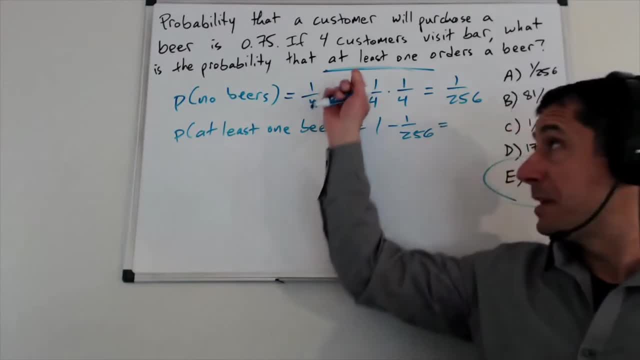 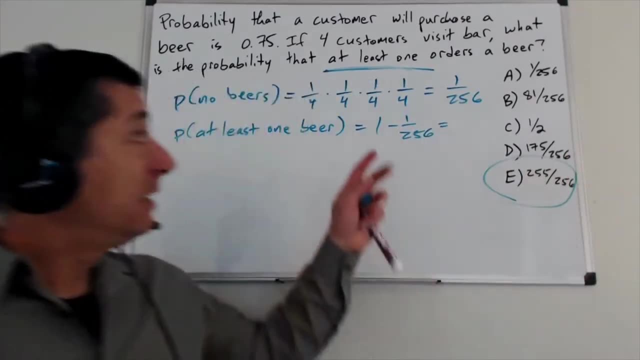 and combinatorics questions every once in a while. So just make sure that jumps off the page at you and you think through the intuition. What is the probability that you select a household with the opposite or better phrasing might be? what's the complement of that thing, In this case at? 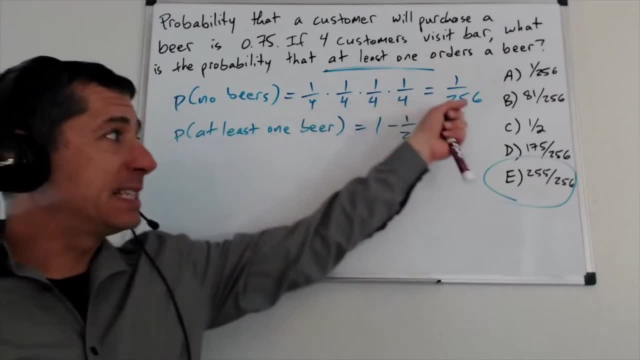 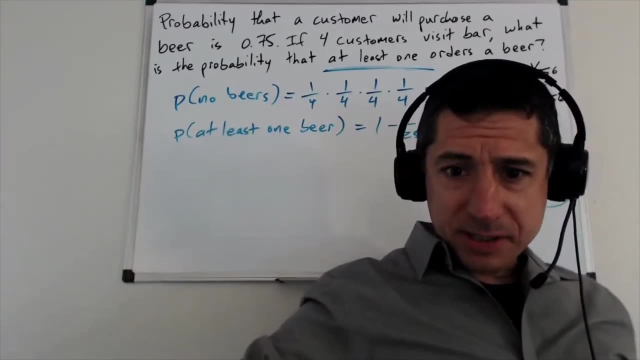 least one orders a beer. Complement is: nobody orders a beer. That's really easy to calculate and there's very little math involved in the end. All right, Now we're going to get into slightly tougher questions in this next third of the video. Good luck to you. 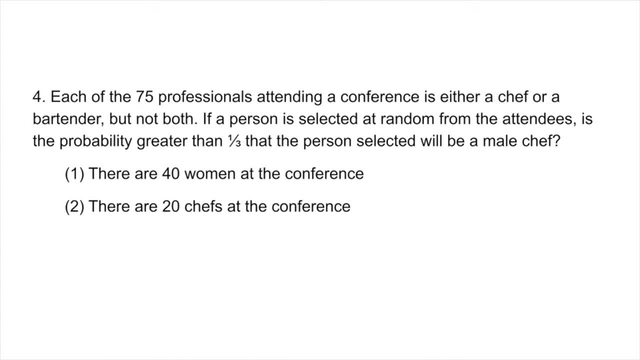 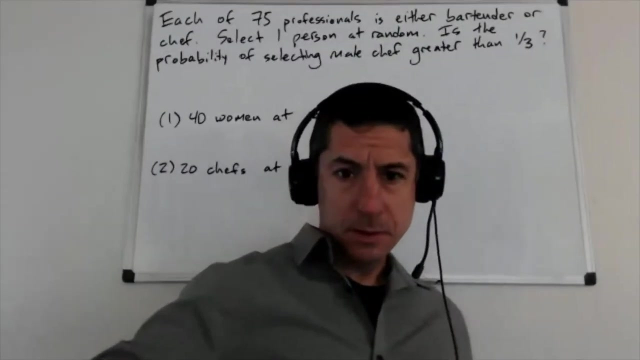 All right. Thank you so much for watching. I'll see you in the next video. Bye-bye, Bye-bye, All right, If you need another minute, feel free to hit that pause button. Okay, Now we're getting into questions, where it's not going to be as easy as it used to be. 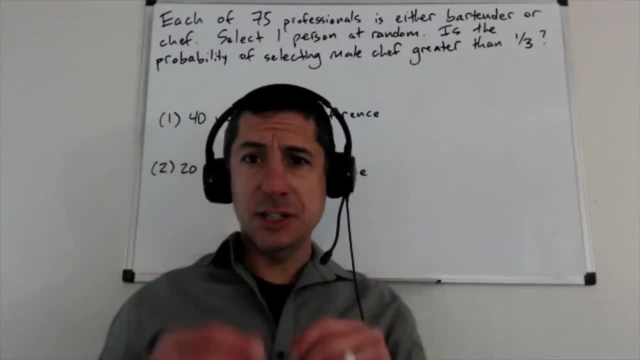 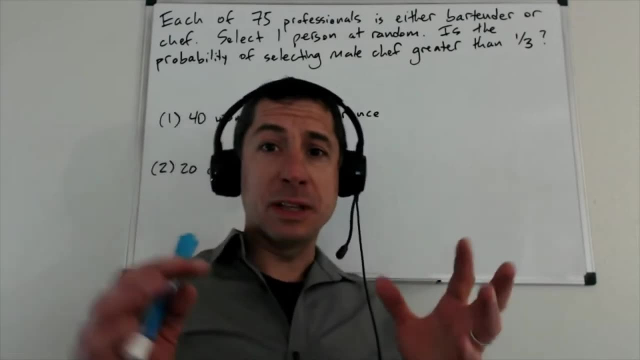 It's not just about the mechanics Now. it's about applying some intuition or some sort of logic. that's going to get to the question. If you're just kind of using brute force, just multiplying fractions together, this third of the video and the last third of the video, you're going to get. 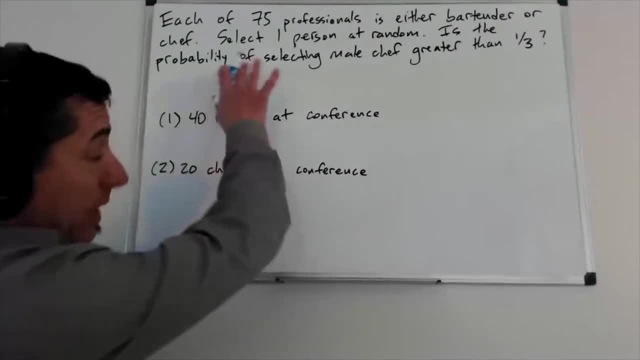 yourself into trouble Here. fairly straightforward sounding data sufficiency question. We've got 75 people at a conference. They're all either bartenders or chefs and we're going to select one at random And we want to know: is the probability of getting a male chef greater? 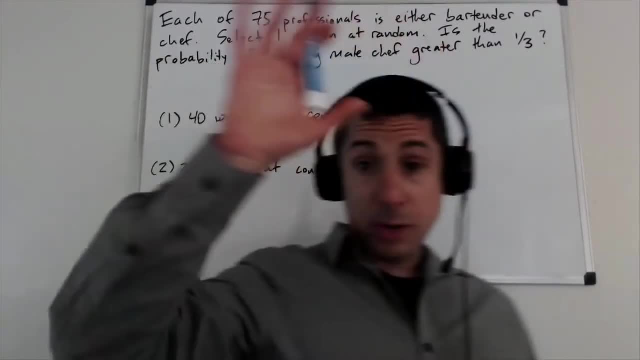 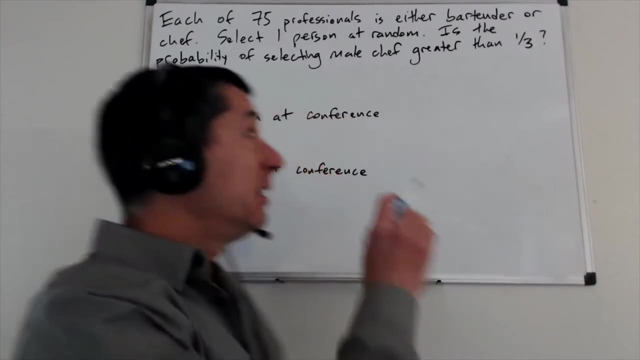 than one third. One of the things we talk about a ton in quite a few of our videos is on data sufficiency. Anything you can do to refresh the question, rewrite it and then you can do it In a way that's logically equivalent. do it every time. That's going to help you a ton. 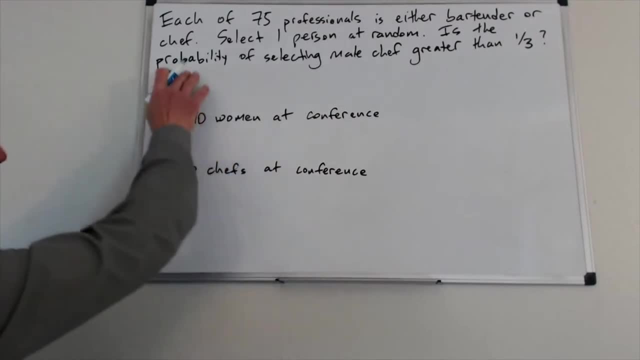 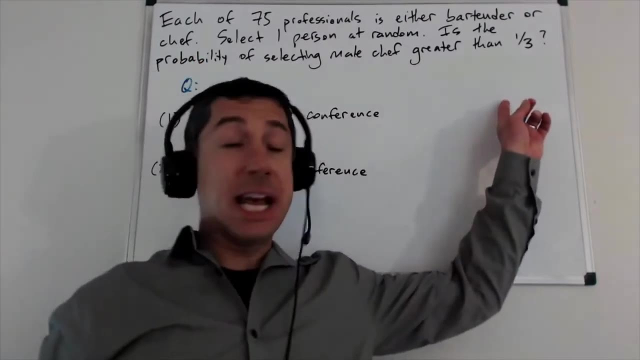 save you a ton of time over the long haul on data sufficiency. So probability of selecting a male chef is that greater than one third. Well, I can rewrite that in terms of the number of male chefs, right, Because I know that there are 75 people there and I want to know: is the probability? 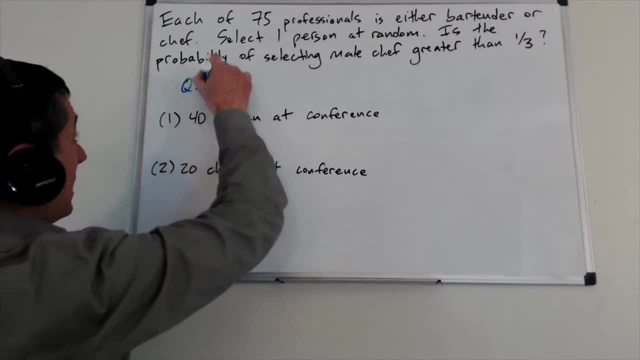 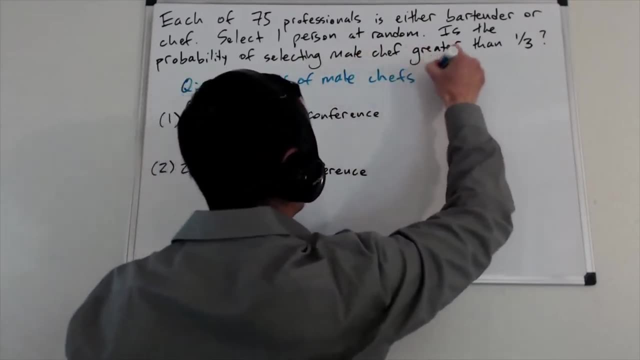 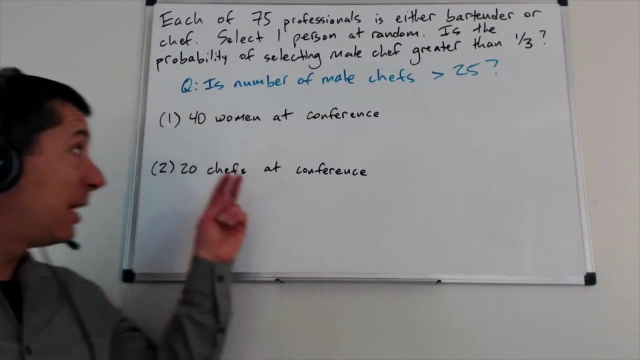 greater than a third. So what I'm really being asked here is: is the number of male chefs greater than 25 at this conference? All right, And then lo and behold. of course our answer choices are in terms of actual numbers. We know that there are 40 women at the conference, which 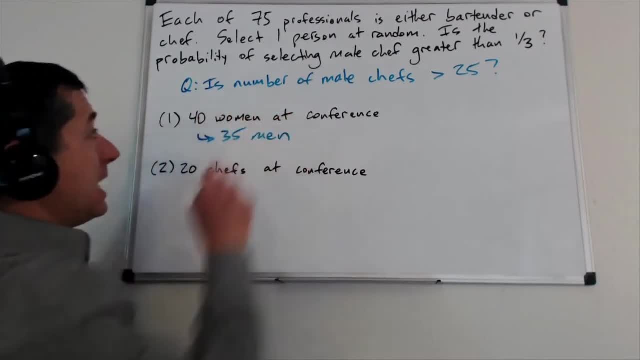 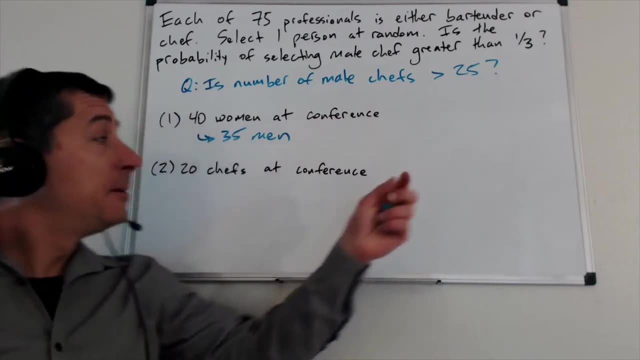 means that there must be 35 men. Is it possible for the number of male chefs based on this, Is it possible for the number of male chefs to be greater than 25? Sure. Is it possible for the number of male chefs to be less than 25? Sure, because we have no idea if those 35 men are all. 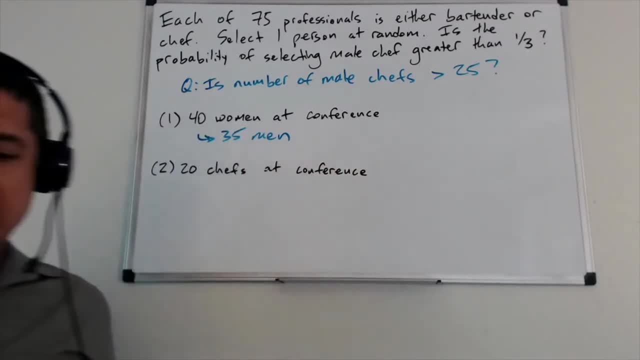 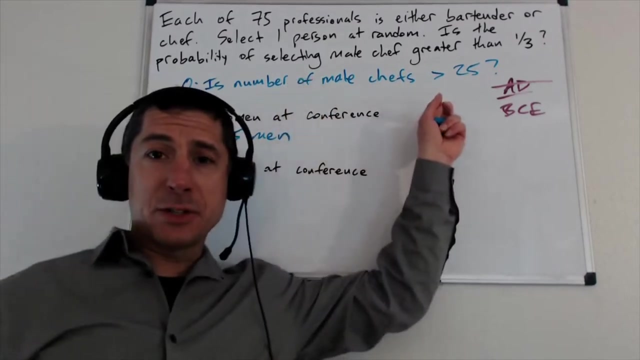 chefs or all bartenders, or somewhere in between. So statement one is not sufficient And we can cross out AD. Now what about statement two? there's 20 chefs at the conference. So if there's 20 chefs, is it possible for the number of male chefs to be greater than 25? Nope, And 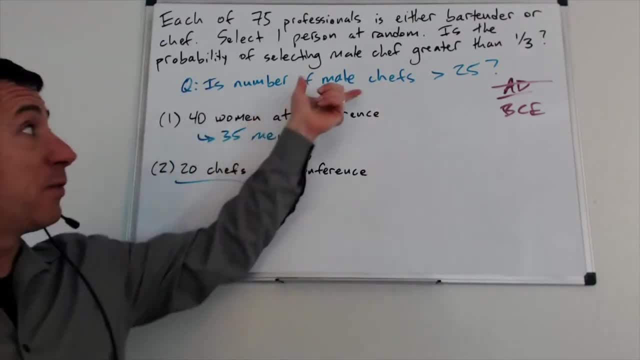 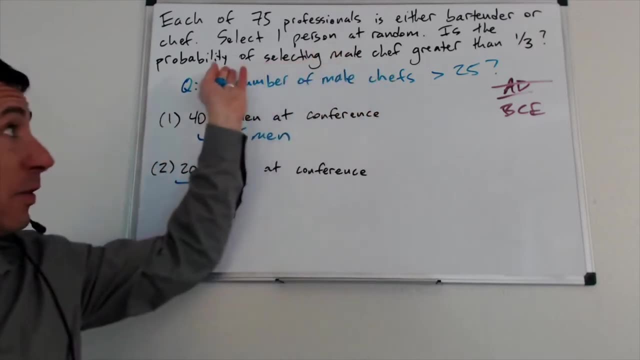 since this is a yes, no question, this is sufficient. We know for a fact the number of male chefs is not greater than 25, since the number of chefs is less than 25.. And therefore, we know that the probability of selecting a male chef can't possibly be greater than one third. 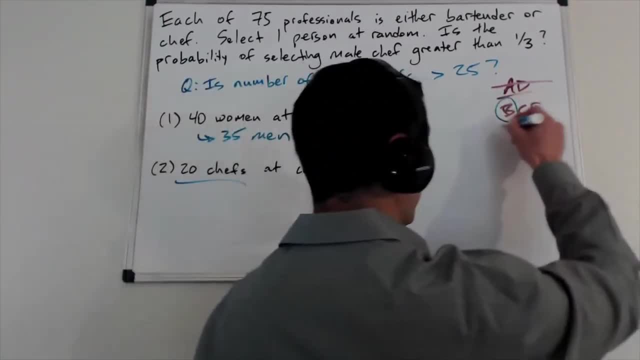 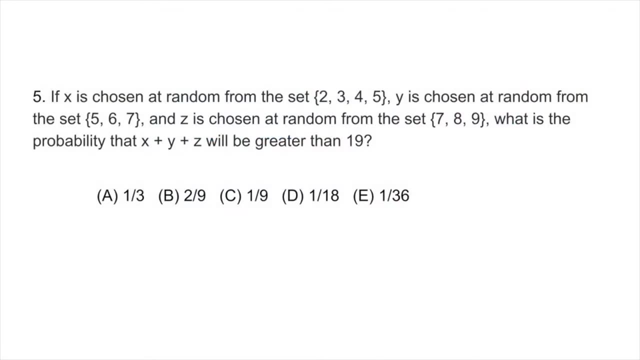 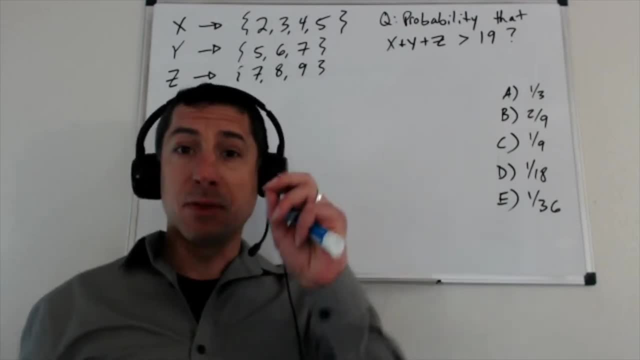 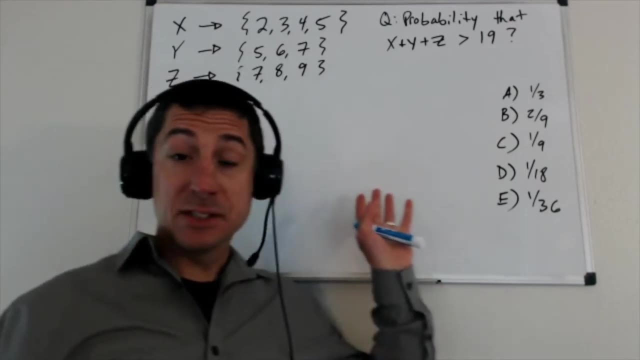 OK. So once again, kind of the theme of this video is: be really, really careful if your instinct is always multiply, multiply, multiply. Just take a bunch of fractions, multiply them together. This is the kind of question that isn't super difficult, Nothing super technical here, But you. 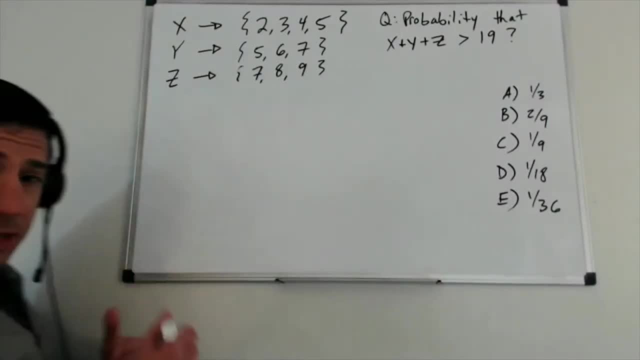 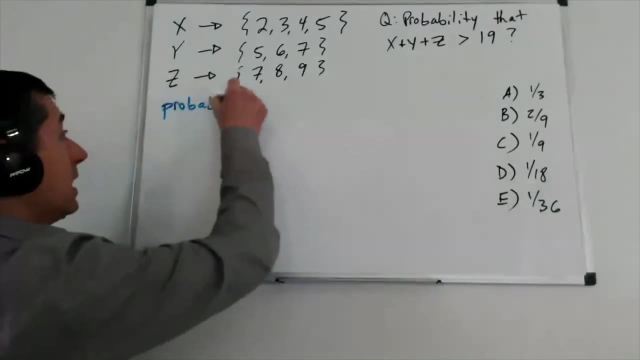 get yourself into trouble if that's your mindset And really, really basic thing. that sounds silly, but we often don't anchor ourselves enough in the definition of probability. Don't think of this as a formula. But what is it? Probability is always the number of desired outcomes, whatever desired might mean in a 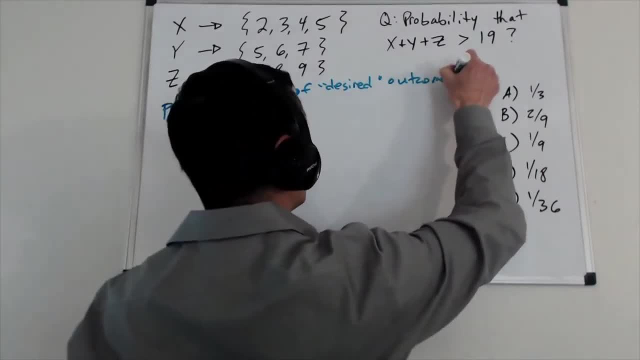 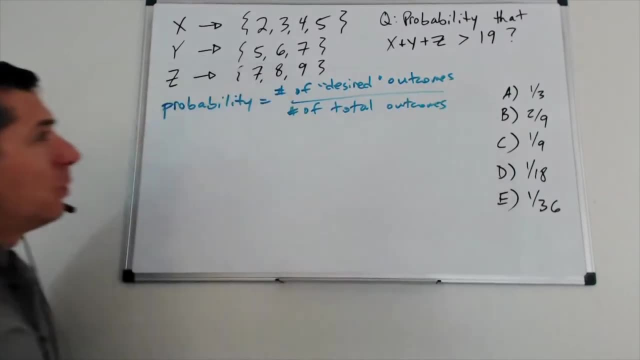 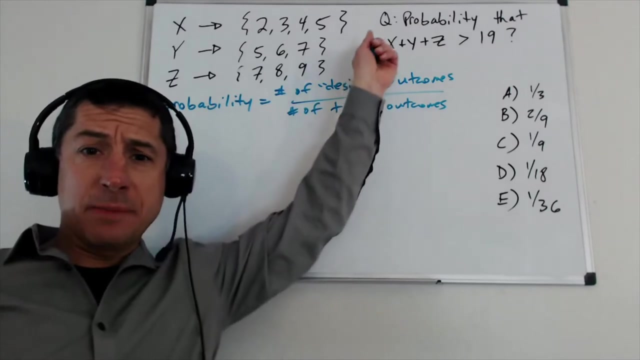 particular context over your number of total outcomes. Great, Well, here let me start by thinking about: how many total outcomes do I have? Well, I've got X, Y and Z. four options for X, three options for Y, three options again. 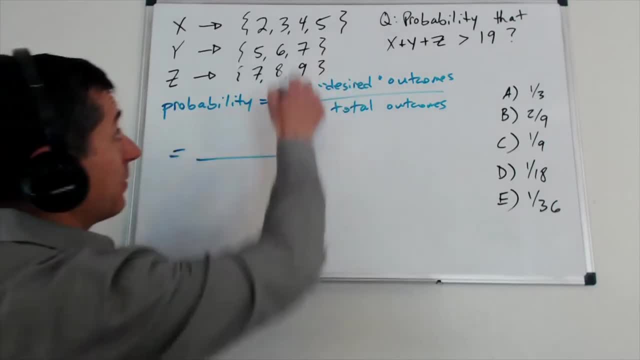 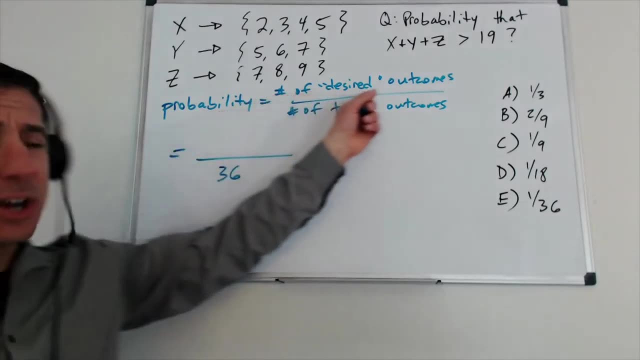 for Z. So my total number of outcomes here has to be four times three times three, which is going to give me 36.. Great, And now the question is: how many desired outcomes do I have? These questions are typically rigged so that it's not going to be. there's not going to. 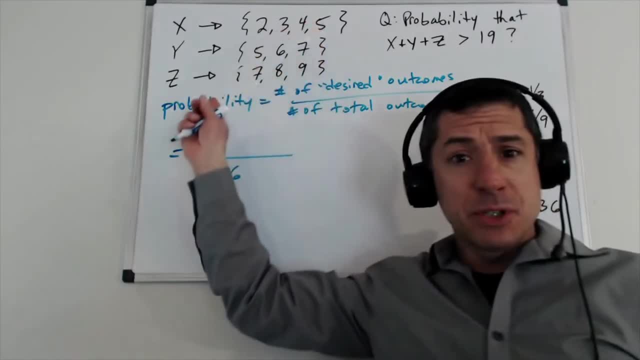 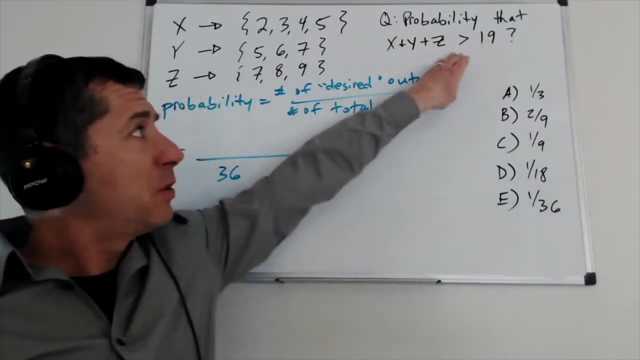 be a ton of different ways to calculate it. Notice that if we take the biggest numbers from each set- so the five, the seven, the nine- we're going to get 21,, which isn't so far from 19.. Also, notice that we're being asked for the probability that X plus Y is greater than 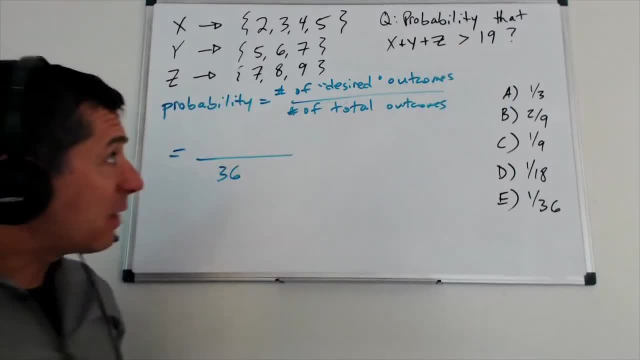 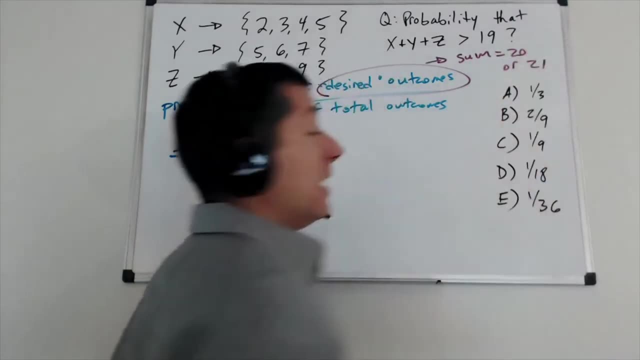 19.. So what is our desired outcome here? Our desired outcome is just that the sum equals 20 or 21.. That's not so bad. Now, how many ways are there to get a 21?? Well, that's just one way. 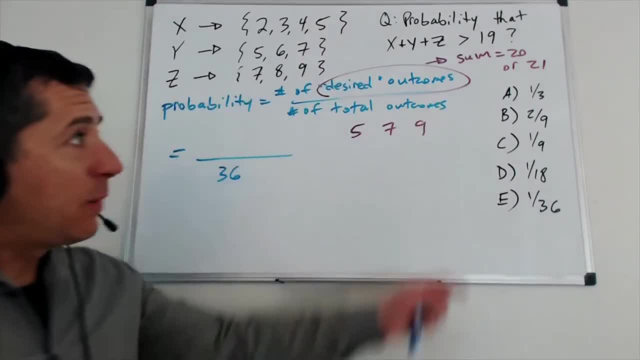 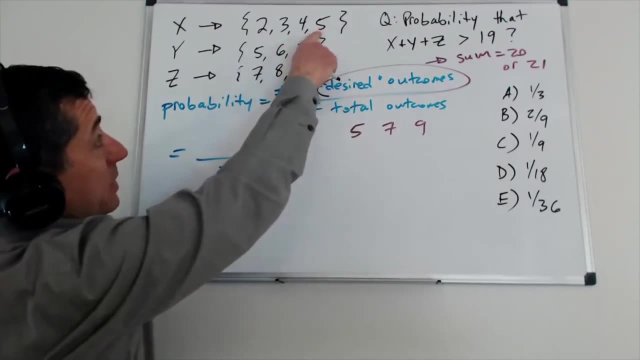 I've got to have five, seven, nine, And now how many ways to get 20?? There can't be that many of them. These are nice consecutive integers in each of these sets, So all I can really do is take the biggest number in each set and turn one of them into. 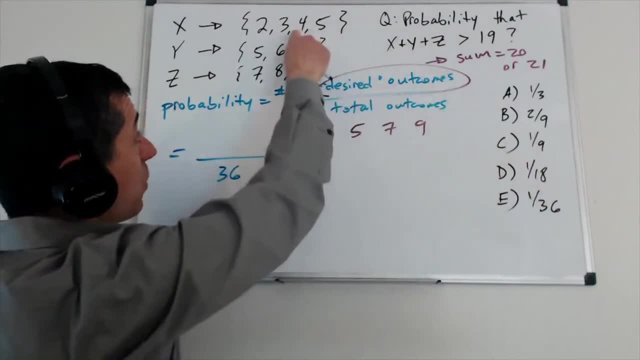 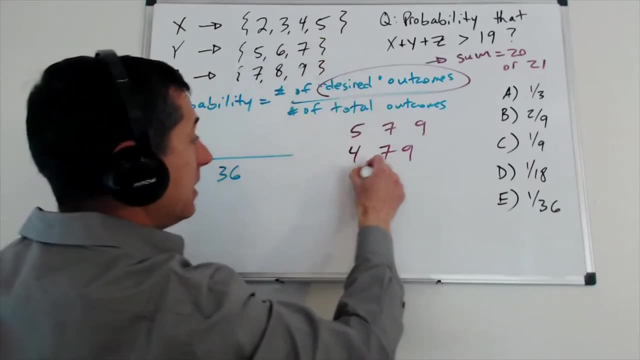 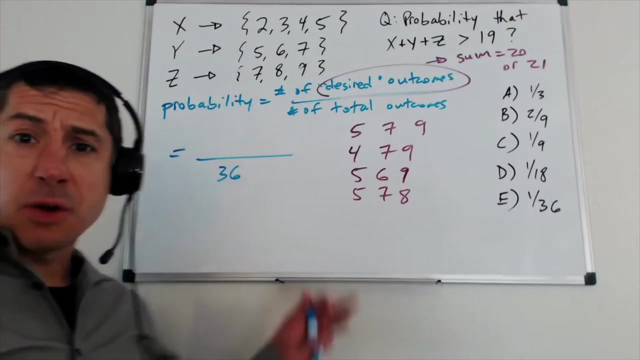 a slightly smaller number. That's the only way I'm going to get 20.. So I could have four, seven, nine, or I could have five, six, nine, five, seven, eight, And that's it. There's very clearly no other ways to do it. the way these numbers are set up. 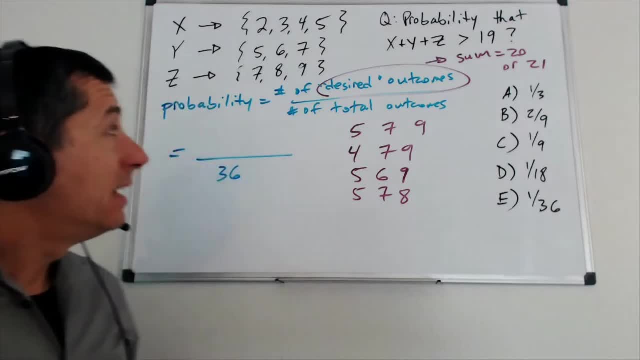 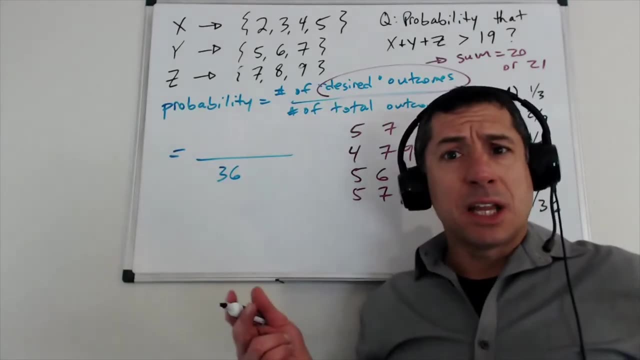 And again, very, very typical sort of thing you might see on the executive assessment of the GMAT: A little bit intimidating. If you try to be too formulaic about it, get yourself into trouble. Looks like it's going to be a lot of work, but in the end it's not a lot of work because 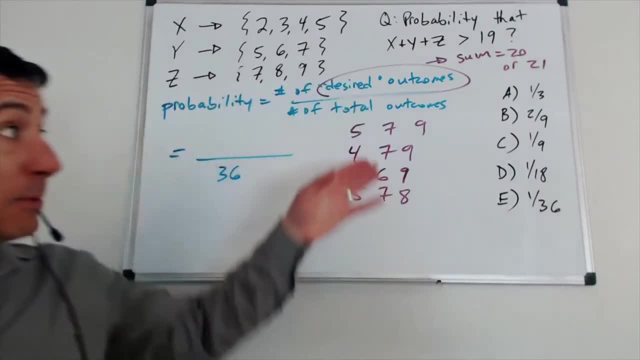 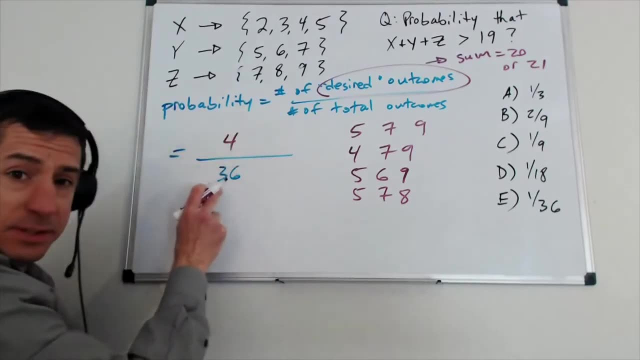 the numbers are arranged in a way that there just aren't that many options, aren't that many desired outcomes. I've only got four of them, and that's the end of the story. So my probability here is those four desired outcomes over those 36 total outcomes. 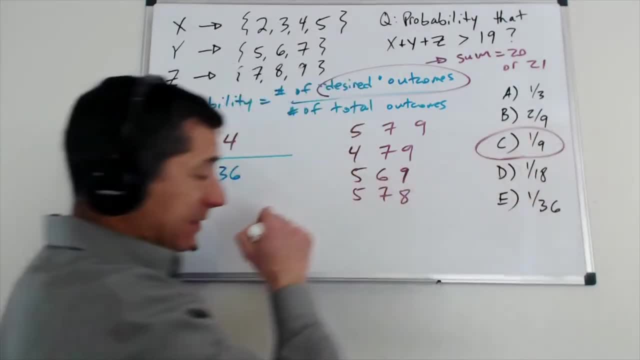 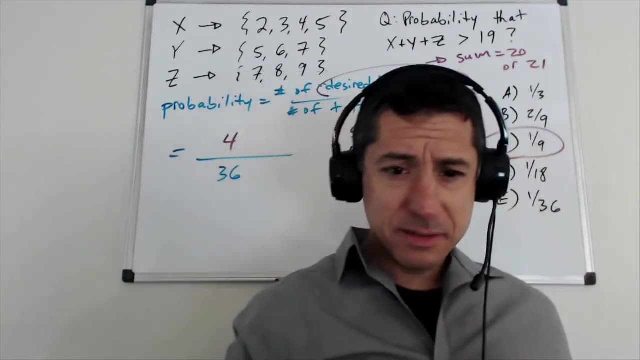 That's going to reduce to one ninth And my answer is C. All right, One more kind of mid-level, sort of funky, sort of conventional, all at the same time probability question, and then we'll ramp it up in the last third of the video. 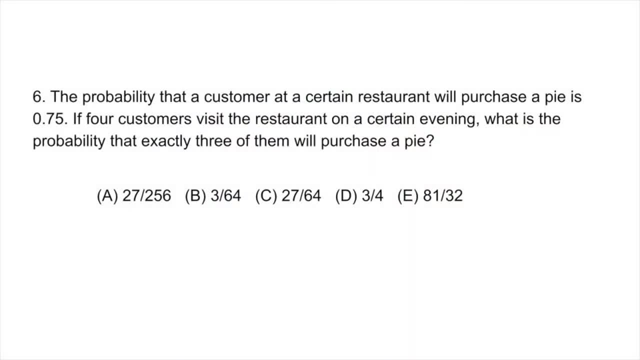 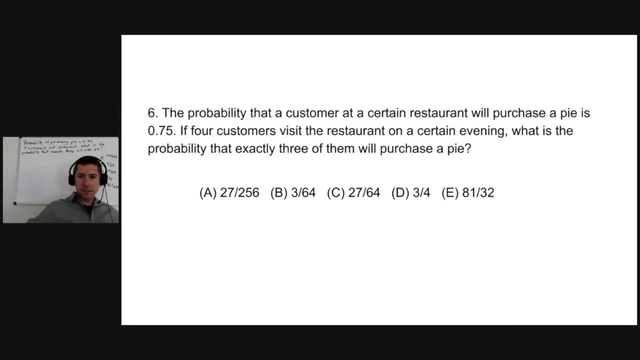 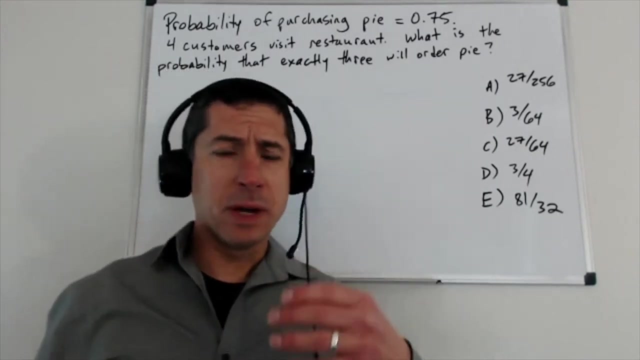 All right, All right, you, you all right if you a little bit more time hit the pause button. so, leading to this question, i called it sort of conventional, sort of funky at the same time. but why do i say that i call it sort of funky? 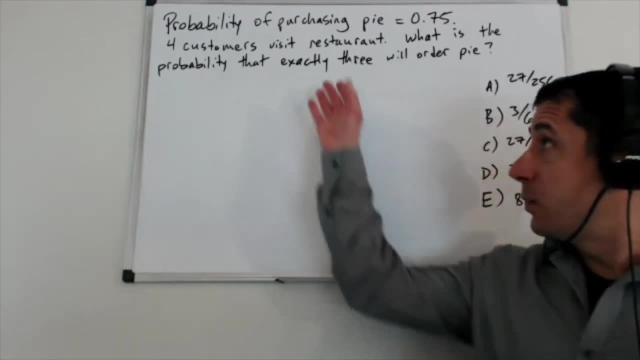 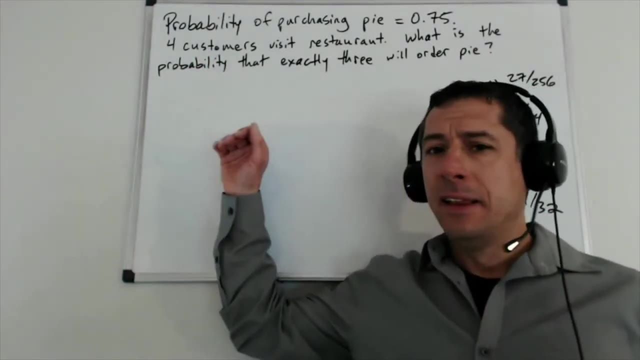 because this is a relatively rare thing on the gmat. how often are you going to see a question that asks you for exactly three of the four things, or exactly one of the four things or exactly two? very, very rare variant. maybe there are three or four official questions in print out of the. 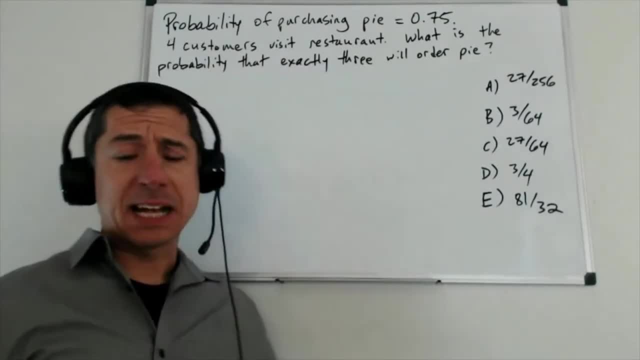 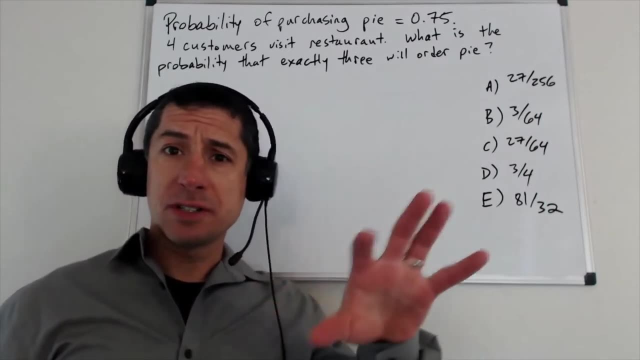 literally thousands that have been published that get at this exact concept. so in that sense, not going to see it a whole lot. um, is it conventional in another sense? sure, because the kind of logic you need in order to solve it is something that you should be able to master pretty easily without. 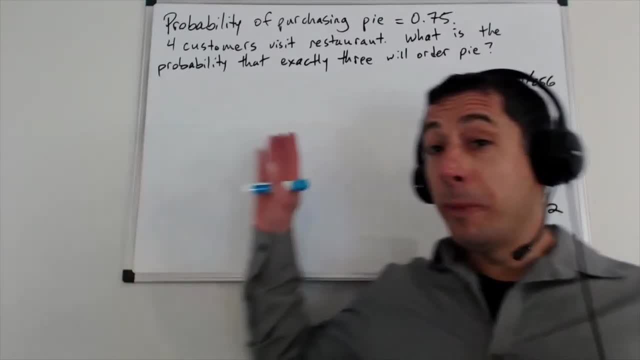 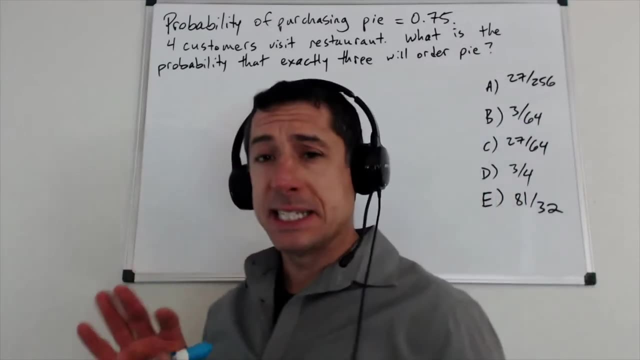 knowing anything terribly technical now. that said, a whole bunch of different ways to solve this question, so you could solve this using binomial expansion. if you don't know what that is, do not worry about it at all. it is not something that is necessary by any means. on the gmat, some people 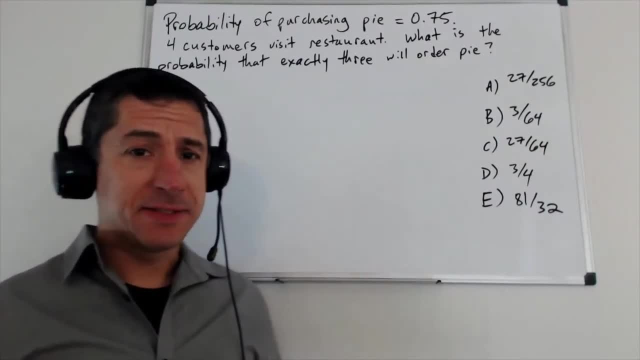 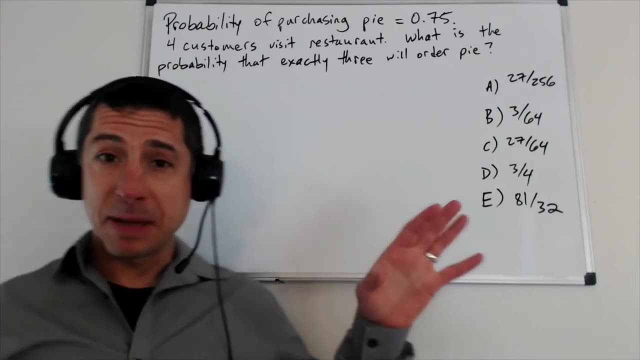 with really strong technical backgrounds in math like to solve it that way. good for them. that's fantastic. you could solve this using combinations again. if that's something that you're really comfortable with, you could solve it using combinations again. if that's something that you're really comfortable with. good for you. not going to talk about that here. we have a separate. 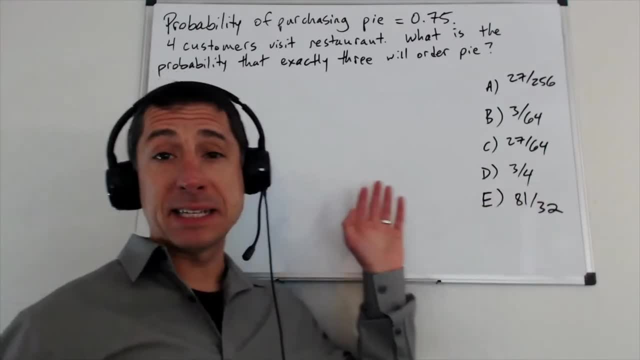 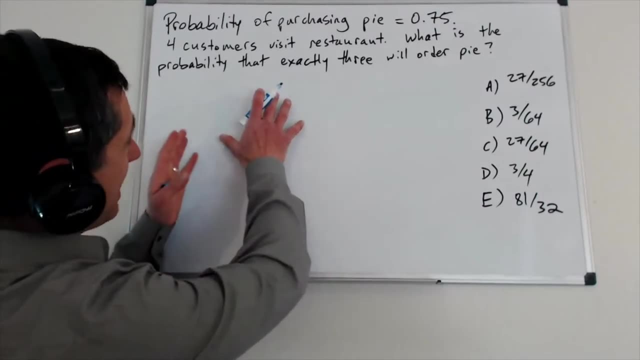 video on combinations and i think it's just easy to solve this with a little bit of logic and basic, basic probability. so that's our third path, that's what i'm going to show here. so i could kind of start by saying, okay, exactly three will order pi. so just to write down the exact numbers here. so 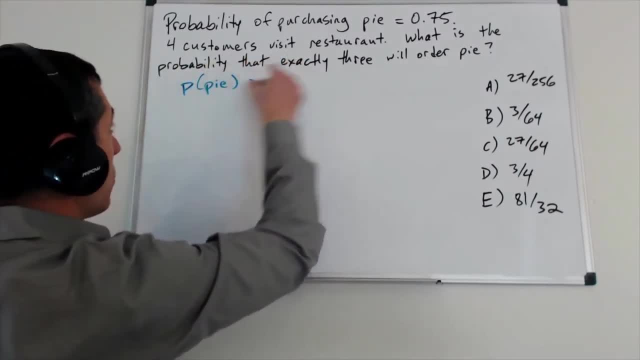 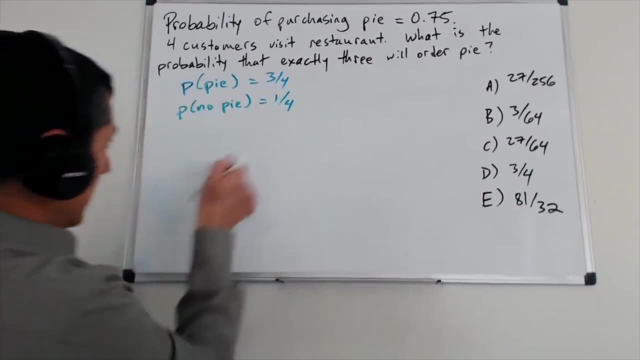 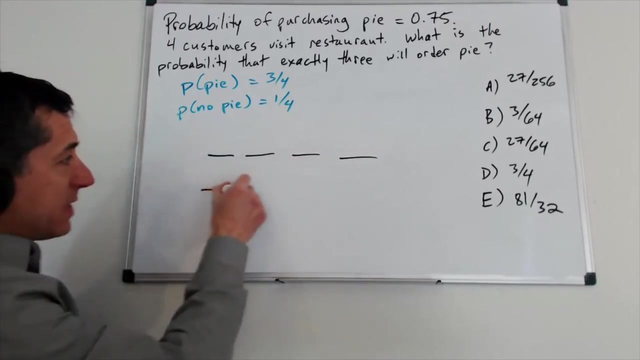 probability of ordering pi is three-fourths, probability that you do not order a pi is one-fourth. and i could kind of go through and say, well, let me kind of do our good old thing of kind of these: four different selections, four different customers walk in and there's a whole bunch of different ways that you could get at this, because 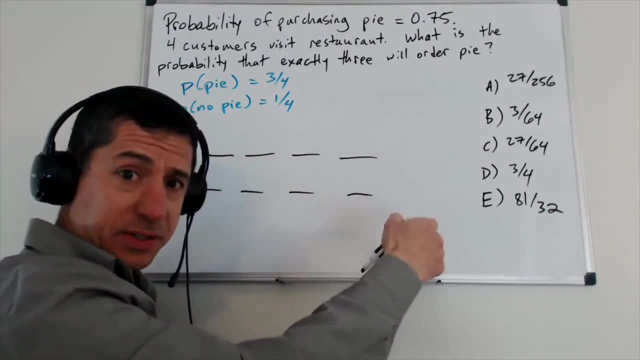 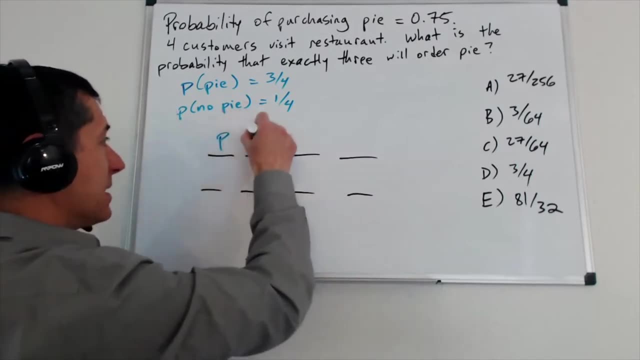 it doesn't matter which of these customers does and does not order the pi, as long as you have three that do and one that doesn't. so how many ways are there to set that up? well, you could have the first one order pi and the second order pi orders pi and the third one orders pi. no pi for. 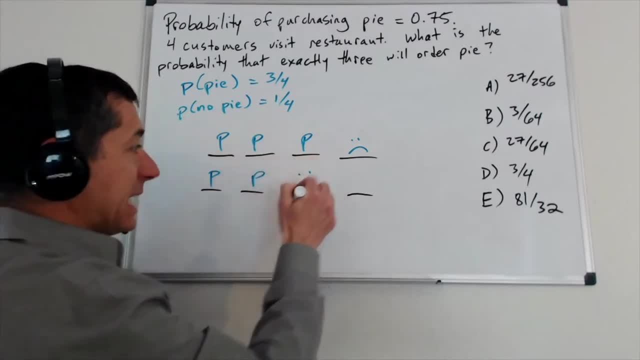 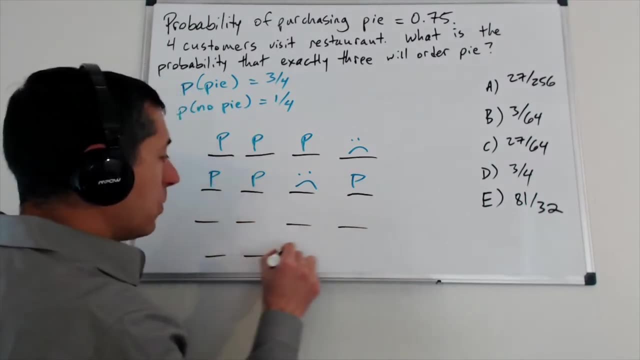 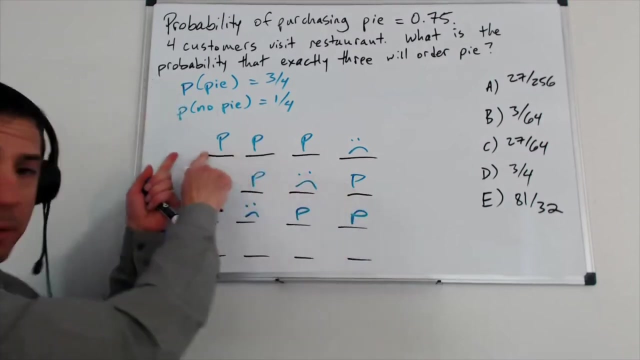 that last guy, same idea, except it's the third one that doesn't get the pi, and so on. i'm not saying you need to draw this out. what is really useful is to recognize the concept here that you have the probability that let's say, let's say we fact that, the probability that the 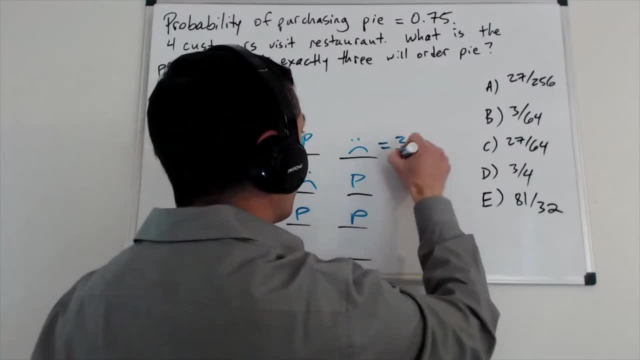 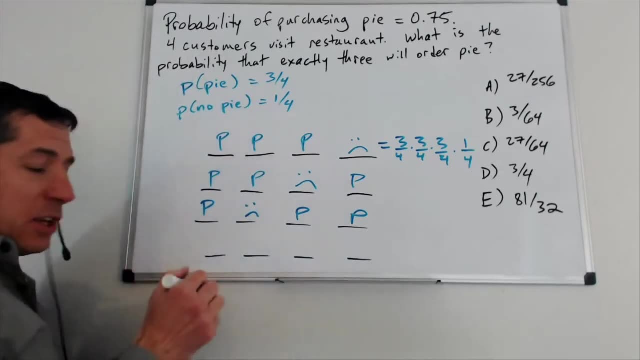 last one doesn't order pi, but the first three do, and we get three-fourths times three-fourths times three-fourths times one-fourth- great, my point is that you're going to have that exact same probability three more times, oops. so first one doesn't order pi. 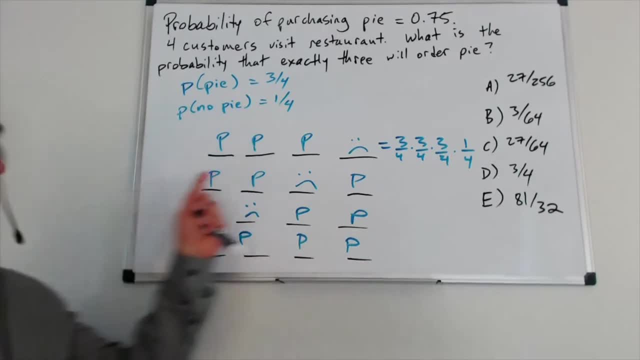 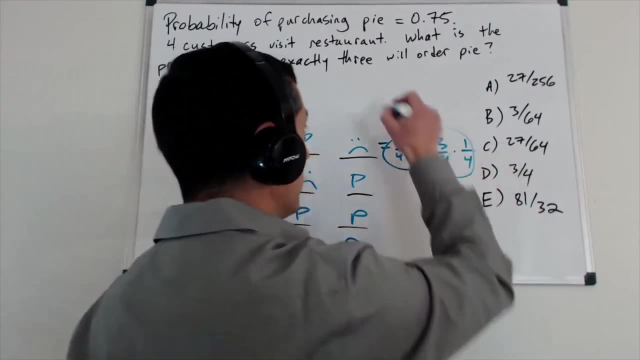 second one, third one and fourth one do so. there's four ways to rearrange this. so if you can recognize that the probability that the first three do order pi and the fourth one does not is this number, and then it's going to be exactly the same if it's the third one, that doesn't get. 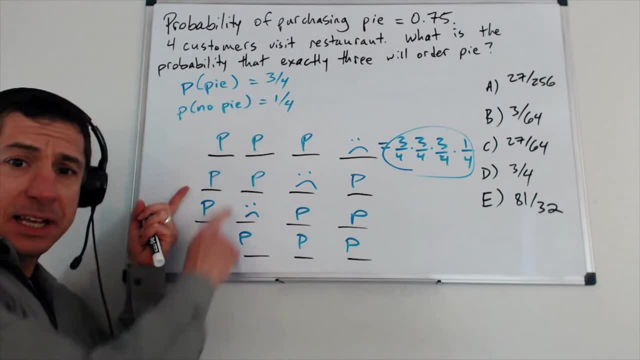 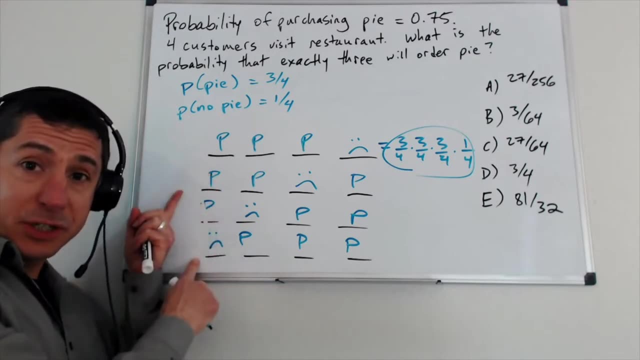 pi, or the second one that doesn't get pi, or the first one doesn't get pi. as long as you can recognize that logic, you can solve any question that looks even vaguely like this, because all you have to do is recognize that intuition and say, well, i'm going to take this original probability. 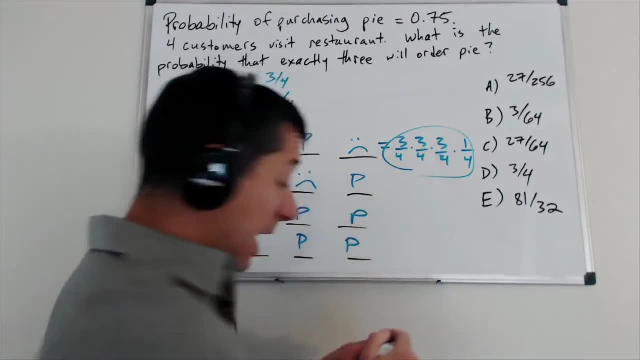 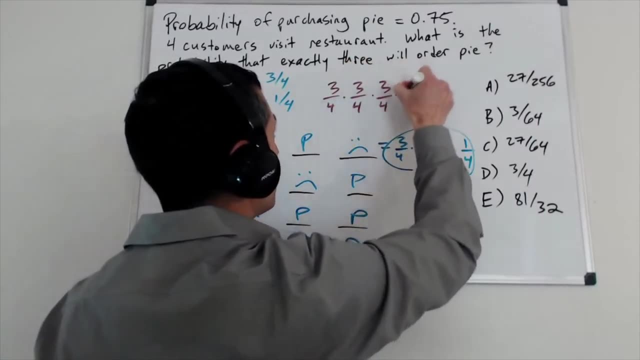 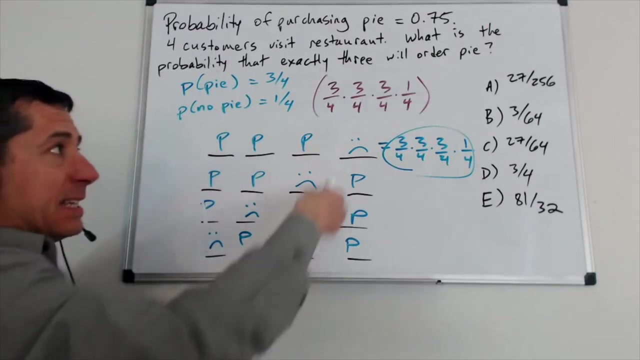 multiply it by four, and i'm done so. here we get. i'll rewrite all this. so three-fourths times three-fourths times three-fourths times one-fourth is the probability that the first three order pi last one does not. but that's going to be exactly the same as these. multiply this by four. we can cancel out these. 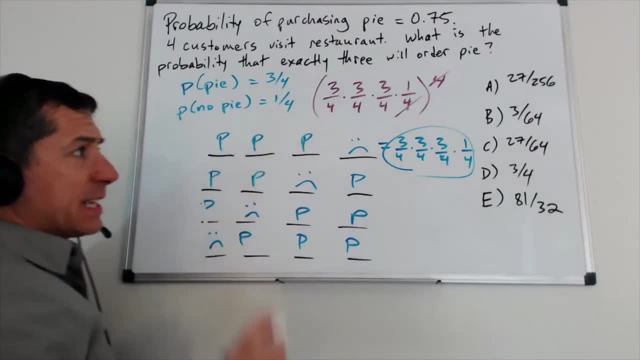 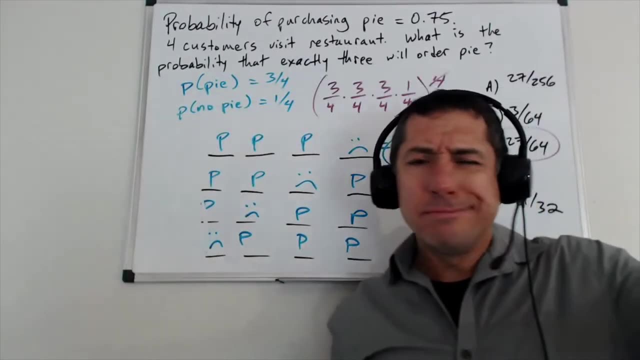 fours and we just get 27 over 64 and our answer is c. so a lot of what happens on the gmat, especially some of these more i don't know, exotic questions types. a lot of the time it's basic, basic foundations. they start building a little bit. 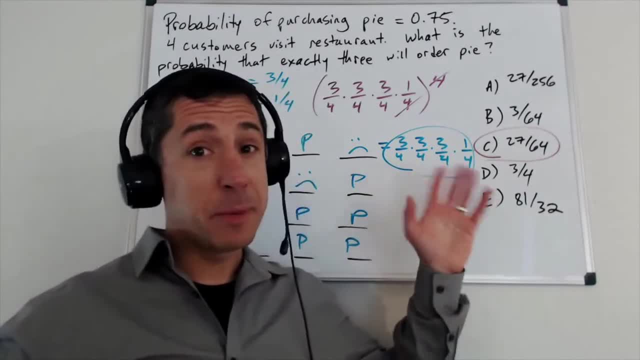 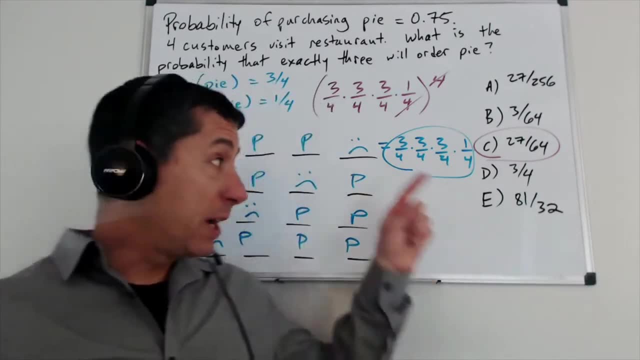 of logic on top of that- and it's not that you need to know anything more technical again- you could find a mouse expansion, a whole bunch of combinatorics. you can do that. that's wonderful. if it works for you, fantastic. if not, if that's not your cup of tea, no worries, just apply. really. 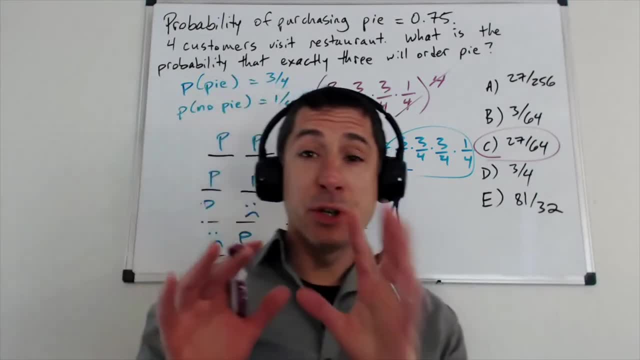 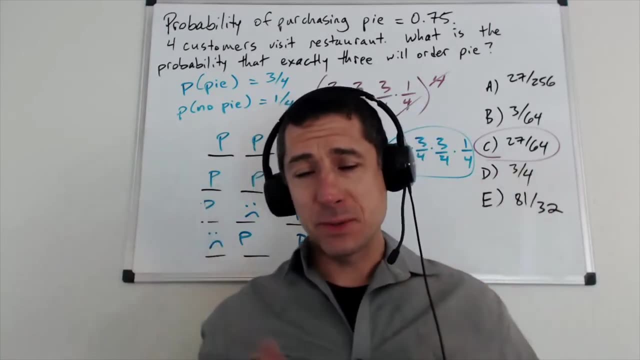 strong reasoning and you're going to be in really, really good shape. all right, we're two-thirds the way through the video. this last third, so this next question, i think, is the toughest in the video. it's: it's within the boundaries of the gmat. it's based on a few things we've seen before. 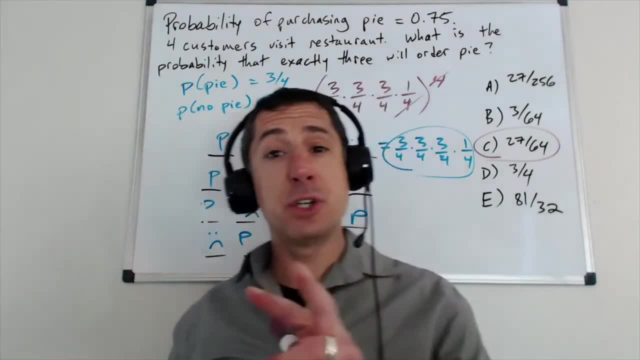 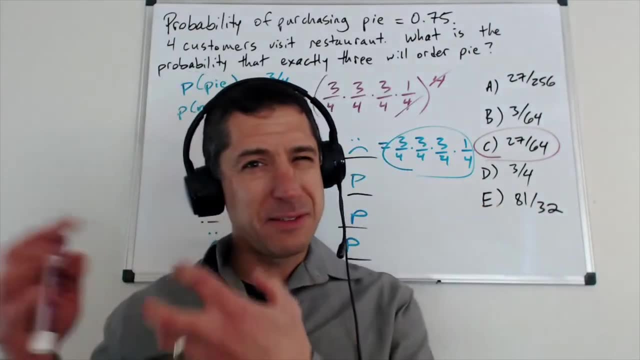 super, super tough about as hard as probability gets from there. we're going to cover a couple, two questions that are not really about probability at all. they use the word probability built on a very, very super basic foundations of probability, but it's really kind of combining other things. i 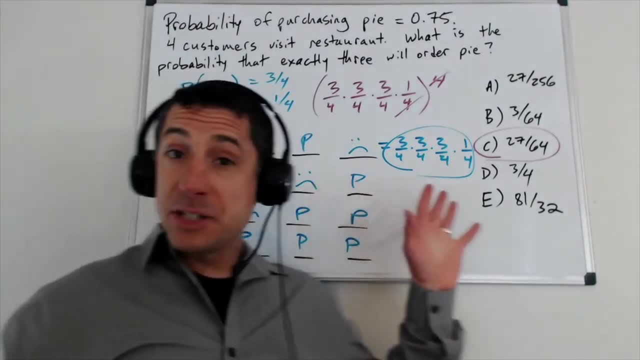 want to illustrate a couple of those at the end. so, again, if your score goals are modest, you don't really need to watch this last third of the video, but if you're having a good time, stick with us and this one will give you a good challenge. 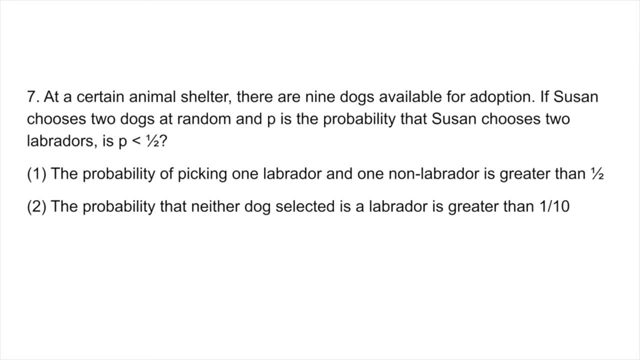 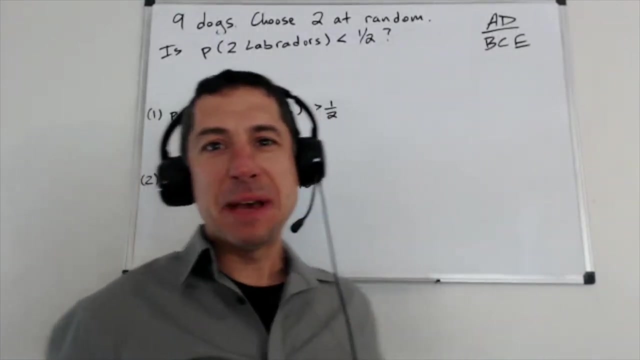 you, you, you. all right, if you did a little more time, feel free to hit the pause button, as always. uh, look, this is about as hard as probability questions get on the gmat. if i were to go through the several thousand official questions that have been published or things we've, 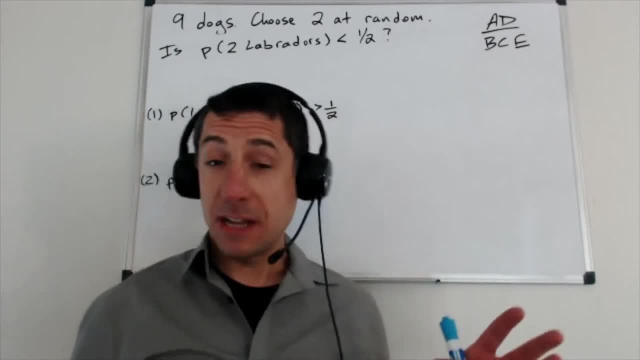 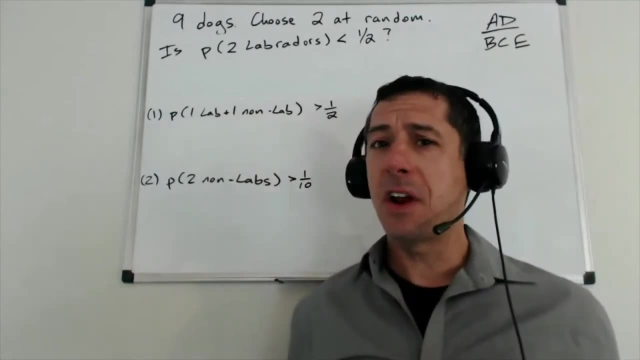 said in the past that have been published and that have been published and that have been published. on the actual exam, i don't think we're going to find five questions that are tougher than this one. now, this is derived from official questions there. there are some that get at the same kinds of concepts in similar ways, but there are very, very few of 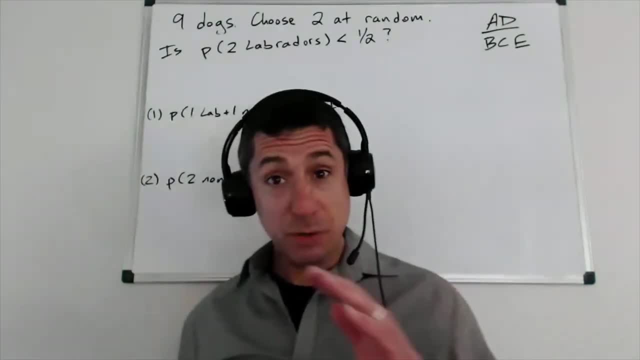 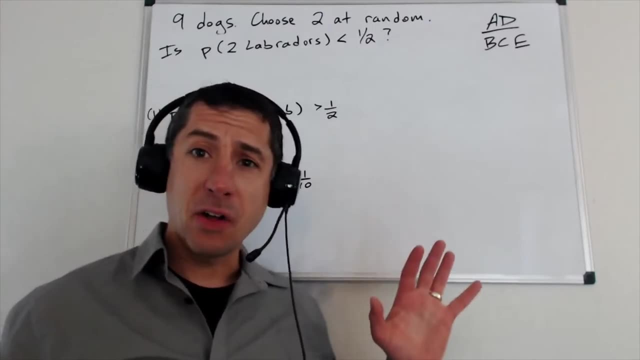 these very few that are harder. so if you found this easy, good for you, you're doing phenomenally well. if you struggled a little bit on it, you're probably still doing pretty well. if it was just minor struggles, if you got obliterated by this, no shame in that at all. this is not. 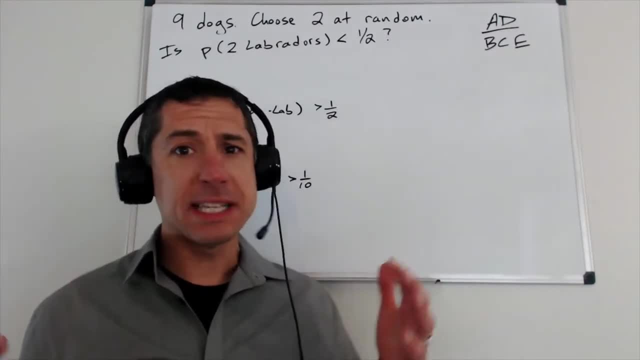 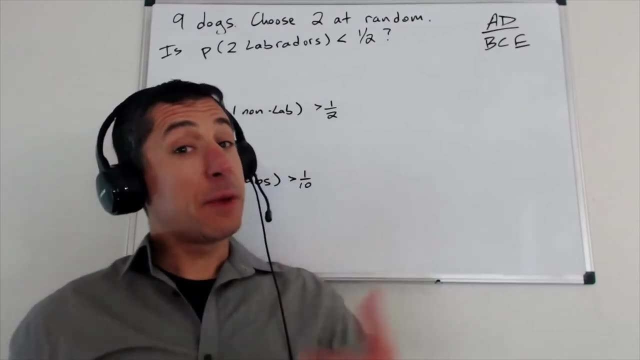 something you absolutely need to get, especially if your goals are something like a 47 or a 48 or anywhere below that on the gmat quant. this isn't something you need to lose too much sleep over now. that said, the thought processes definitely are things that are. 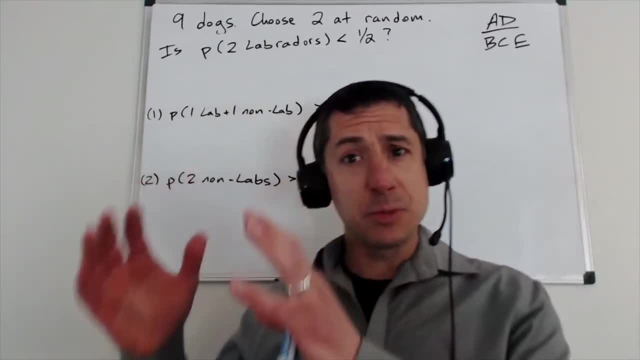 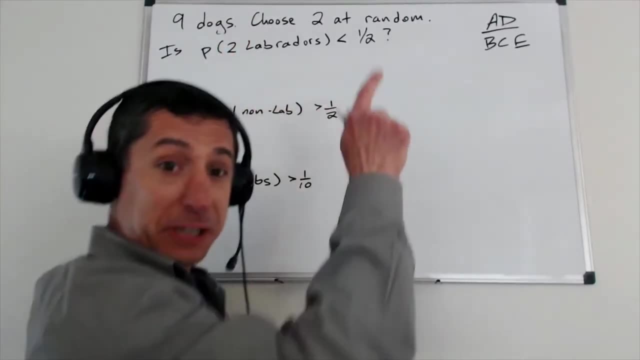 fair game. it's kind of a matter of toggling back and forth between a little bit of algebra and a little bit of intuition, so i'm going to try to model that here. all right, we got nine dogs at the animal shelter. we're going to choose two at random. we want to know the. 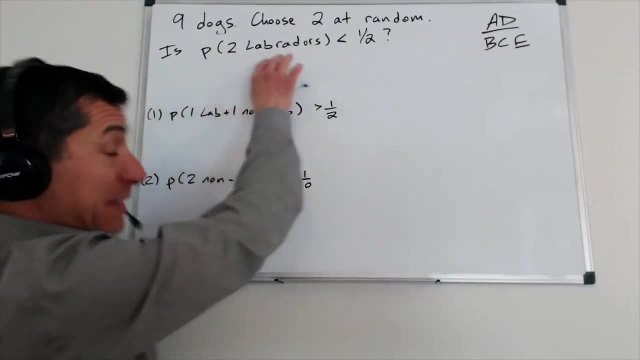 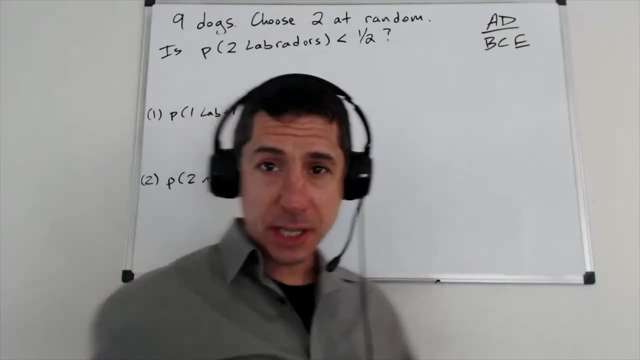 probability that we get at least. well, we want to know whether the probability of getting two labradors is less than a half. now, as always, on data sufficiency, the more i can do to rephrase that question logically equivalent ways, the better off i'm going to be. so let's try that. 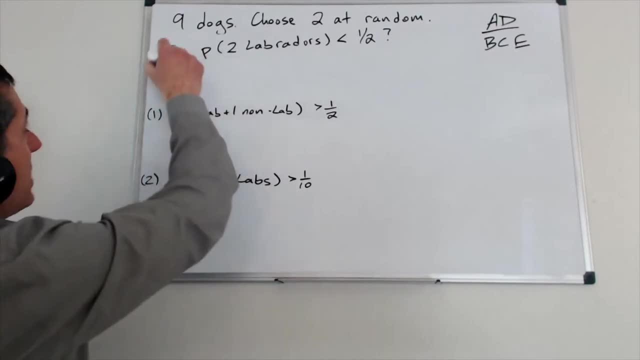 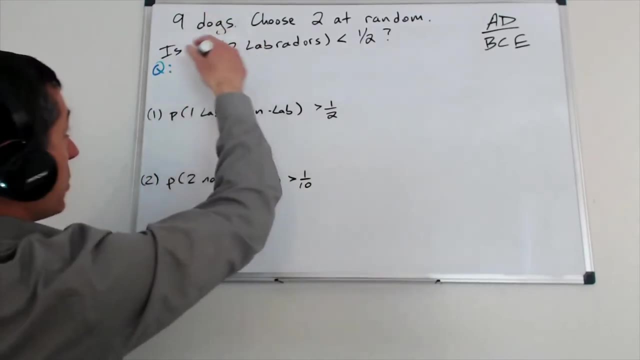 here and see where i'm going to end up. i'm going to end up getting two labradors and i can take it. so that question- probability of getting two labradors- if, if we let l equal the number of labradors, let's see where that algebra is going to take us. so on that first. 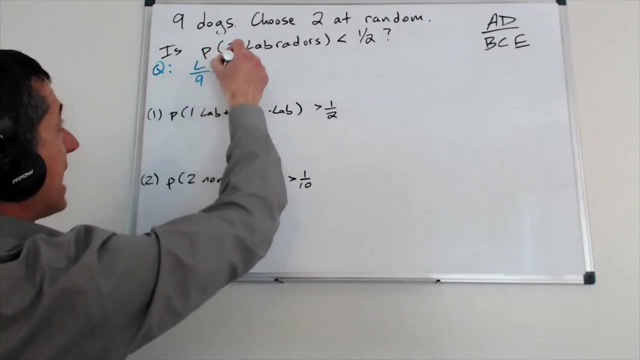 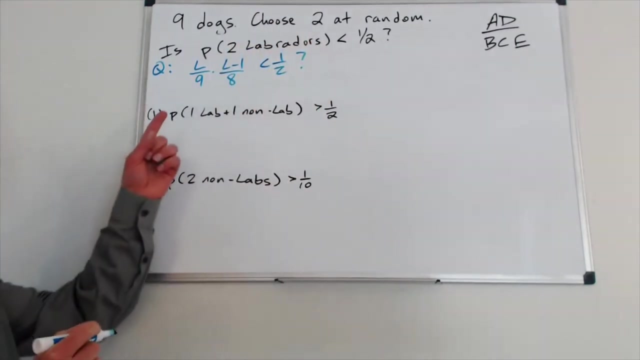 pick: probability of getting a labrador is l over nine. second pick: well, there's going to be one fewer labrador available, one fewer dog overall. so there's my probability of getting two labradors and i want to know: is that less than a half now? next thing i want to do here: i can, i can. 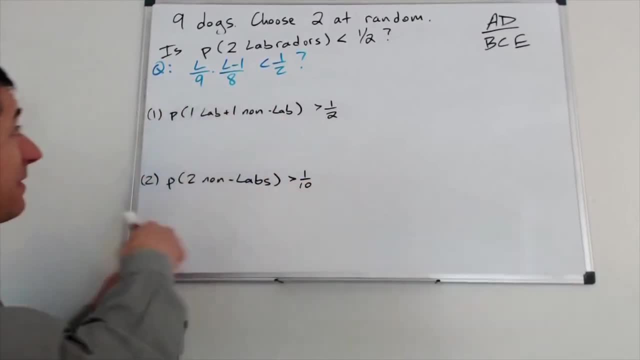 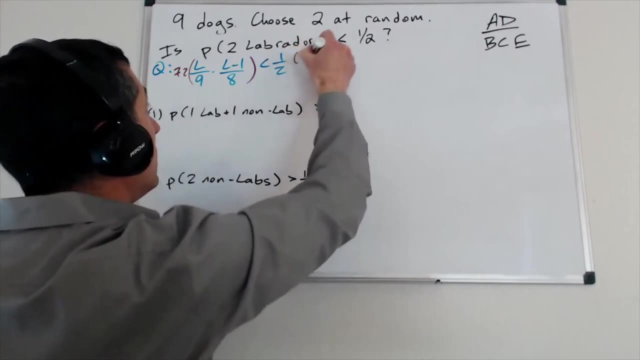 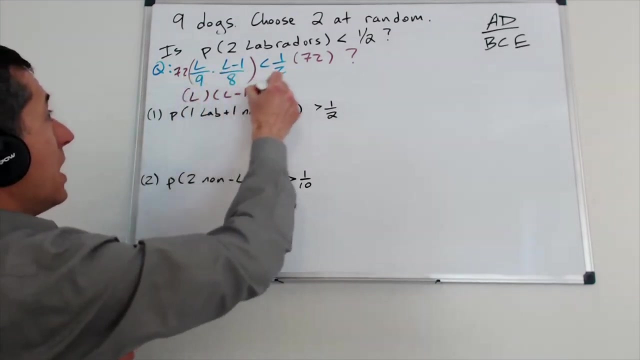 rearrange a little bit. so my first instinct: nine times eight is seventy two. so what if i multiply both sides of the inequality by seventy two? so what's going to happen there? so then i get l times l minus one, less than thirty six, and you've seen this modeled in other videos if you've been with us on these branson in. 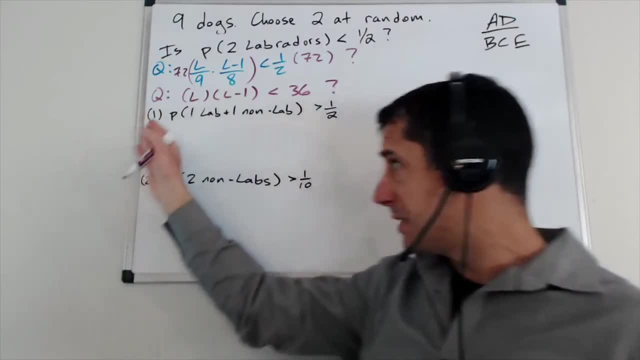 particular in some of those videos that look pretty heavy after algebra and data sufficiency. i always kind of leave that question in the comments section. so let's view some of those ideas i mentioned earlier and hopefully we'll get to that in the next question. so let's see. 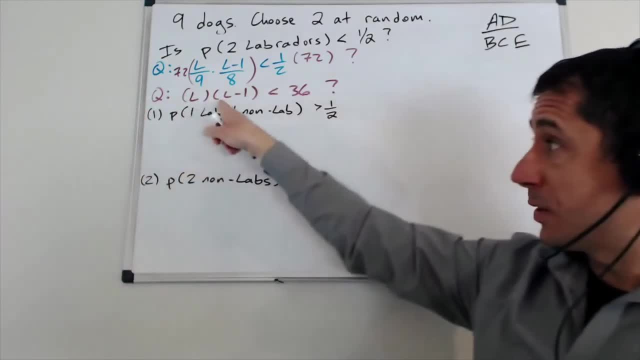 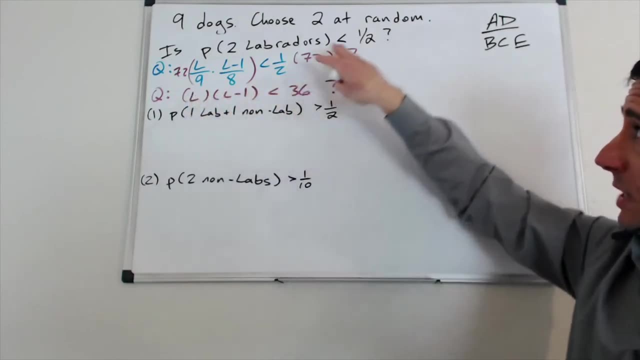 in there, just so that I'm clear about what's a fact given to me and what's the question being asked. So my question here is: is the number of Labradors times one minus that less than 36, logically equivalent to this? So what does that tell me? Or how am I to rephrase that again? 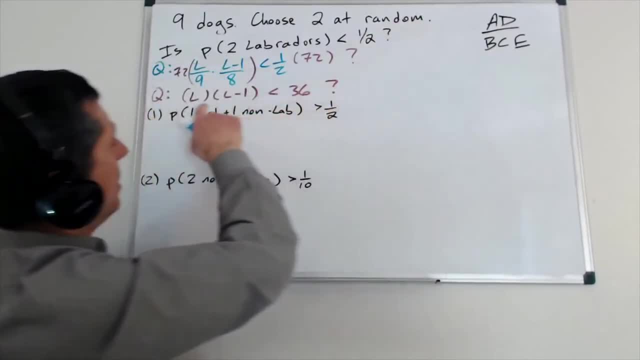 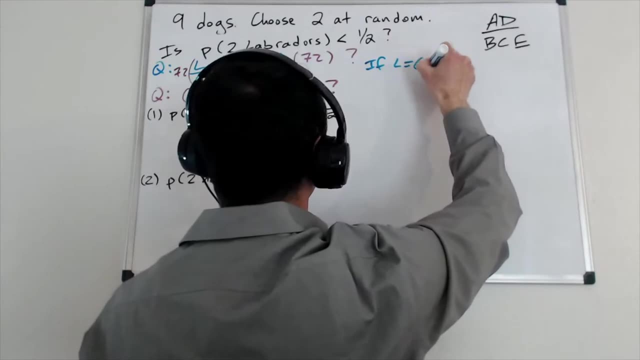 Well, when is this going to be the case? So my first instinct is: okay, if there's six Labradors, is this going to be a true statement? So if L is equal to six, then my answer to this is yes. 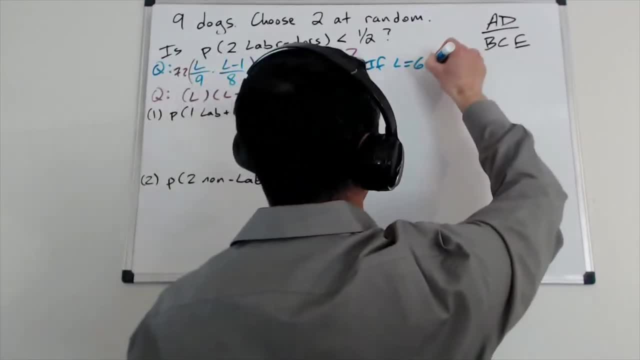 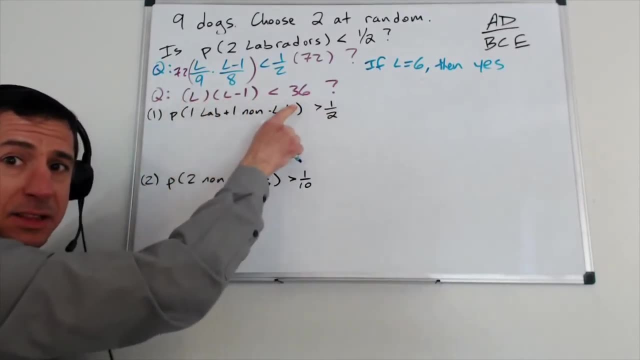 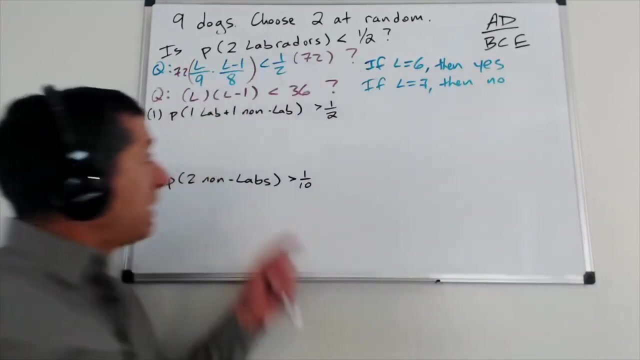 six times five is indeed less than 36.. And now what if I go one bigger than that? Seven times six, is that less than 36?? No, And the answer to my question is no. So think through that a little bit. My probability is always going to be less than a half if I have six Labradors. 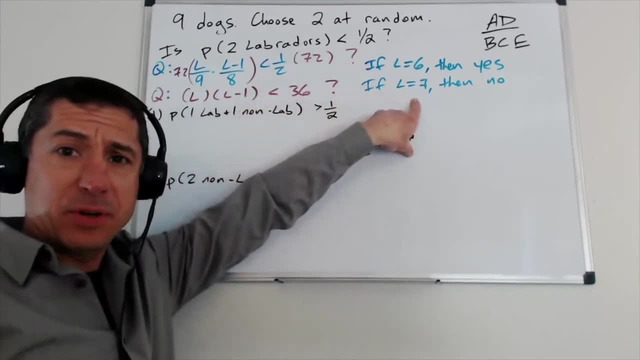 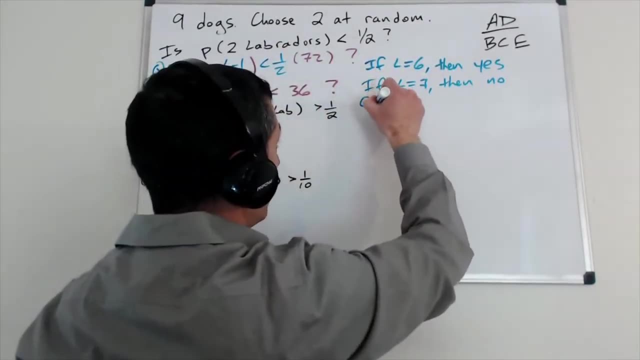 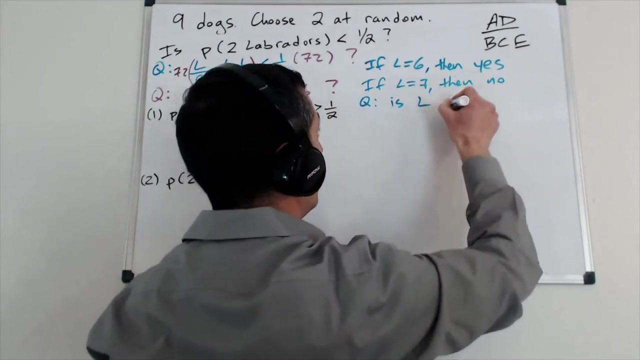 Or fewer. If I have seven, eight or nine Labradors, then it must be true that that probability of getting two of them will be greater than a half. So now I can rewrite this question. So is the number of Labradors- sorry- less than or equal to six? 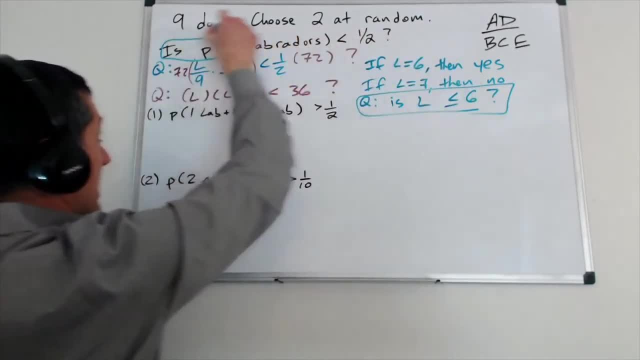 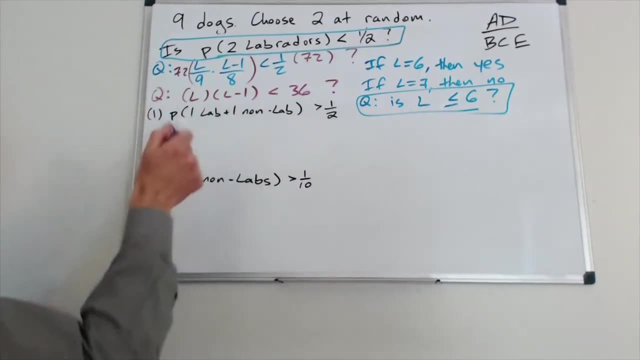 logically absolutely equivalent to this guy. Okay, great, Let's tackle statement number two here. So the probability that we have we get one lab and one non-lab is greater than a half. This is where it gets really fun. So L over dine. let's say we get a Labrador on the first pick. 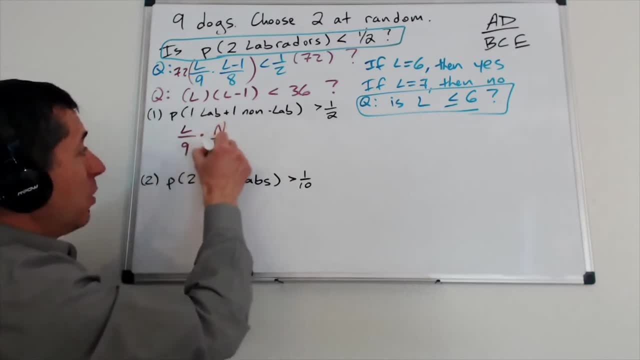 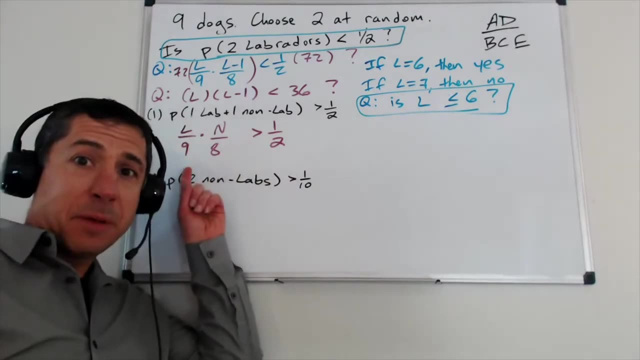 times a non-Labrador. I'm going to call that n here over eight And that's going to be greater than a half, but you got to be careful here. The way I just wrote this up, that's the probability of getting a Labrador on the first, non-Labrador on the second, And that's not quite what I'm going. 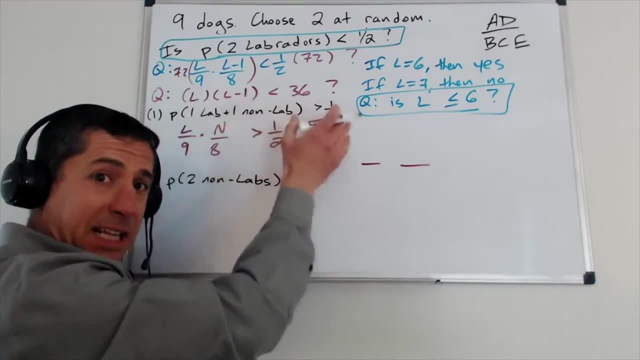 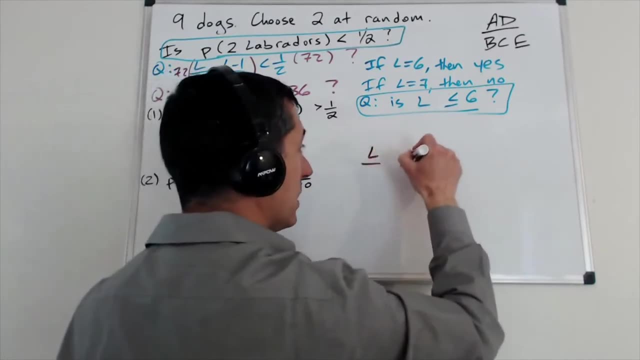 after. I don't care about the order here. I wanted the probability of getting the exact one lab, exactly one non-lab, in any order. So what that's going to be, what I just calculated here is the probability of a lab on the first, one, non-lab on the second. That's going to be. 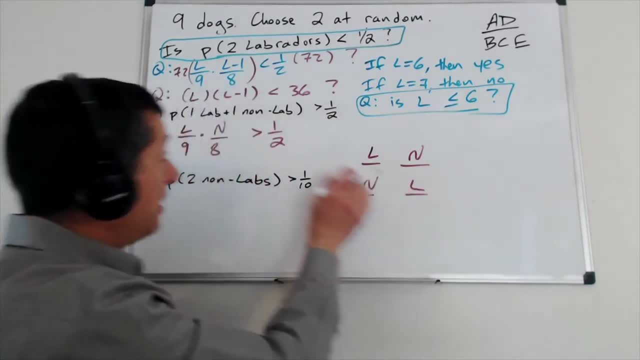 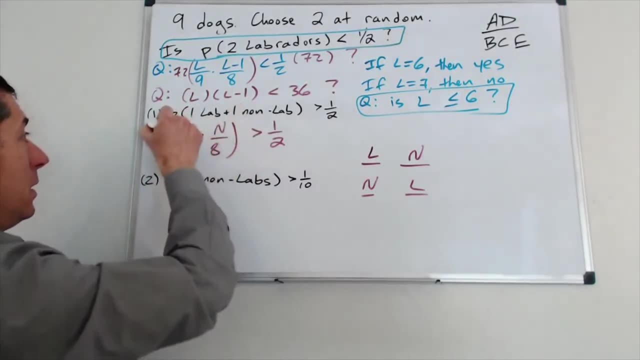 equal to the probability of getting a non-lab first and then a lab. So if I want the probability of getting exactly one of each, I've got to multiply this thing by two And I'm going to do the same kind of thing I did up here. So I'm going to cancel this out. cancel the two with the eight. 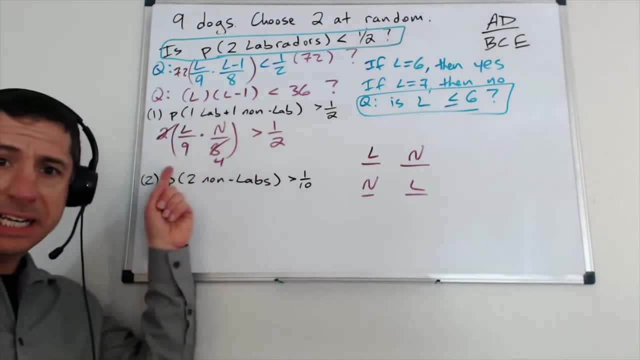 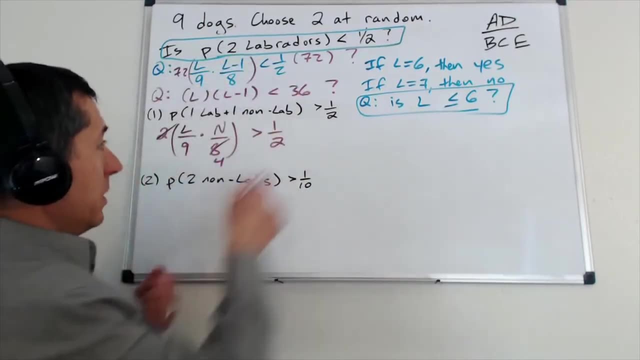 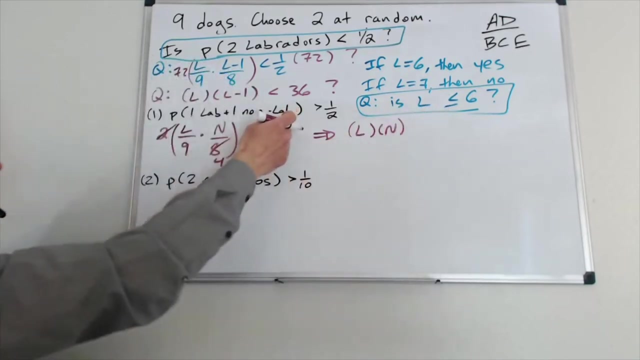 I get a four. Now I'm just going to multiply both sides by 36.. Nine times four is 36, just so that I get this simplified nicely. So this is going to give me the number of labs times the number of non-labs. 36 divided by two is going to be greater than 18.. And now I just have to think through. 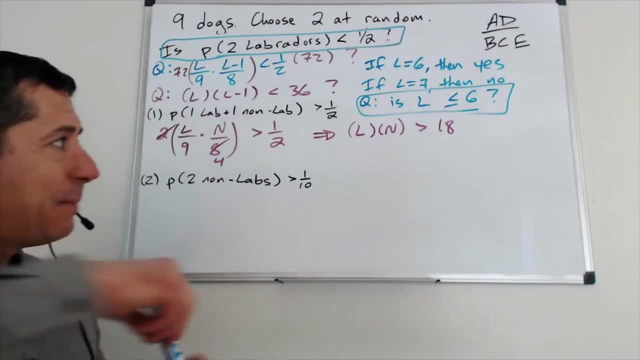 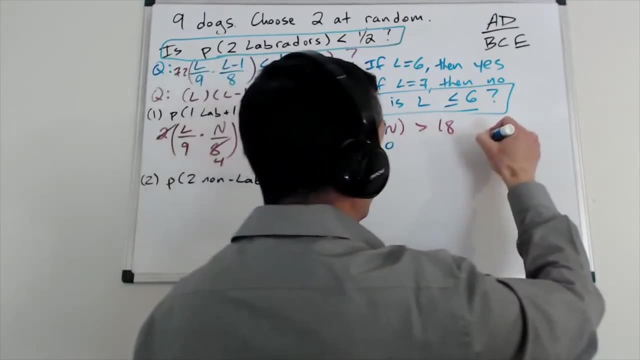 what kind of values does this give me? So if I have one lab, let's start with a big number here, I suppose, What if I have nine labs, No labs, And obviously this is not going to be true. So that can't be the case. 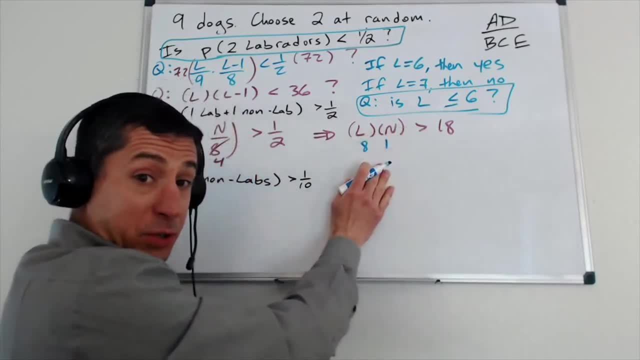 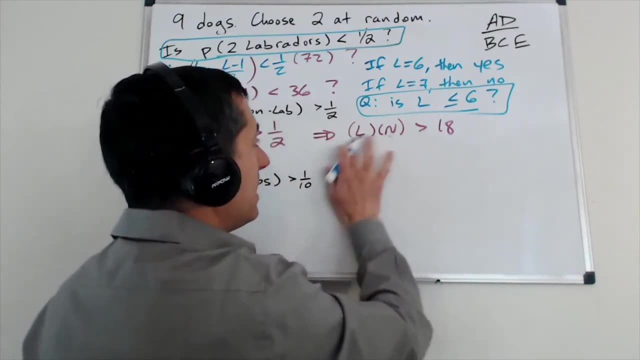 Well, what if this is an eight and a one? Still can't be true, right? There's no way I can have eight Labradors here because of the number of labs times. the number of non-labs is not greater than 18.. What about seven and two? Still not working for me, But now we're getting close. 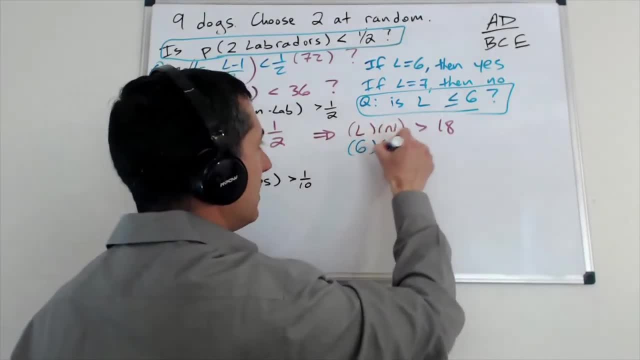 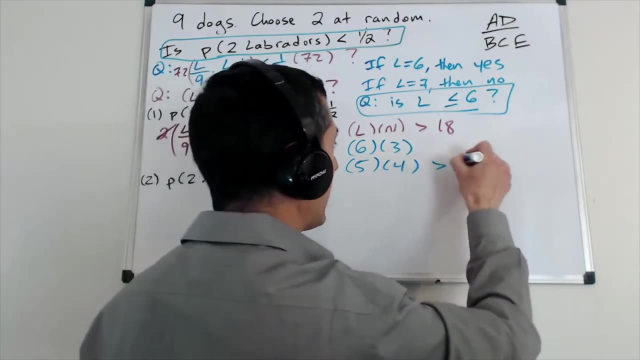 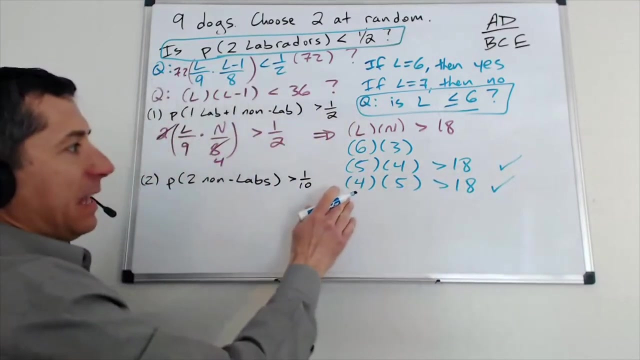 right. Could I have six labs? Not quite, Still not quite. But what about five and four? Yep, that's going to be greater than 18.. I could have four labs and five non-labs. That's going to be greater than 18.. And then we start repeating numbers, right So? 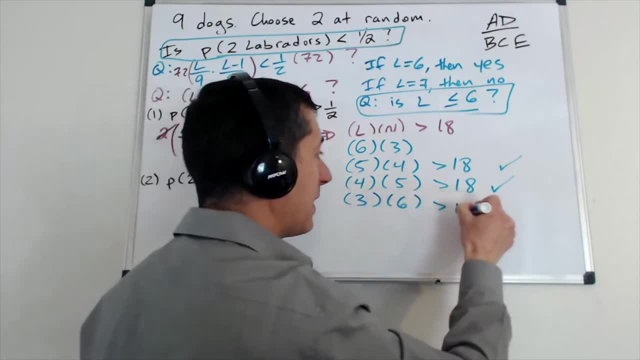 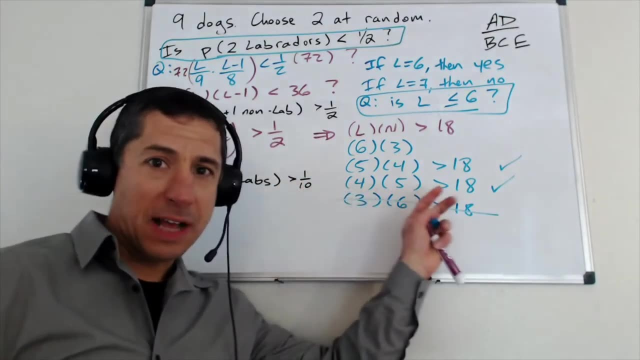 could I have three labs? Nope, that's not greater than 18.. So what does this say? This is saying I either have four or five labs. Takes a little bit of trial and error to get there, But, notice again, the numbers aren't that big. So what this tells me is that the number of labs is either four or 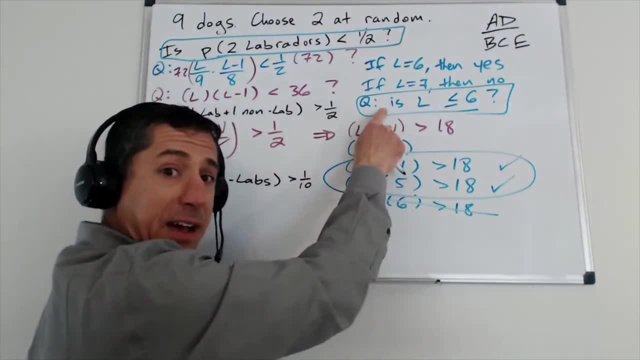 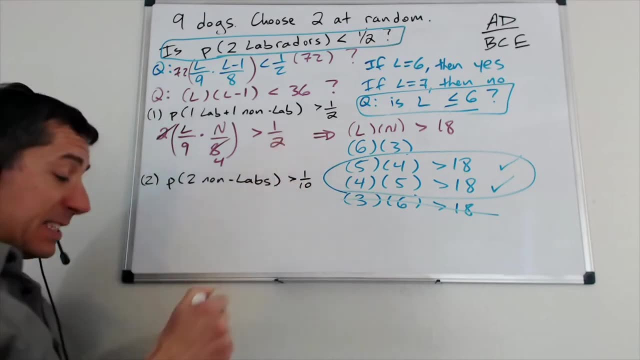 five. Now let's come back to our question. The question is: do I have six or fewer labs? Absolutely, because I have either four or five labs, based on statement one. Thanks to that statement, one is sufficient. We can cross out bce. Having fun yet, All right, I'm gonna erase. 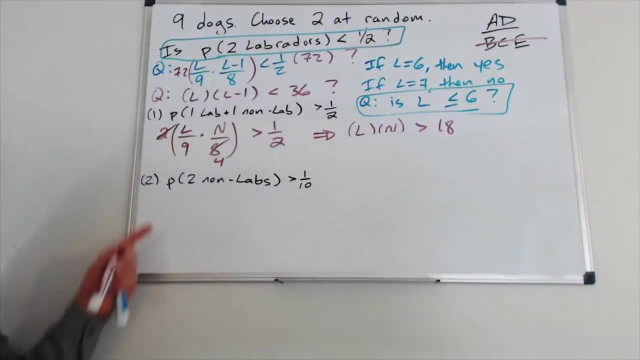 some of this in the interest of space. Probability to get two non-labs in statement two is greater than one tenth. So I can say again n over nine times n minus one. So n is the number of non-labs. First pick: the odds of getting a non-lab are n over nine. Second pick: one dog is. 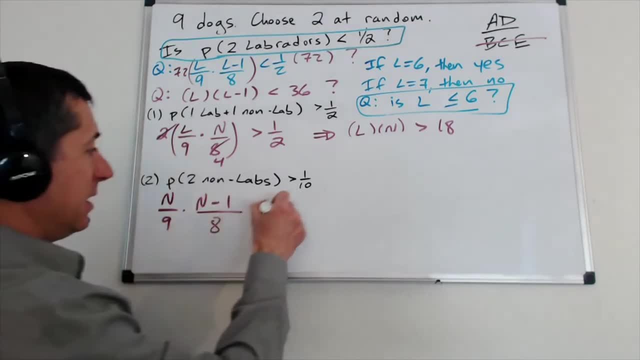 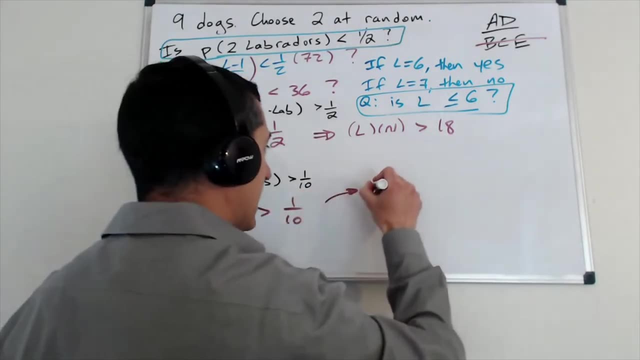 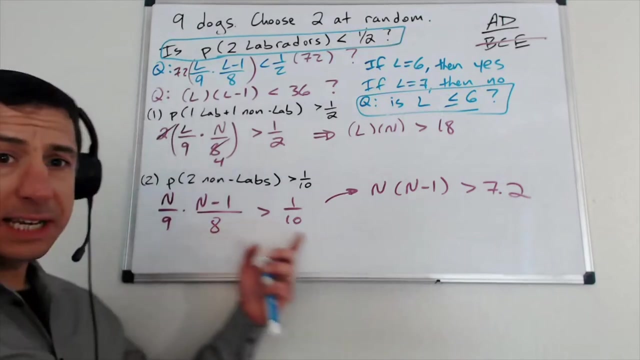 gone n minus one. divided by eight, This is greater than a tenth. Same sort of deal we did before. I'm gonna multiply both sides by 72, by eight times nine, And that's gonna give me this guy: n times n minus one is greater than 7.2.. And again we're back to that beautiful land of strategically. 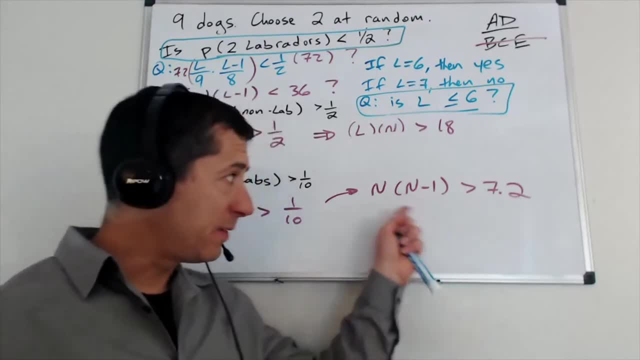 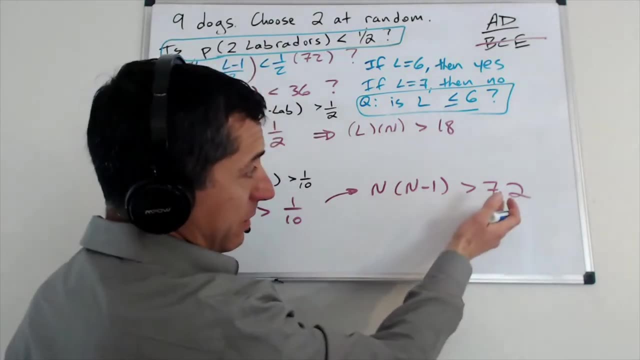 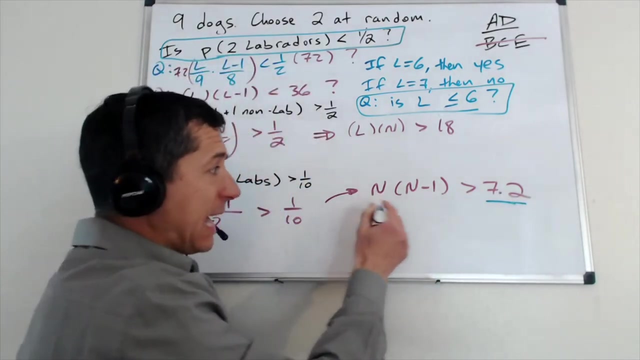 picking numbers here, not blindly, but just trying to think: here can I get to sort of a, a range of values for n? Well, is it possible to have- I'll start with small numbers and work my way up, since this is awfully small. So is it possible to have two non-labs? Nope, Three non-labs. 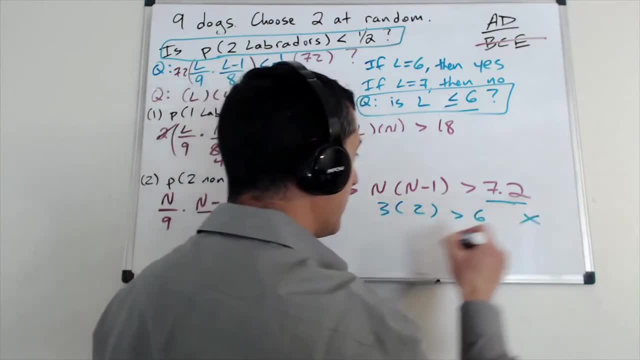 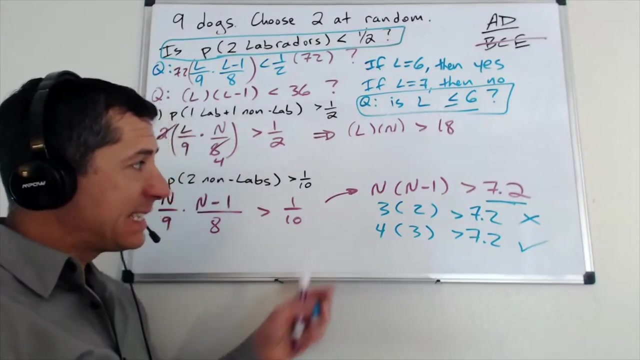 three times two, not greater than six. but what about four non-labs? Four times three is indeed greater than 7.2.. And then, as I make n bigger, I'm in business, Right? So what is this saying to me? It's saying that n is at least four. 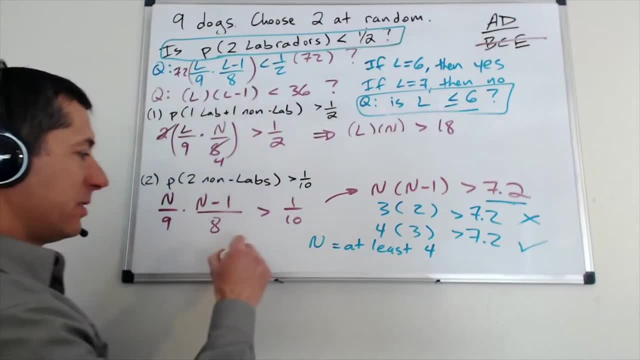 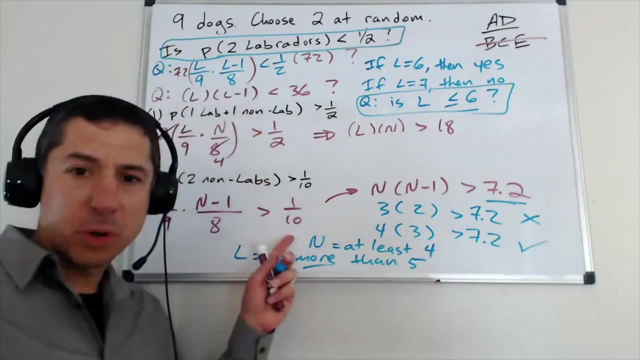 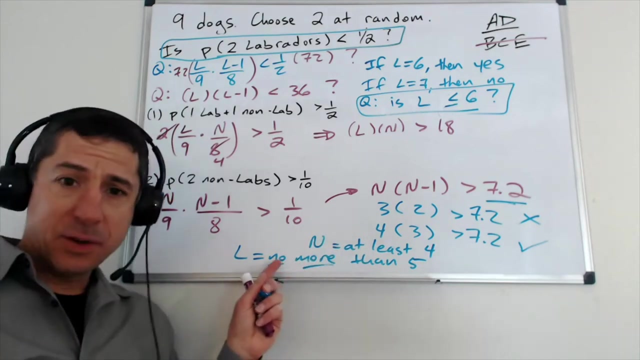 So if there's at least four non-labs here, that means that there's no more than five, So the most I could possibly have. So if the least number of non-labs I can have is four, the greatest number of labs I can have is five. So I've got five or fewer labs. 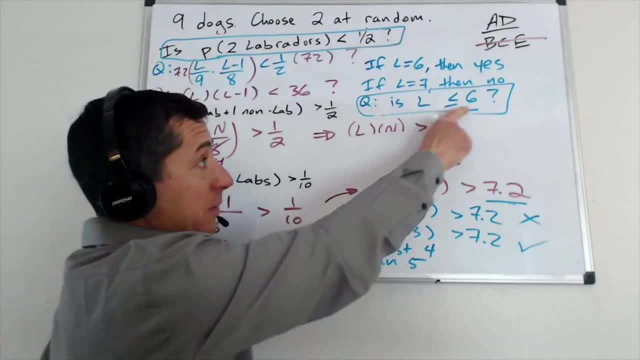 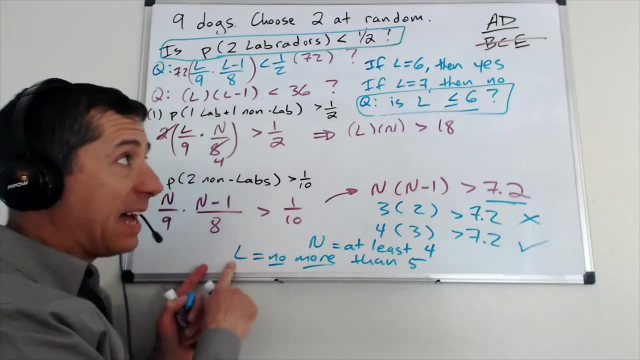 And that's perfect, Exactly what we're looking for. I want to know: is the number of labs equal to or less than six? And statement two is telling me the most I could possibly have is five. So that's efficient as well, And our answer is D, If your 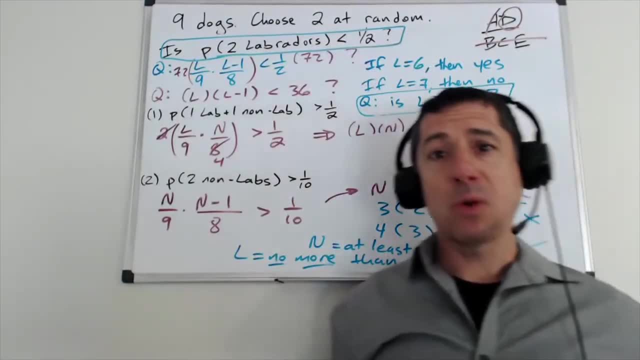 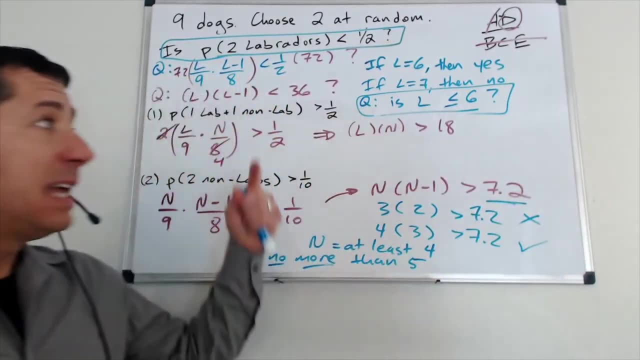 head is spinning. don't lose any sleep over it at all. The odds that you see something quite this complicated are virtually zero. But again notice, all this is a little bit of algebra, a little bit of really fundamental probability. And then we're just kind of going through and 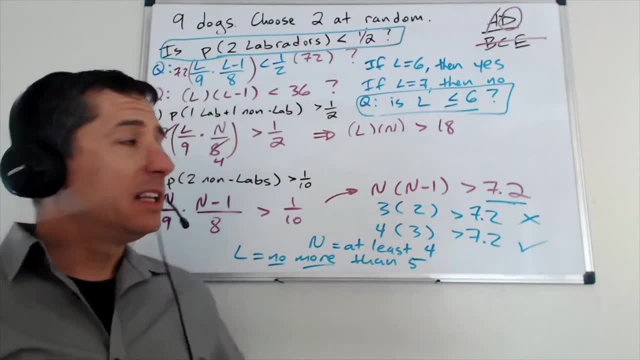 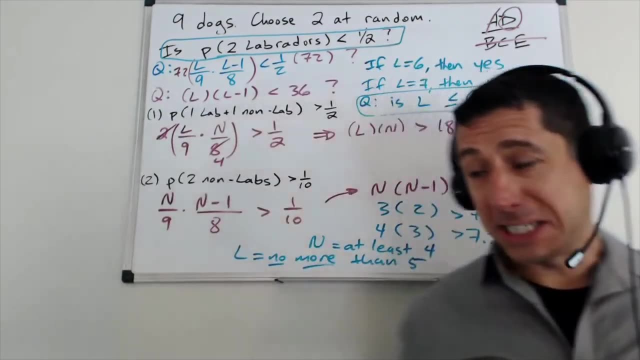 just thinking through the numbers as logically as we can, keeping information straight a little bit and error, and just thinking intuitively about the numbers, and that's all there is to it. it's just that there's so much of it that the question gets pretty bogged down. all right, last. 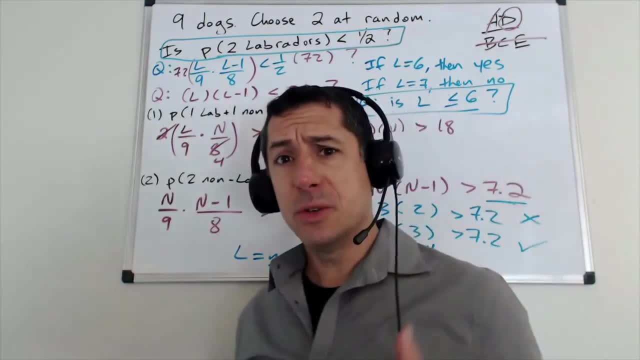 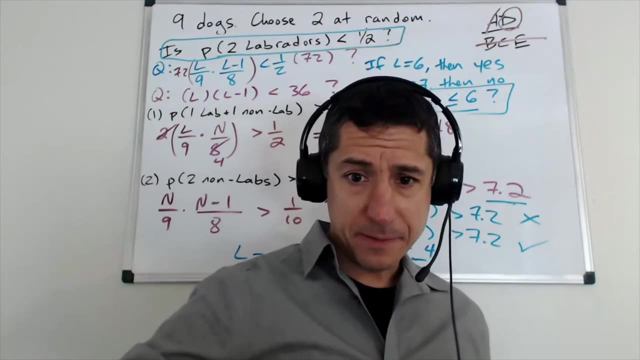 few questions here. we're going to mow it out a little bit. these last two are questions that use the language, use the term probability, but really the heart of the question is about something else. one illustrate a couple of examples of those, and then we'll wrap this up. 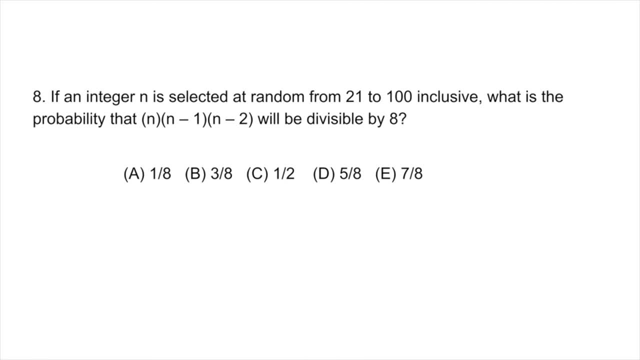 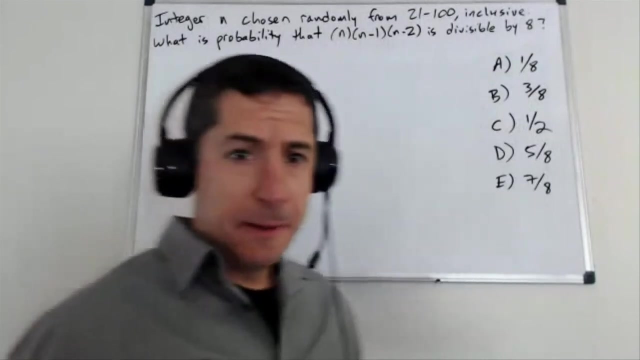 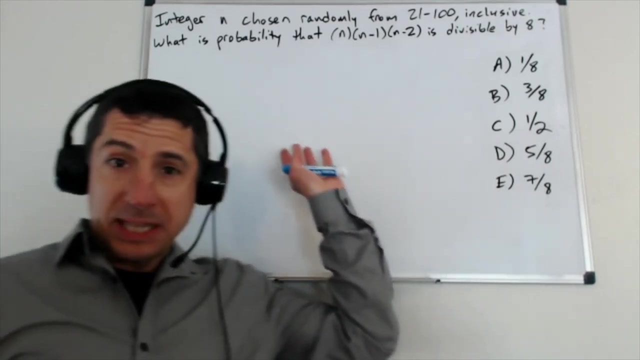 you, you, you. if you need another minute, feel free to hit that pause button, as always. okay, now we're in the not really probability section of the probability video on these last two questions questions. So not infrequently in questions that seem to be about probability, It uses the word 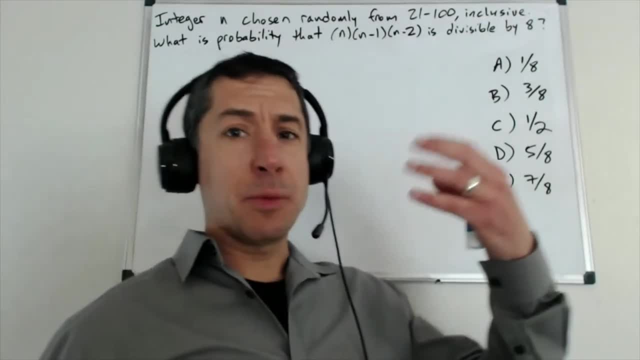 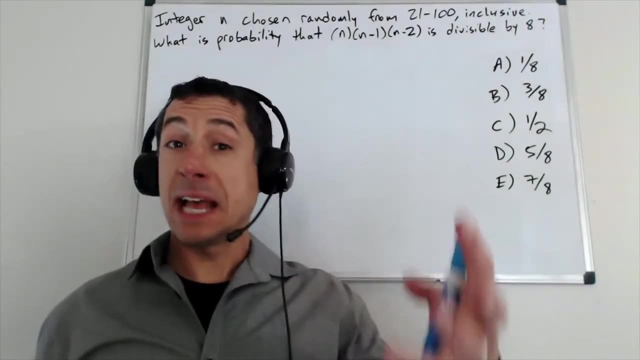 probability. Sure, it's based on that basic foundation that your probability is the number of desired outcomes over the number of total outcomes. But, fundamentally, what makes the question difficult really isn't the probability at all, It's something else. In this case, this: 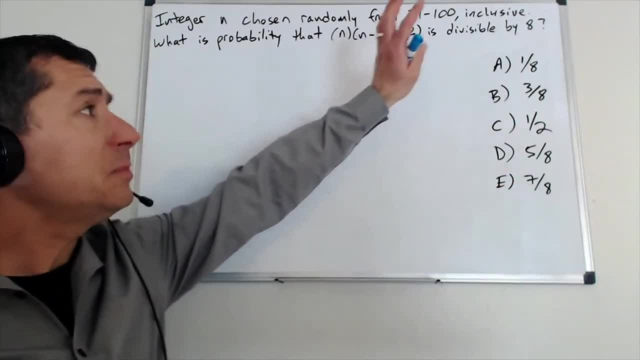 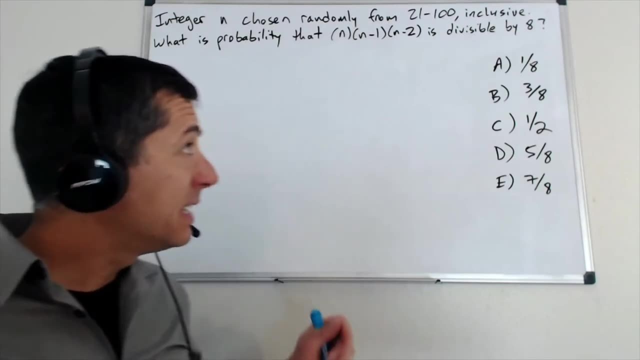 is really a number properties question disguised as probability. If you struggle a bit with number properties, please check out Harry's two videos earlier in the series: Absolutely fantastic, pretty comprehensive treatment of number properties. I'm going to assume that you have some basis in it, because that's really the heart of what we're going after here. 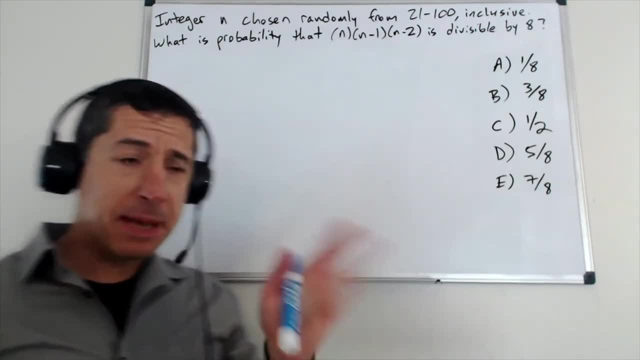 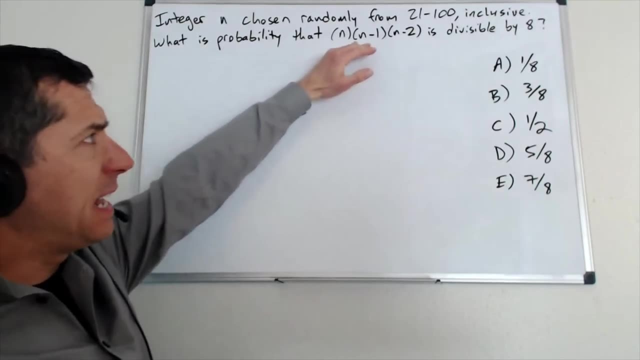 And for what it's worth. if you're not interested in number properties right now, no problem. Skip ahead to the next question. All right, Integer n is chosen randomly from the numbers 21 to 100 inclusive, And I want to know the probability that n times n minus 1. 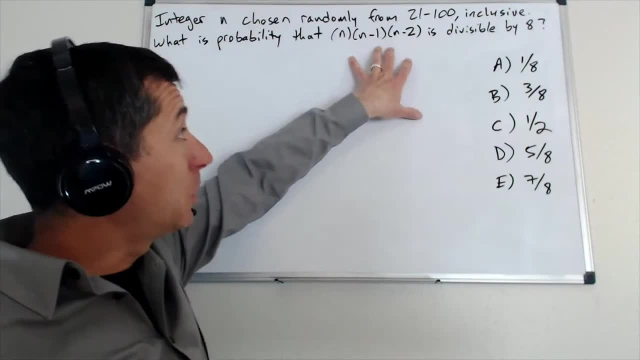 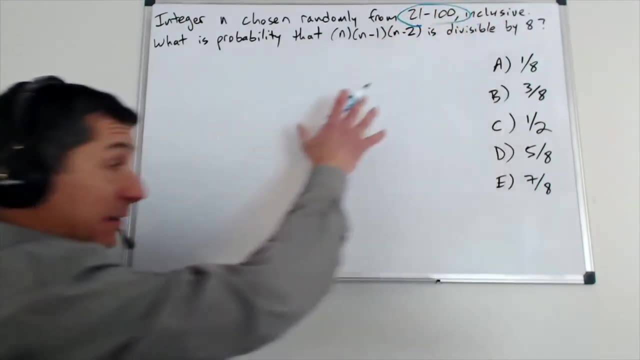 times n minus 2.. So three consecutive integers here multiplied together. I want to know the probability that that product is going to be divisible by 8.. First thought here is: well, how many integers do I have total? What's my denominator going to be? What are the total? 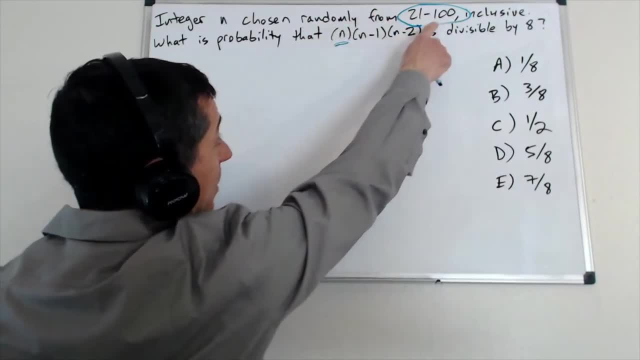 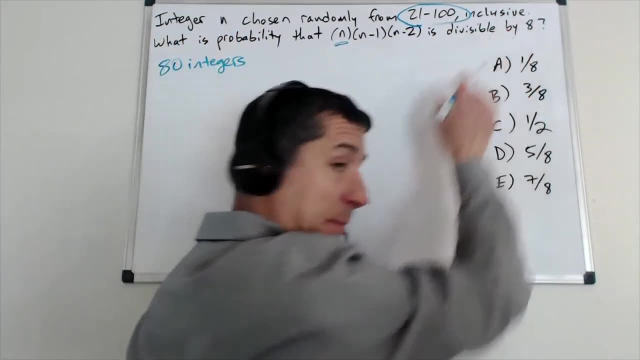 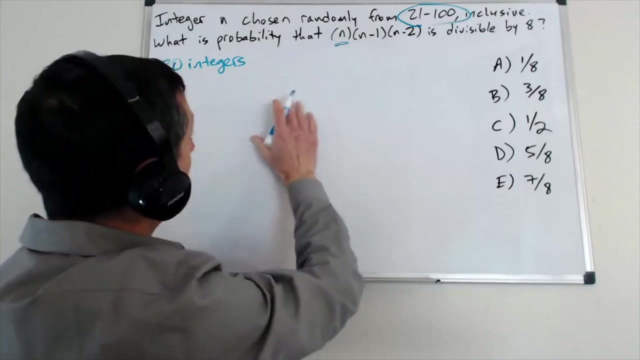 outcomes: Total different options for n. Well, this works out nicely. This is going to be 80 integers, And that makes sense. We want to know something about what fraction of those are going to be divisible by 8.. Kind of nice that the number of total integers is divisible by 8.. Good, Okay Now. 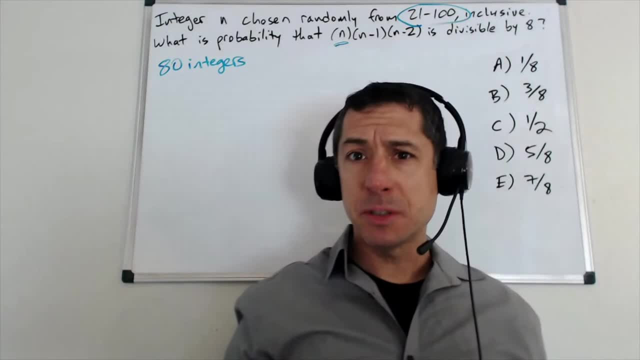 it's just about figuring out what are the different scenarios that might give me a multiple of 8 here. So my first thought is: let me think about even numbers and see if that gets me anywhere. So let's say that we have that n is even. 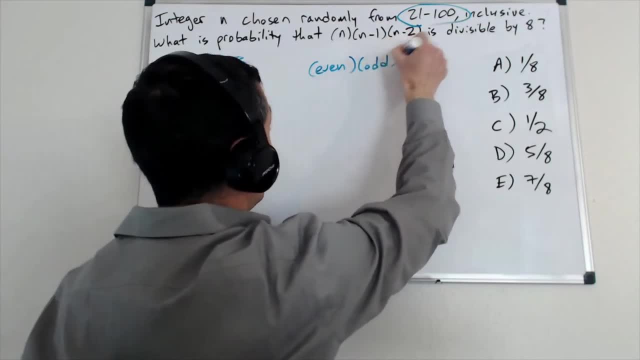 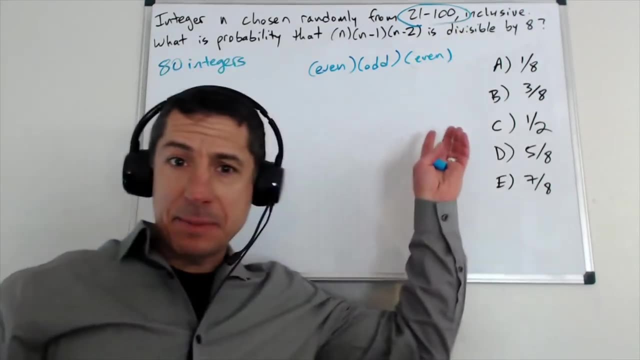 Which would make n minus 1 odd, Which would make n minus 2 even again. And the first instinct is: well, that doesn't tell me anything, because you could have two even numbers. Maybe they're multiples of 8.. Maybe they're not. Yeah, But think about what's going on with the 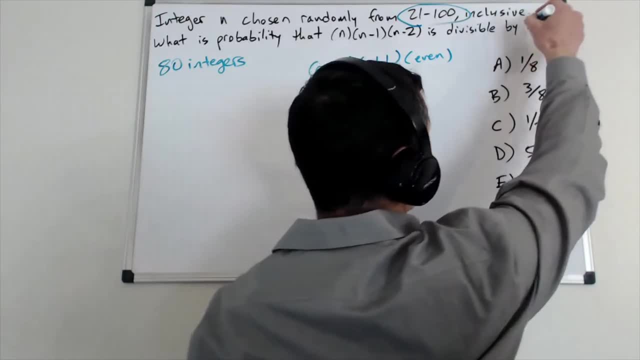 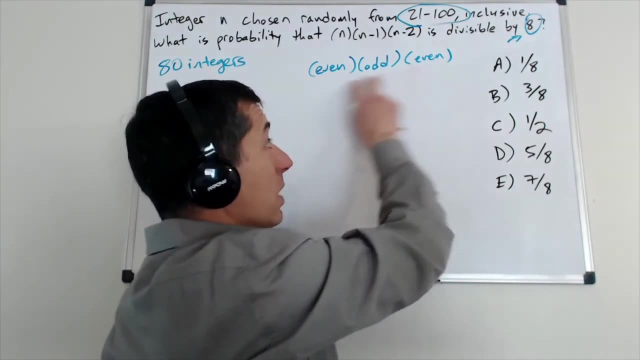 product here. So to be divisible by 8, what we need is one of these numbers to be divisible by 4, the other by 2, put another way: Somewhere in this string of numbers we need three 2s in that prime. 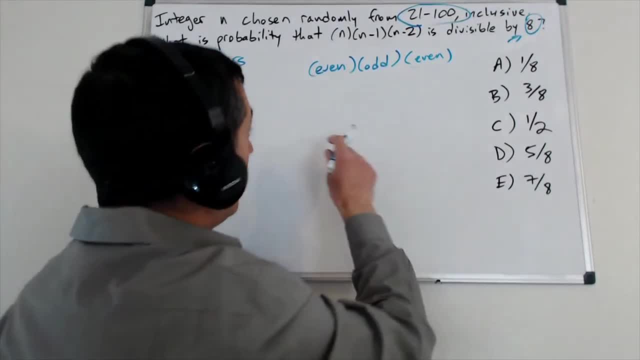 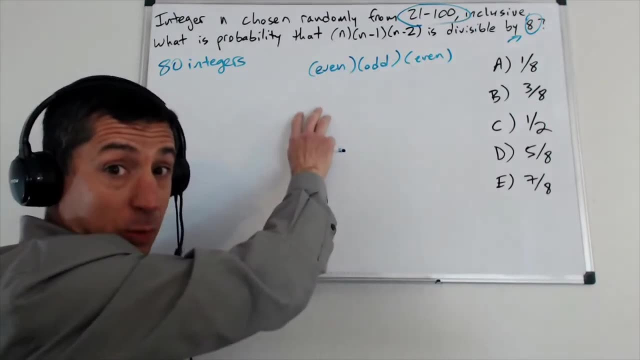 factorization, Whichever way of thinking about that works best for you. Now think about what goes on here. If n is even n, minus 2 is also even now at least. well, exactly one of those needs to also be a multiple. 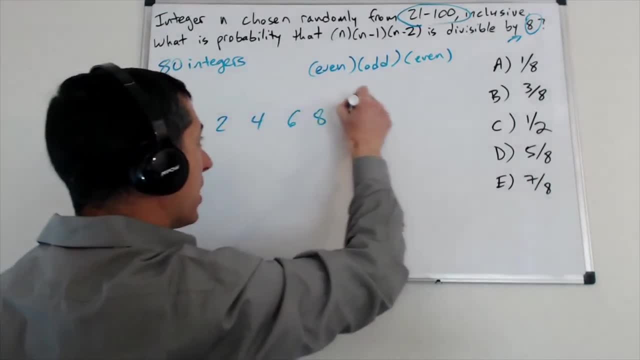 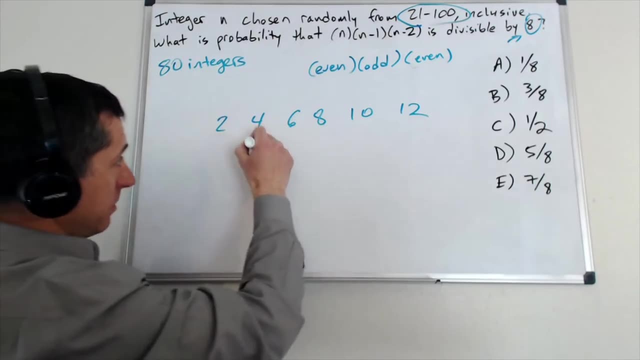 of 4.. Why is that? If it helps spot the pattern here, So just taking a random sample of consecutive even integers: not a multiple of 4, obviously a multiple of 4, not a multiple of 4,. multiple of 4,. 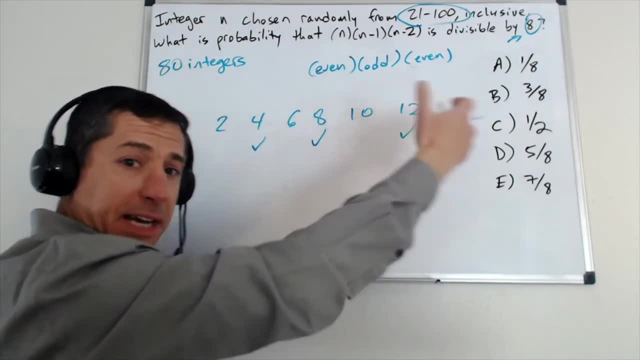 not a multiple of 4,, 12 is a multiple of 4.. And it's going to continue like that into infinity. So, okay, well, let's say that this first one is not a multiple of 4, but it's even. 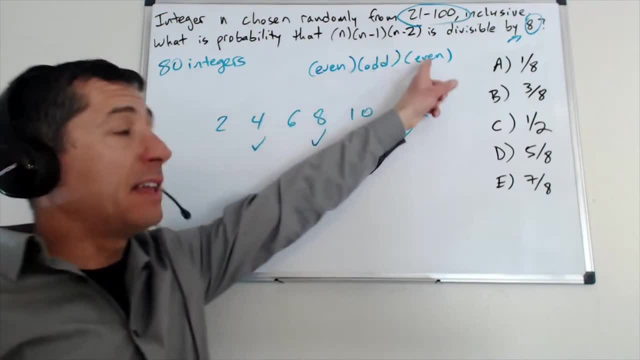 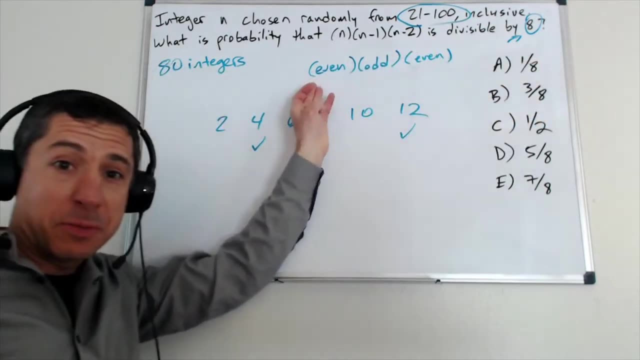 That's going to have at least one 2 in its prime factorization, Then this one would have to be a multiple of 4.. Multiple of 2 times multiple of 4, we're getting a multiple of 8.. Doesn't matter whether this one's a multiple of 4 or not. If it is a multiple of 4, great, that's just a multiple of 2.. 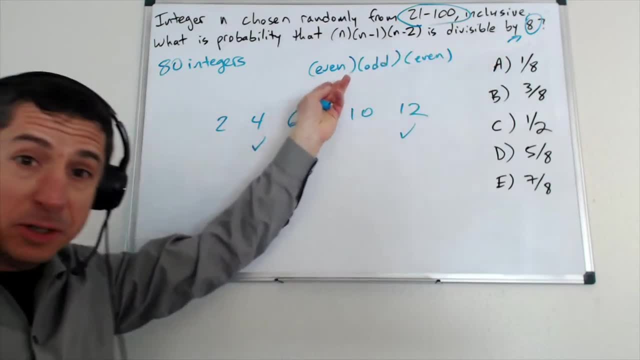 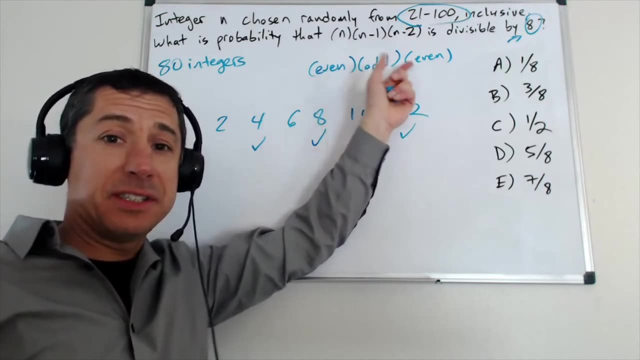 We still get something divisible by 8.. If this is not a multiple of 4, then this one would be Either way, as long as n is even, that's going to give me a number that's divisible by 8.. So what's the probability that this is the case? 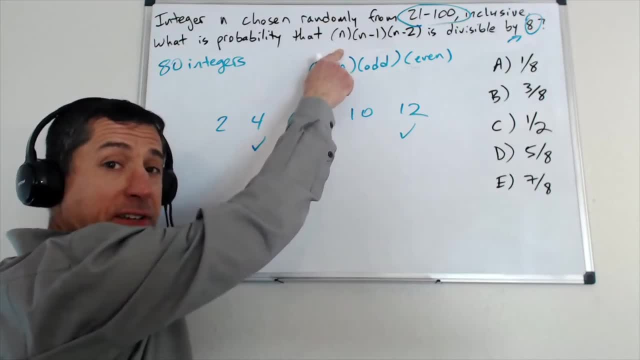 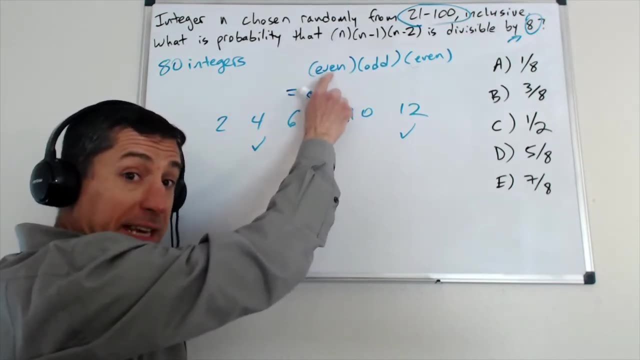 Well, 50-50 shot right. Out of any 80 consecutive integers, 40 of them are going to be even. So I know that my probability of getting an even here on that first, that n is even- the probability that n is even- is going to be 1 half. 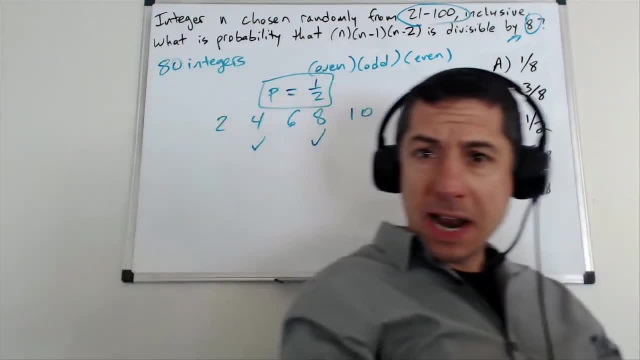 Okay, let's hang on to that and now think through. are there any other scenarios? Is there any other way for me to get these three consecutive integers? Is there any other way for me to get these three consecutive integers multiplied together to be a multiple of 8?? 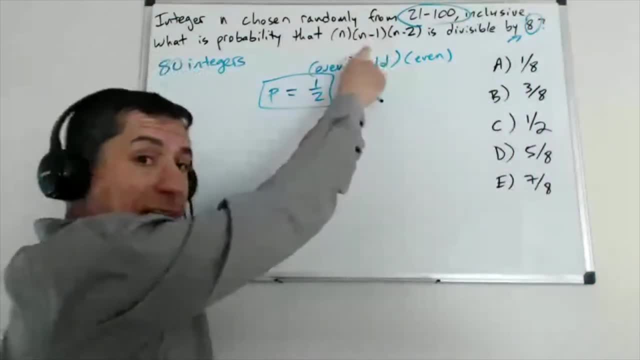 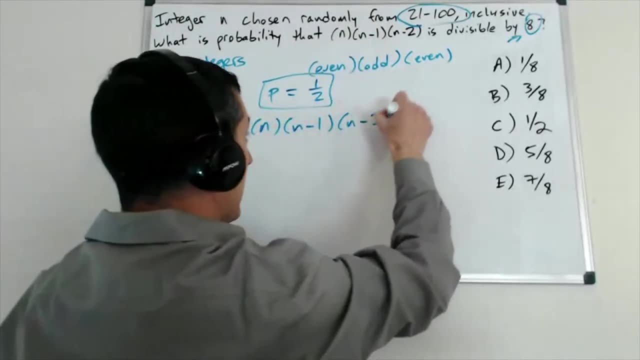 Well, what if this middle number is a multiple of 8?? What if n minus 1 is a multiple of 8?? That's the only other way to do it right. So n times n minus 1, times n minus 2.. 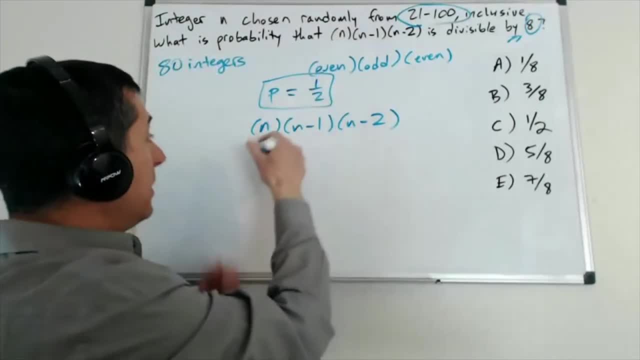 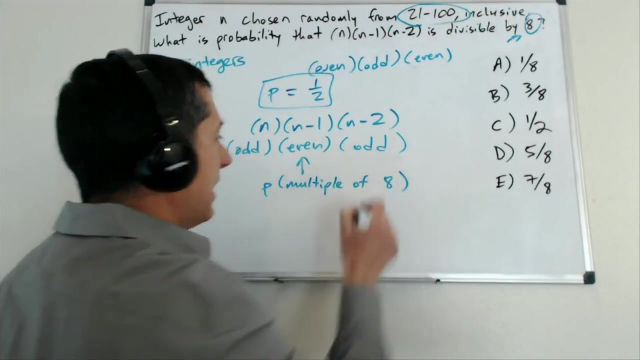 We've already accounted for all the possibilities that we start on an even. So this is odd. This is even in this scenario, And this is odd, And I want to know what's the probability that this is a multiple of 8.. And that's easy enough, right? 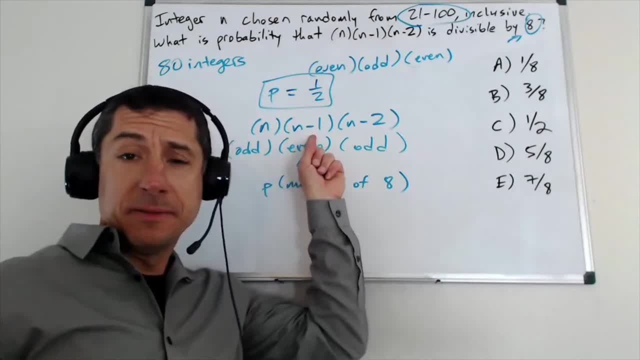 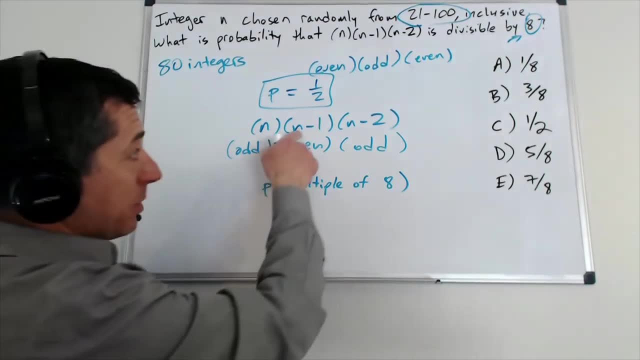 So out of any 80 possible values for n minus 1, exactly 1 eighth are going to be multiples of 8.. So I'm going to get 10 of those out of those 80. So the probability that I get a multiple of 8 here in this middle term is going to be equal to 1 eighth. 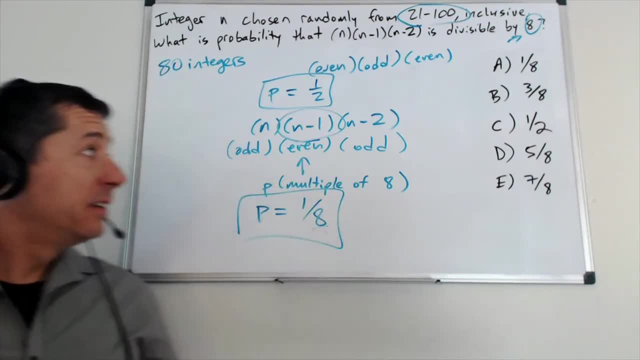 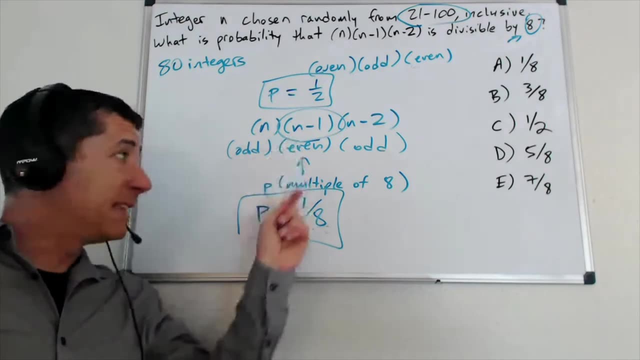 Great. Any other scenarios? Nope, I think we've covered it. So if the middle number is even, so, if n is odd, n minus 1 is going to be even Probability that this is a multiple of 8, total 1 out of 8 different values of n are going to give me a multiple of 8 here. 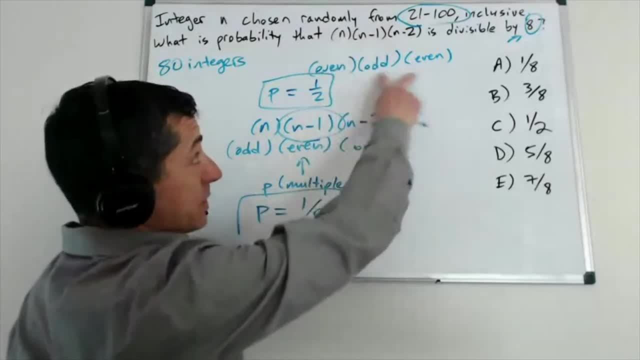 And then, 1 out of every 2 occasions, I'm going to get an even number on the first, which gives me a multiple of 8 as well. 1 half plus that 1 eighth just gives me 5 eighths. 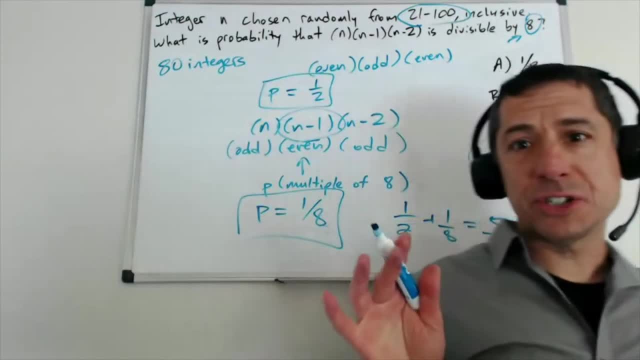 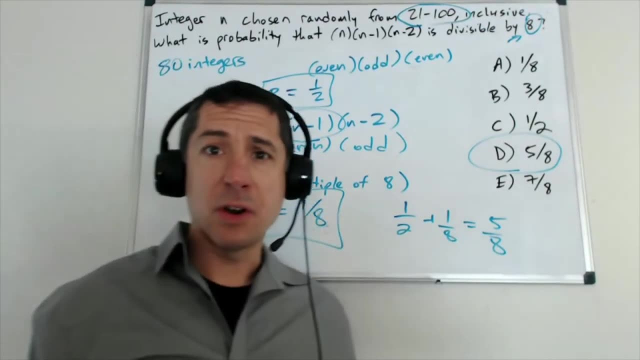 And my answer is d. And just to be clear, pretty darn tough question here. Even if you're pretty good at number properties, even if you're great at probability, you might struggle a little bit with the number of properties And logic here. no shame in that whatsoever. 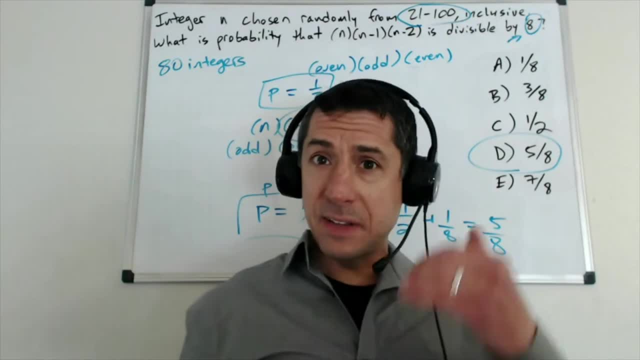 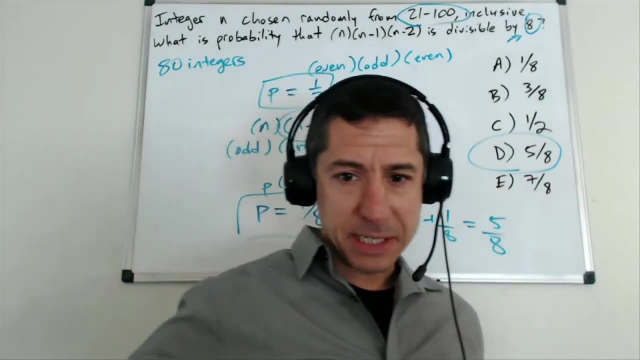 One last question, actually not super hard to end the video, but I just want to kind of illustrate how a lot of these questions end up being kind of interdisciplinary. It's a probability question in terms of the language, but really it's about combinations and permutations. 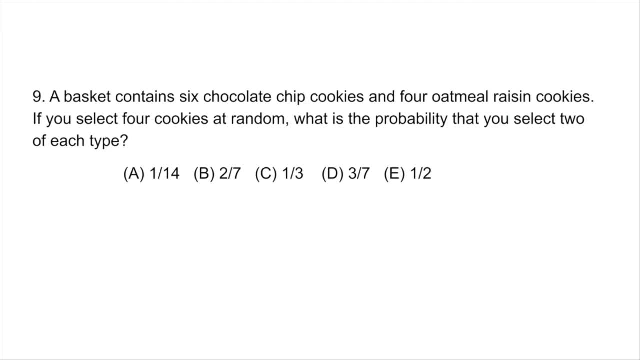 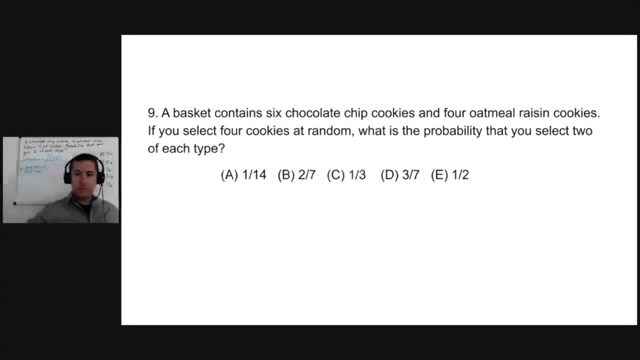 Give you guys a couple of minutes on this one. One last question. So this is going to be a very, very build up in real life 나 The idea that you have to be able to represent one you, you all right. if you need a couple more minutes, hit the pause button, as always. 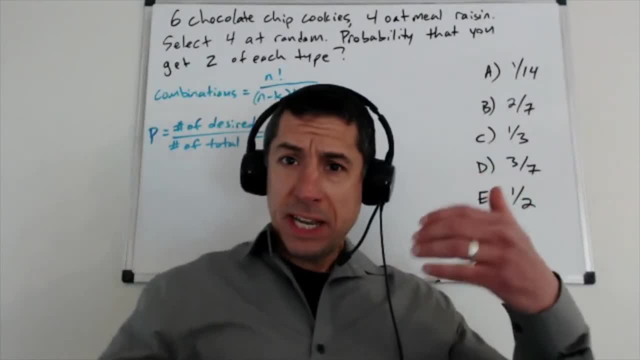 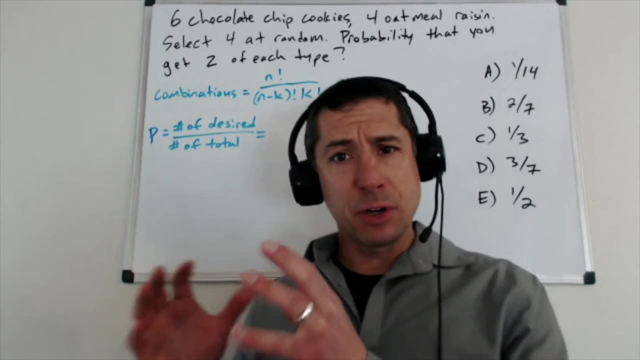 all right. last question of the video. my point here isn't that you need to know a ton about combinations and permutations. it's not we're going with it, but it really is that probability doesn't involve the probability of a combination of combinations and permutations, that many different technical wrinkles. so what have we covered in this video we talked about? 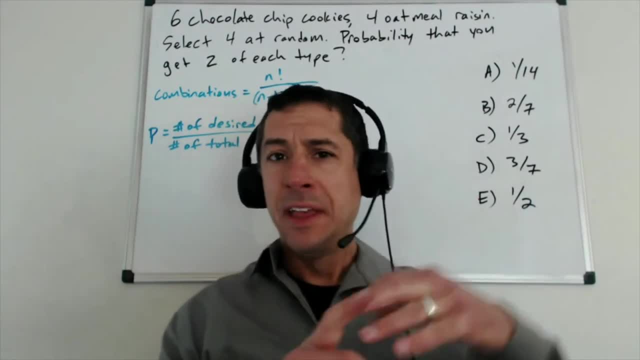 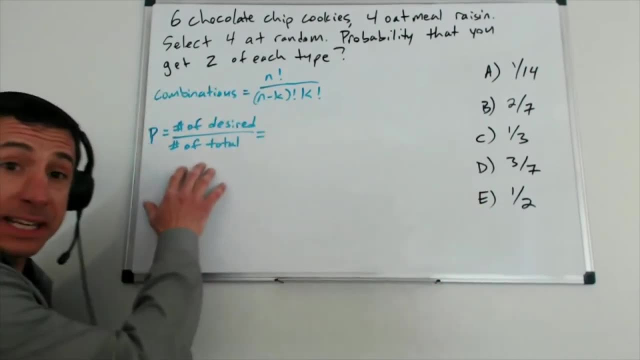 basic language, with and without replacement, talked about at least one and being able to think about that a little bit inside out- really really useful shortcut. from there it's really just a question of anchoring yourself in the basics. probability is always the number of desired outcomes over. 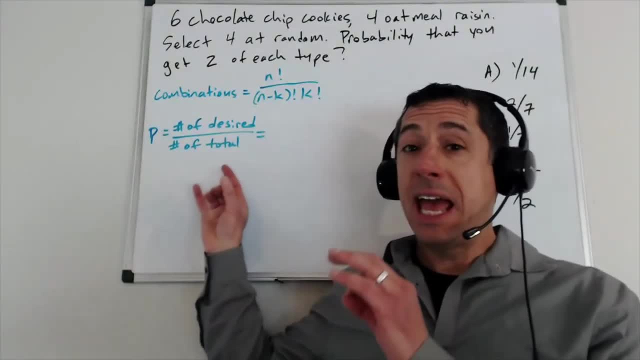 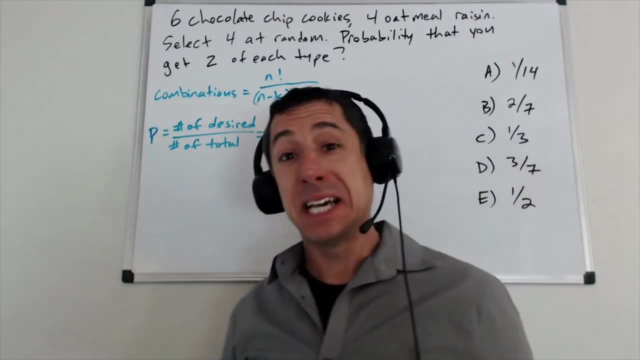 the number of total outcomes. if you can hold on to that intuition and not blindly multiply, you can answer a whole lot of really tough probability questions well, and you're also very unlikely to see a ton of them. there really isn't anything lurking over there. there's no. 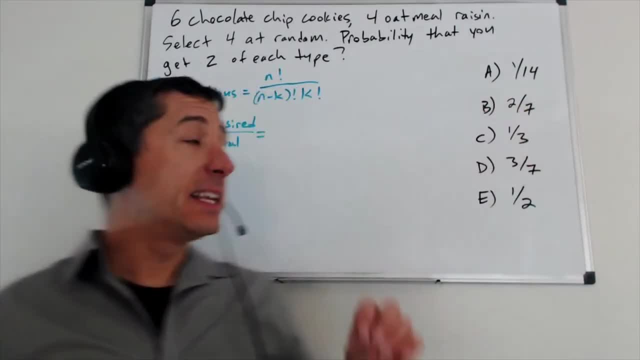 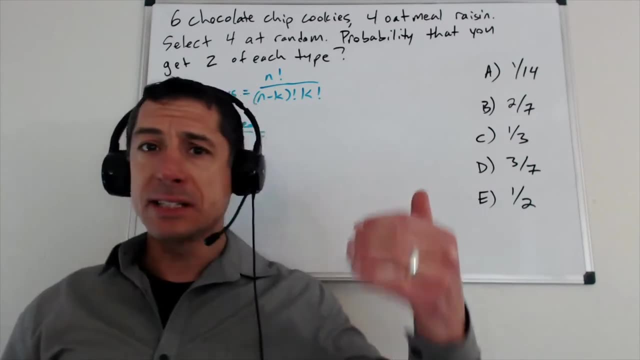 probability bogeyman where there's some magic formulas you need to learn. as long as you can anchor yourself in a little bit of basic logic, follow some intuition on these questions, there's really not a lot that you need to memorize, not a lot of variance on any formulas, nothing like that. it's really a fairly simple topic. 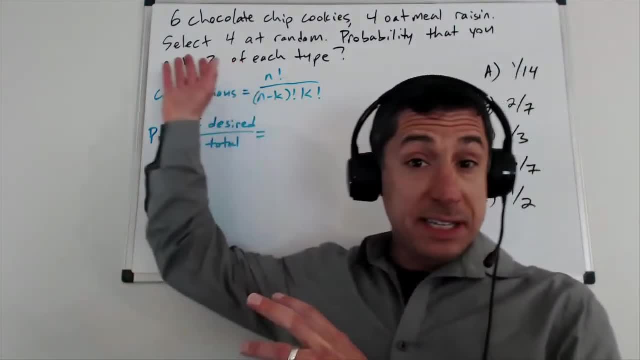 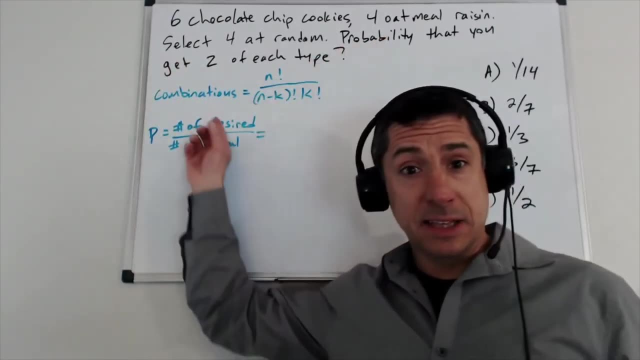 induces a ton of anxiety and maybe part of it is that a lot of probability questions again aren't really probability at all. so uses the word probability, you bet. so we're going to have to calculate the number of desired outcomes and the number of total outcomes and divide one by the. 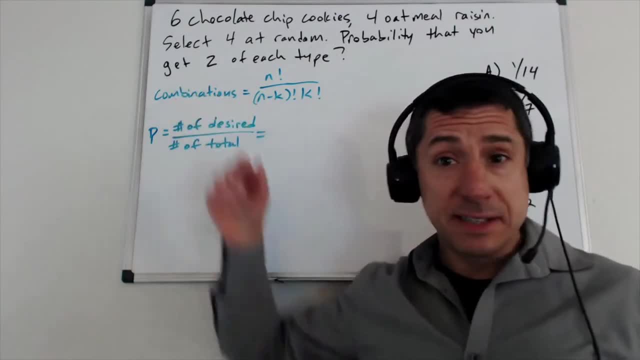 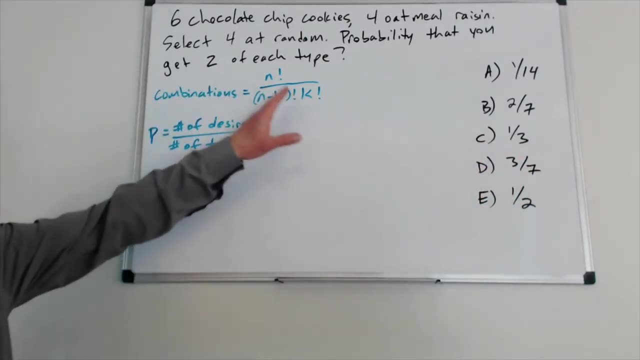 other, but really this is about combinations and permutations, combinations and permutations and combinations in this case. so if you have not seen this before, we have another full video on combinations and permutations coming up next, but here's your basic formula for it. if you don't know that i'm going to keep steaming ahead, as if you do, you can watch that other video if you need to go. 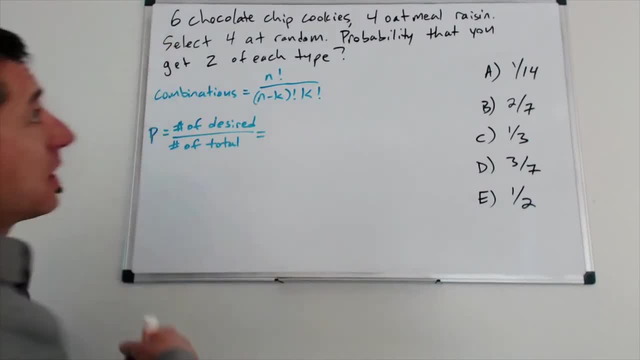 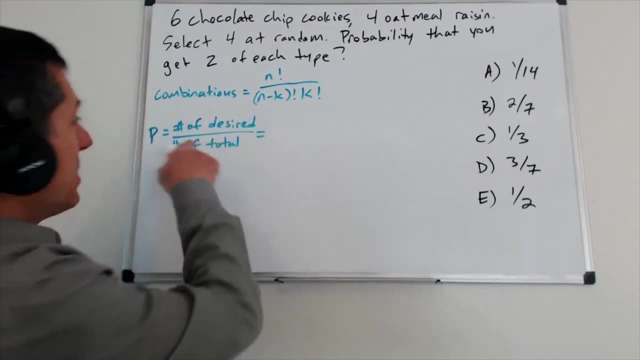 back through the basics with us. so here, what's going on? i got six chocolate chip cookies, four little raisin cookies. i'm going to select four at random. i want to know the probability that i get two of each type, so i'm going to start here. what exactly is it that we desire? what's the desired? 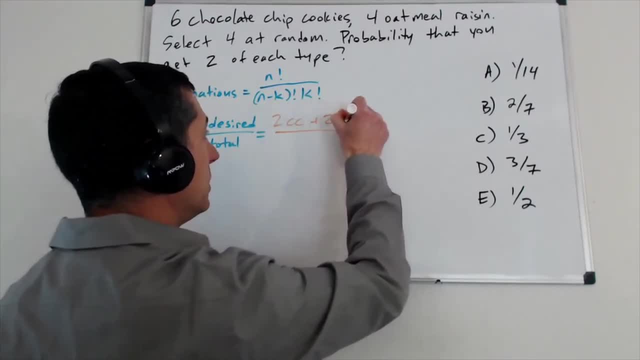 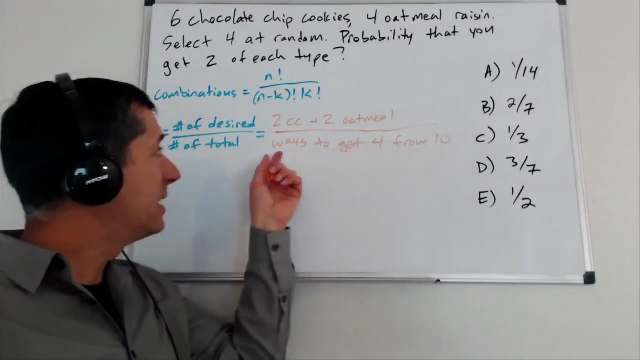 outcome So two chocolate chip cookies and two oatmeal raisin cookies, And what's the total outcomes? That's ways to get four cookies from 10, right? So if I randomly select 10 cookies, how many ways can I get four of them? And now, how many ways can I get two chocolate chip and? 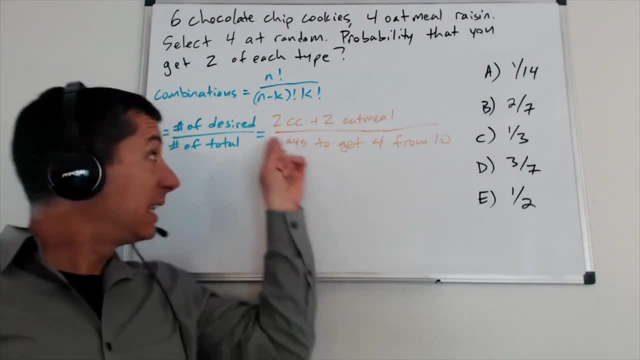 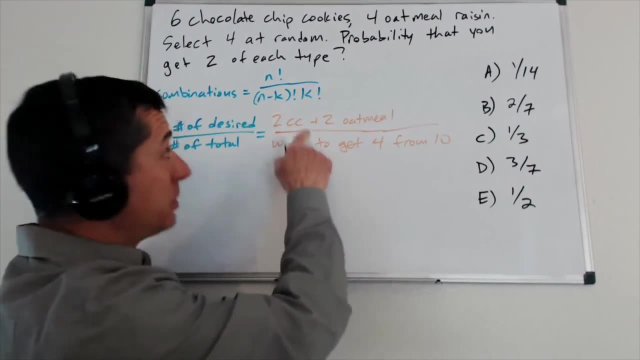 oatmeal cookies. Okay, really, this is just recycling this formula three times and that's all there is to it. So I'm going to start with the ways to get four from 10.. So 10 cookies? I'm going to choose four. punch it into our handy little formula here: 10 factorial over six. 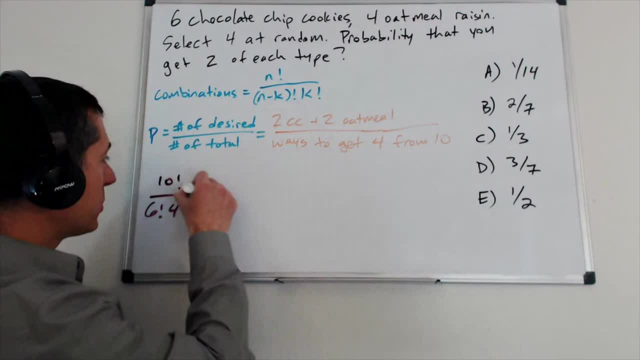 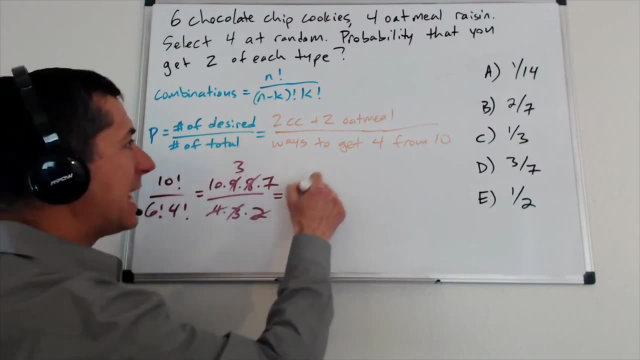 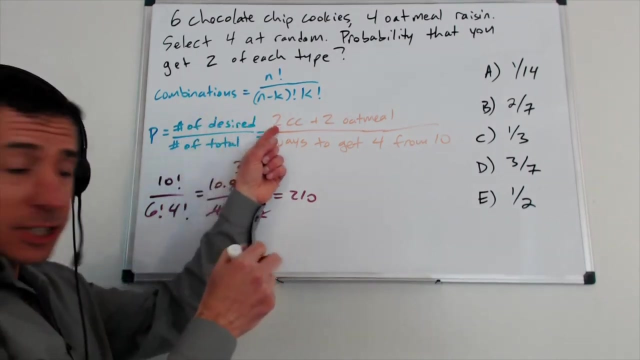 factorial, four factorial. So 10 times nine times eight times seven, four times three times two. eight cancels the three cancels and I get 210.. There's my denominator up there. How many ways can I get two chocolate chip cookies? 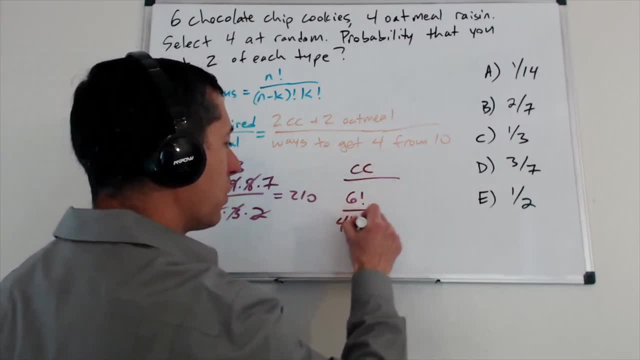 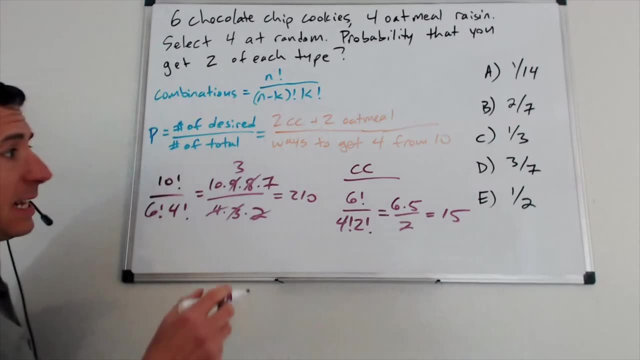 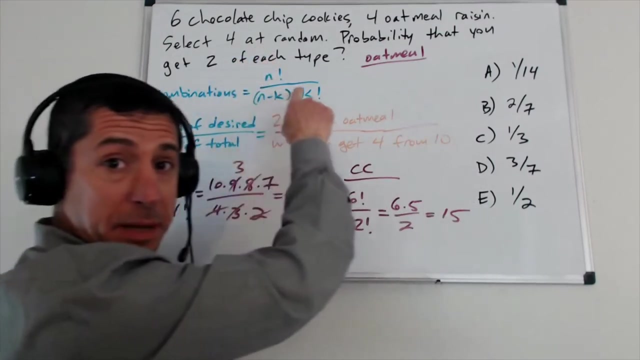 So that's just going to be six factorial over four factorial, two factorial. So six times five over two, that's 15.. And I'm running out of space, my oatmeal raisin cookies. I've got four to choose from. I'm going to choose exactly two. 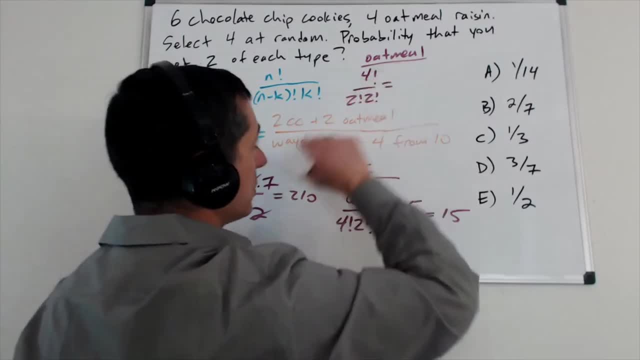 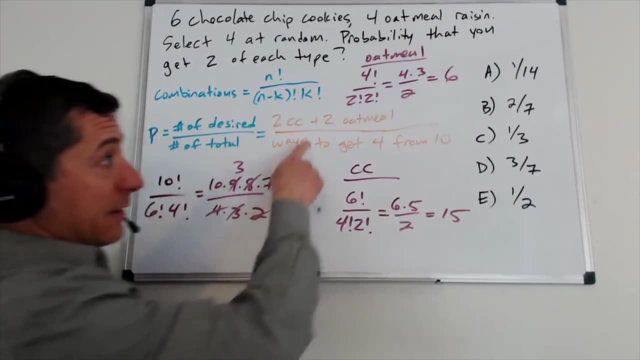 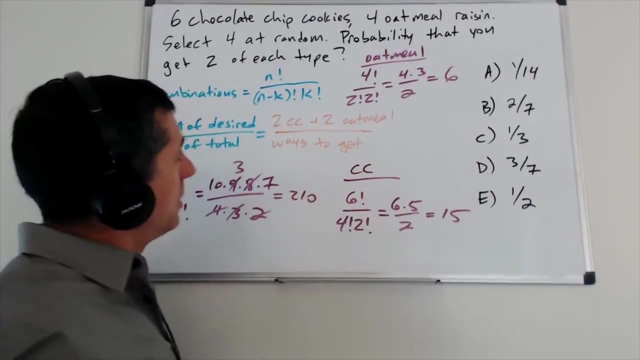 punch in the formula once again: four factorial over two factorial. two factorial. That should give me four times three over two or six. Okay, all I've got to do is just go through this, punch these in and I'm in business. So I'm going to raise this guy now. 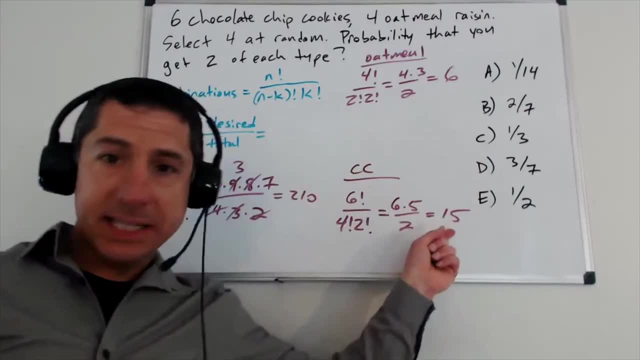 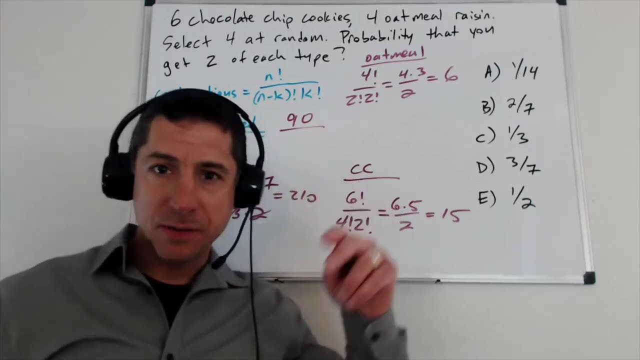 So how many desired outcomes I've got six ways to get two oatmeal cookies, 15 ways to get two chocolate chip cookies. multiply those two together So I get 90 total combinations of two different chocolate chip and two different oatmeal raisin cookies. How many total ways can? 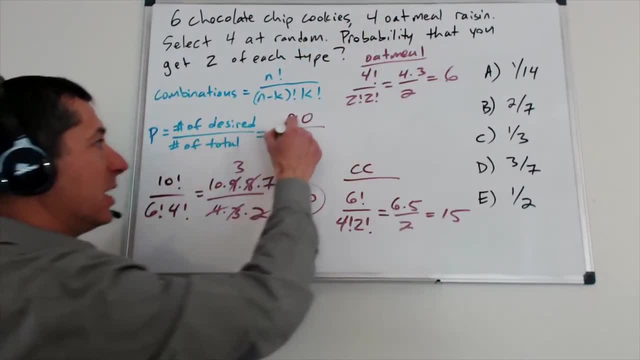 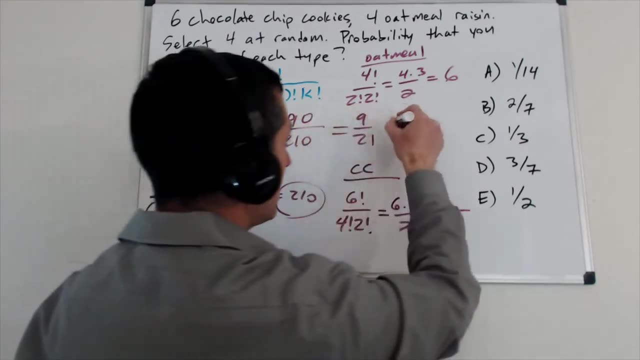 I select four from that group of 10?. That's just the 210 here, And I can simplify a little bit. I get nine over two, 21 by dividing top and bottom by 10, divide top and bottom by three and I get three sevenths. 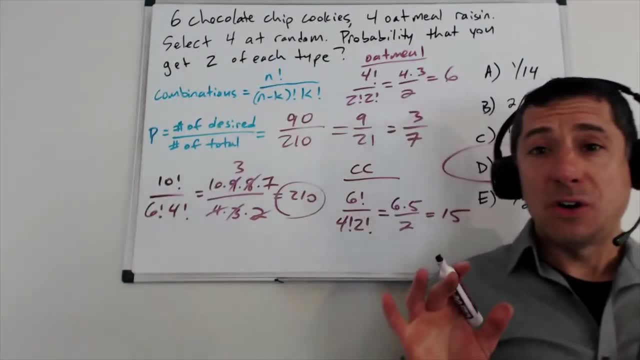 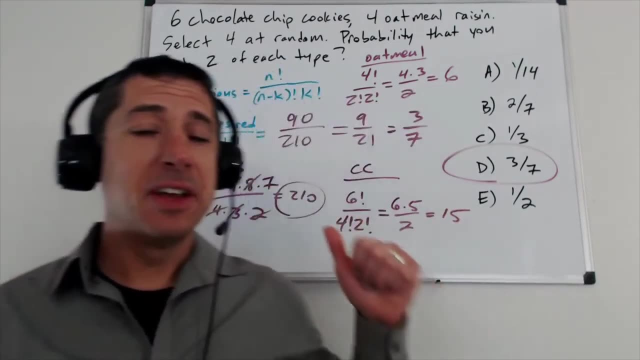 And D is my answer, and that's all there is to it. All right, Biggest takeaway of this video? please don't let probability keep you up at night. Number one can't say this enough: not the most important question type, not even close. One out of every 50 questions. 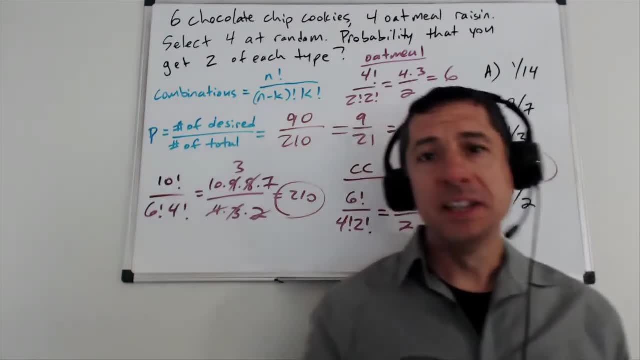 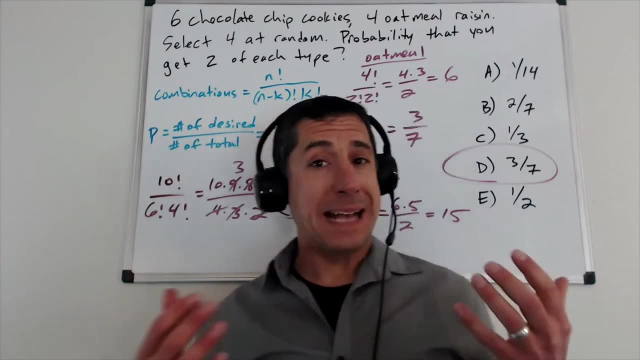 may be on your geometry quant section. it's going to be probability. From that perspective, don't lose too much sleep over it. And also, even if you are shooting for super, super, super high score or you just want to master it because it keeps you up at night and 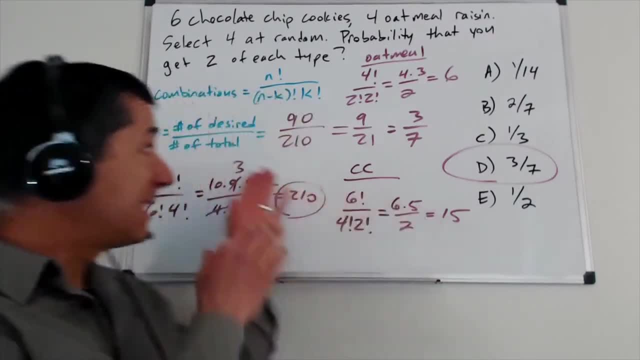 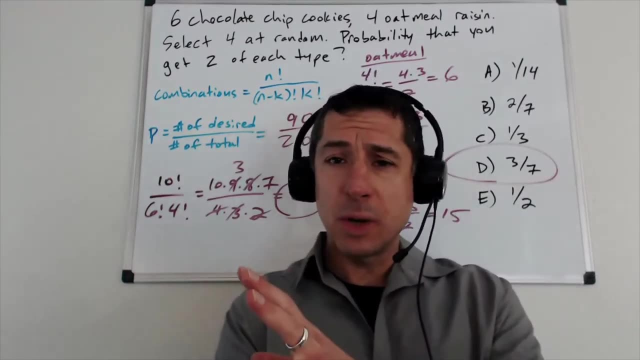 it does bug you. there's not a lot to master here: Basic set of intuition, basic definition of probability, couple of fundamental little pieces of technicalities, language to watch out for. that's really all there is to it. There's nothing else lurking there. You don't want to sit up and 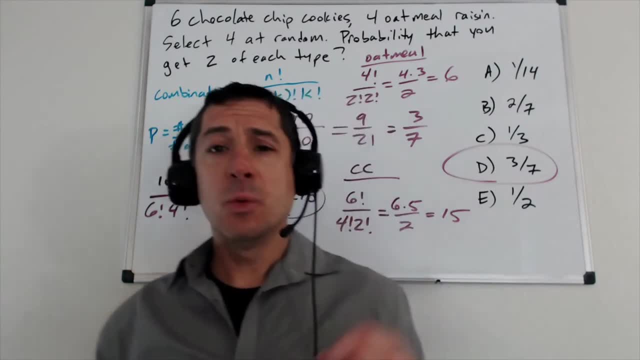 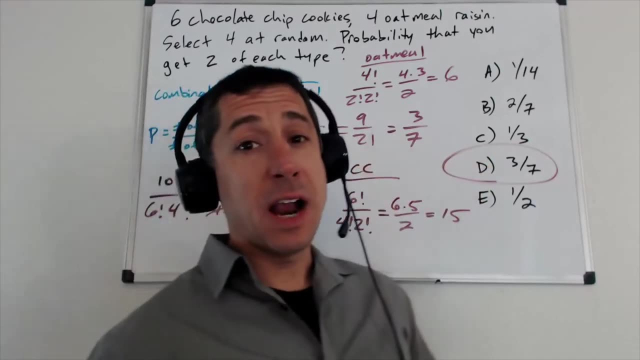 study probability for hours on end. There are far more important things on the test. When you do encounter it, just anchor yourself in the basic intuition, even if the question is pretty funky and you're going to be in perfectly good shape, All right. that wraps it up. Thank you so much for watching and we'll see you next time.